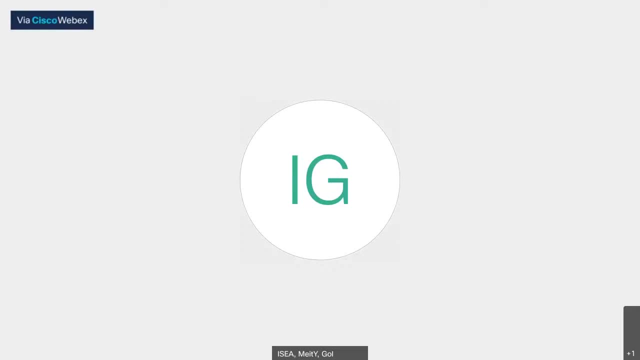 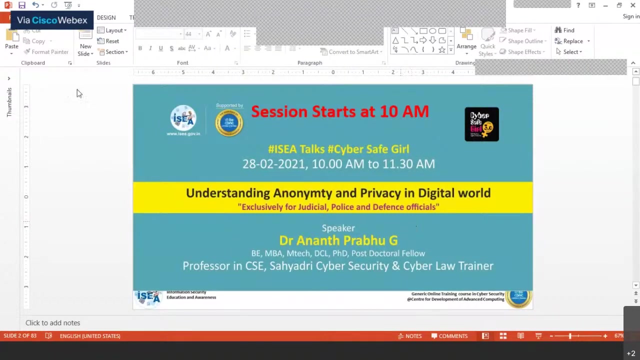 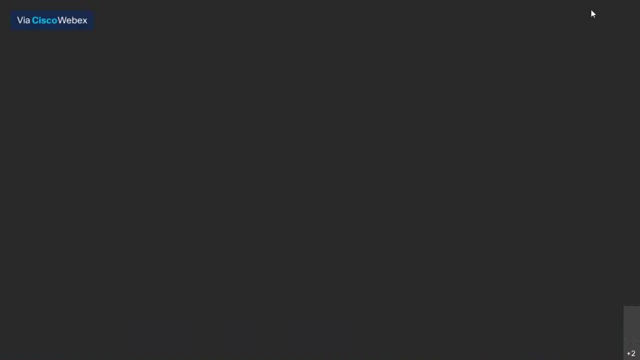 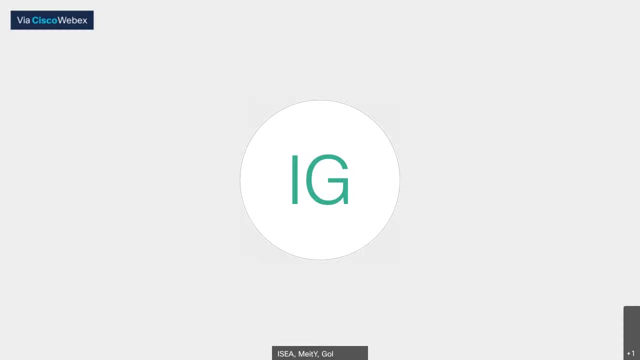 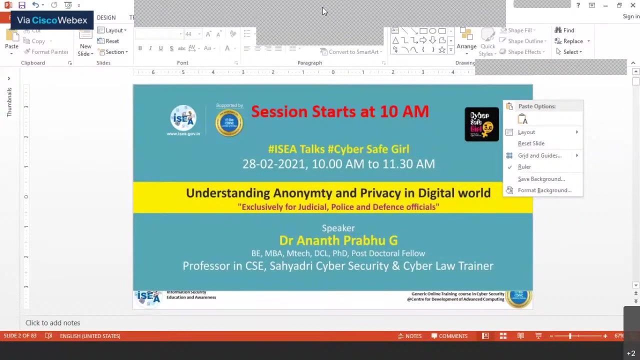 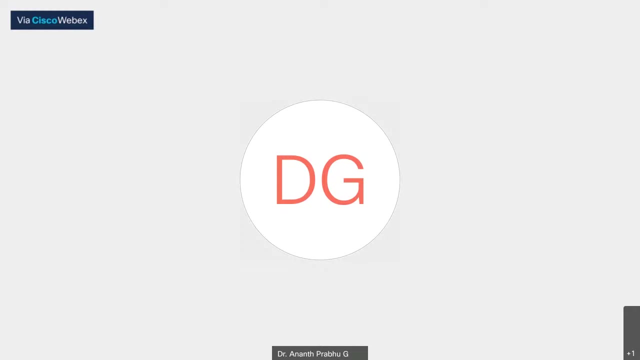 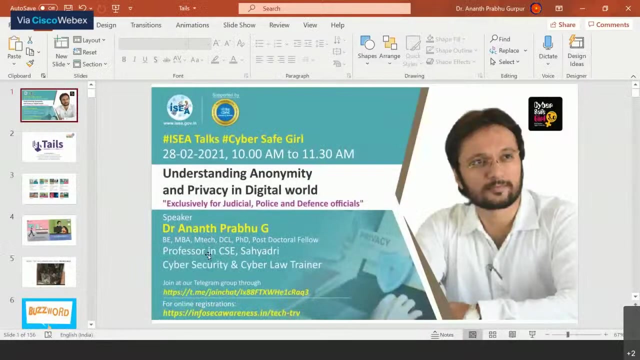 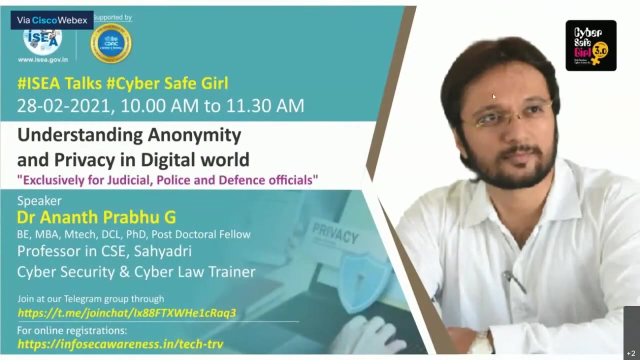 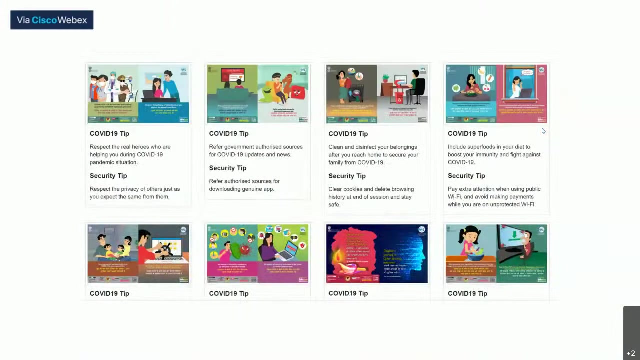 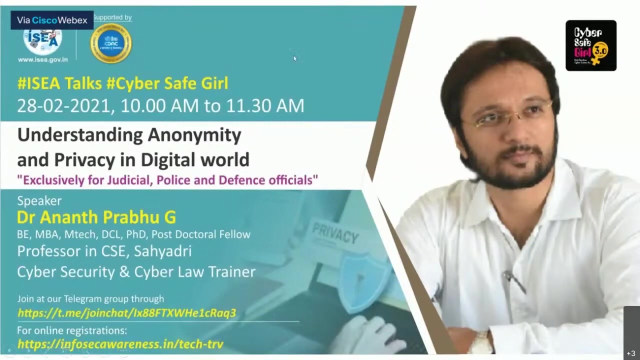 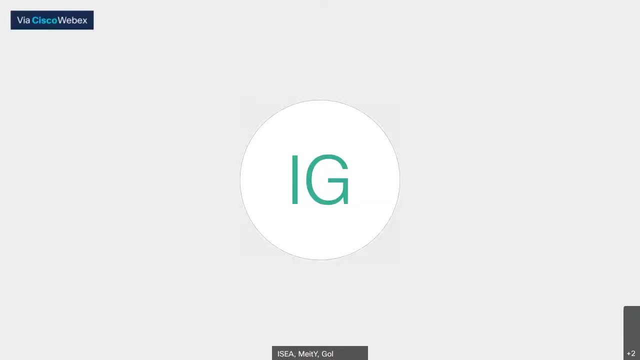 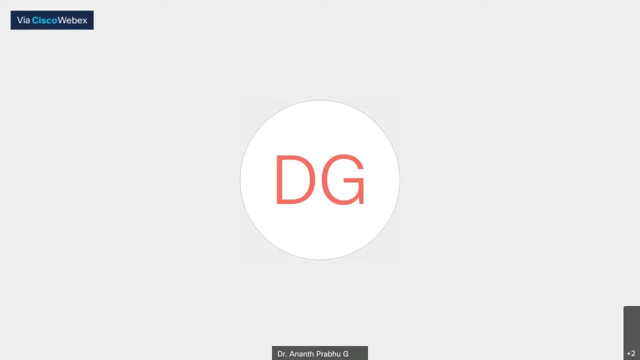 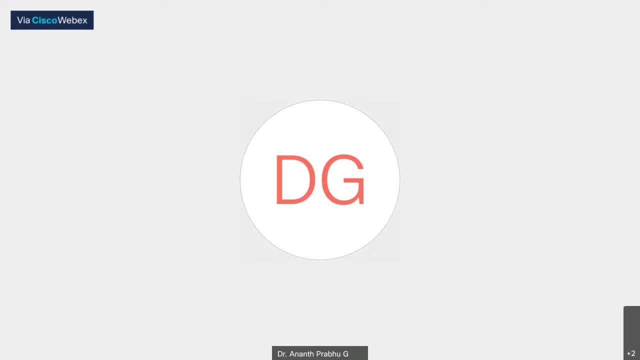 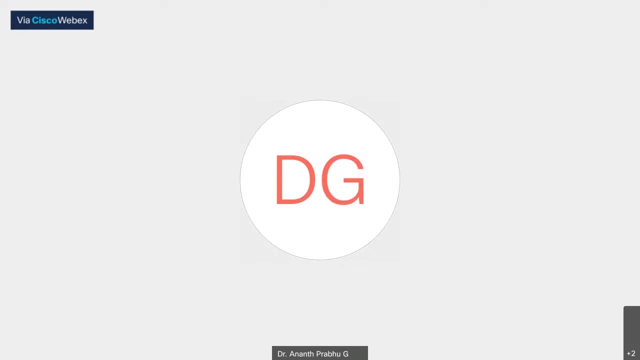 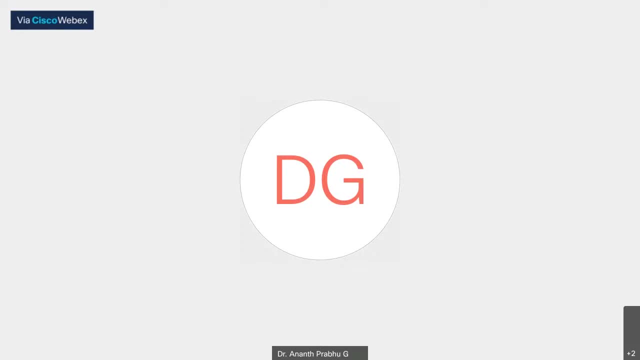 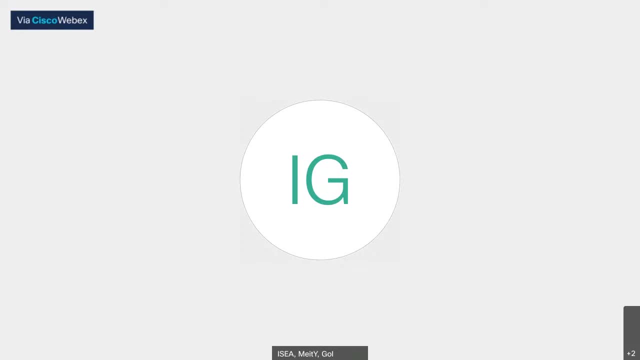 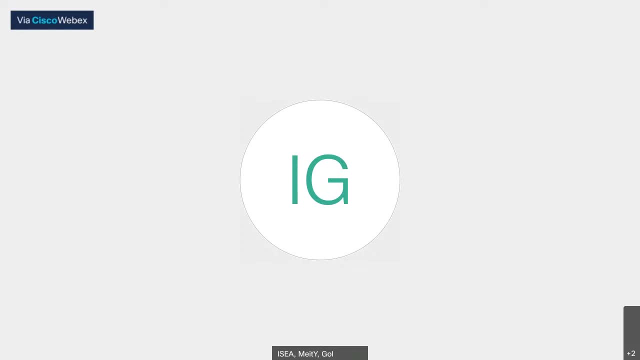 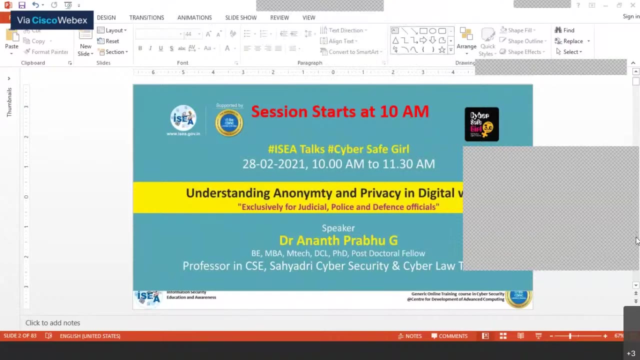 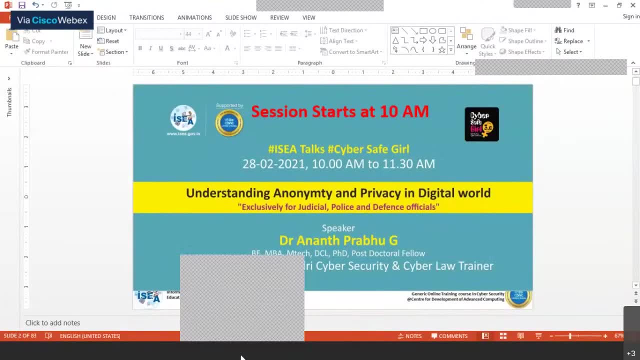 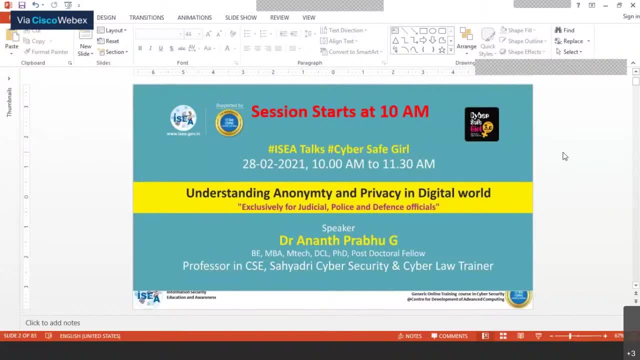 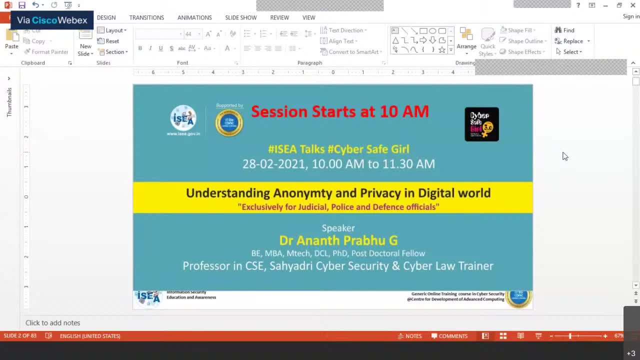 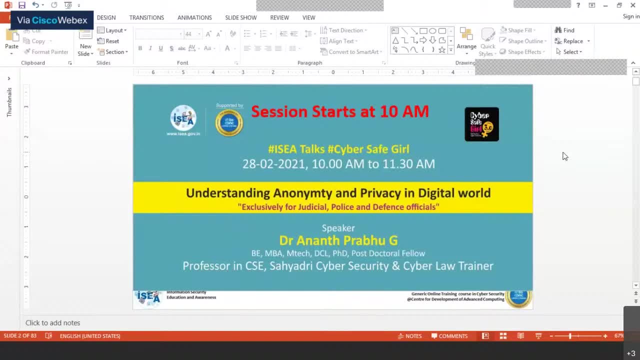 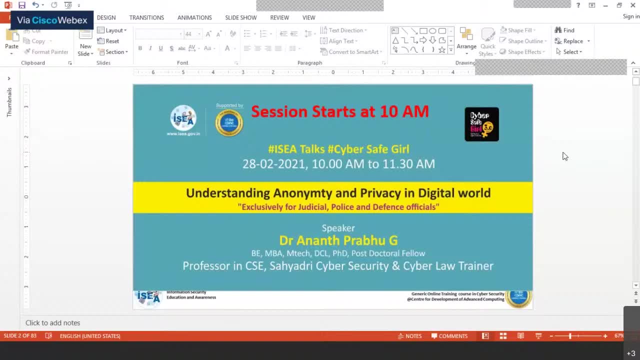 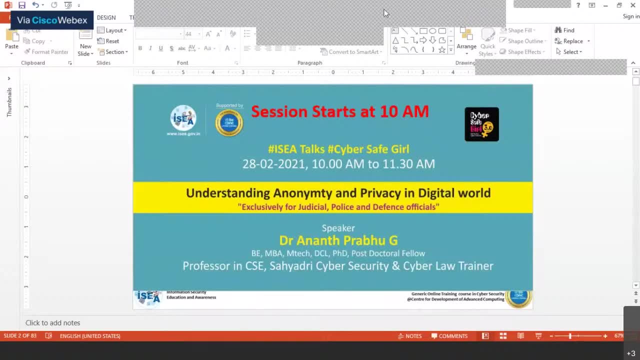 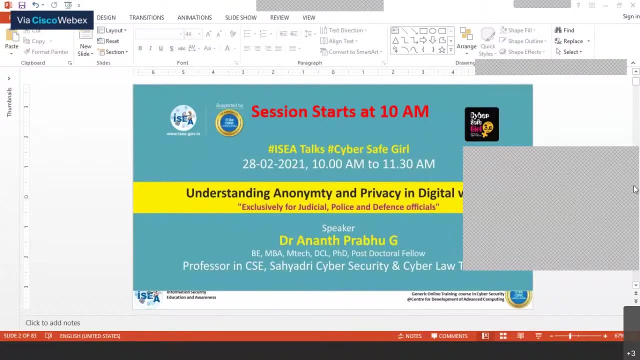 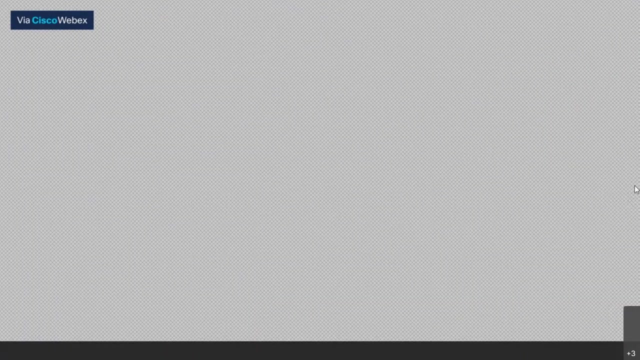 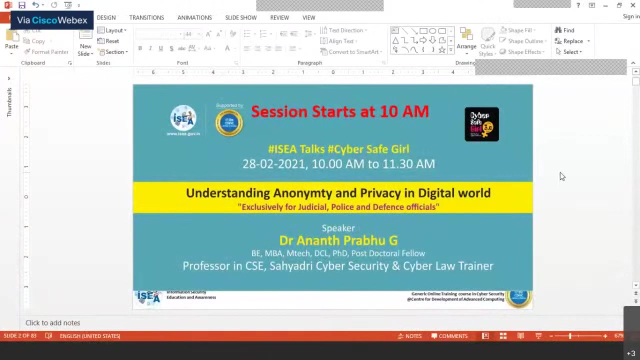 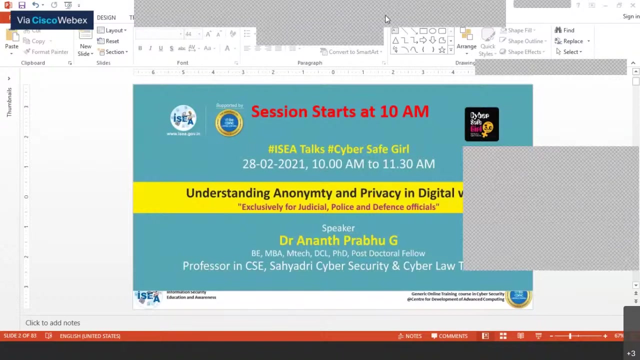 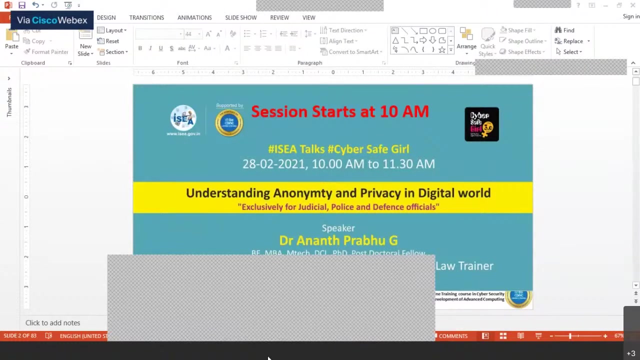 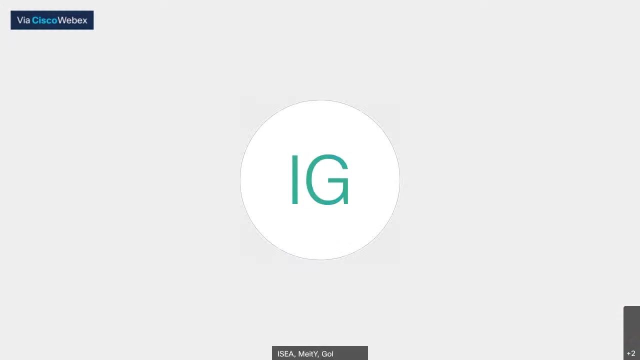 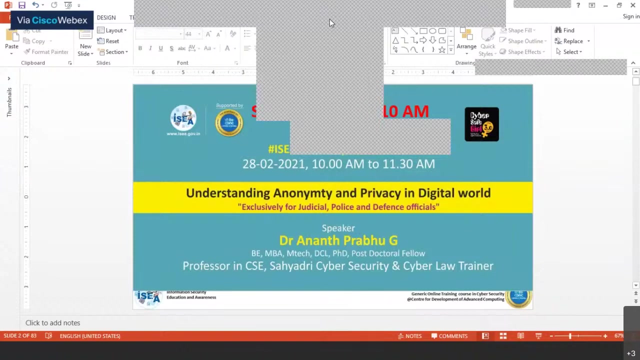 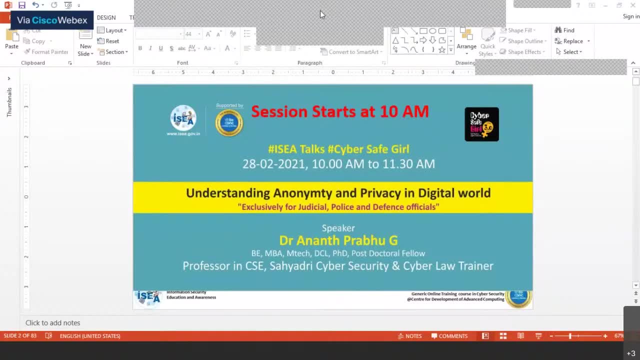 the workshop on understanding anonymity and privacy in digital world. the program is exclusively being conducted for judicial, police and defense officials and I've only welcome all the officials present for this session. the session is basically on privacy related issues and, as you all know, privacy is serious and 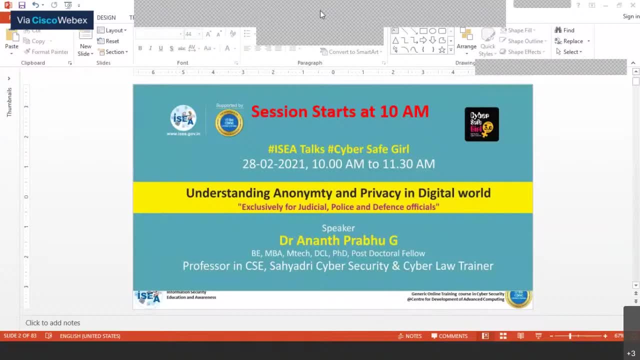 much debated issue currently. in this age of cyber espionage and electronic surveillance, privacy becomes a crucial subject, and this is the focus of the current workshop you that is being conducted in the webinar form. I welcome the guest speaker of today, dr Anand Prabhu. sir, I take the privilege of introducing dr Anand. 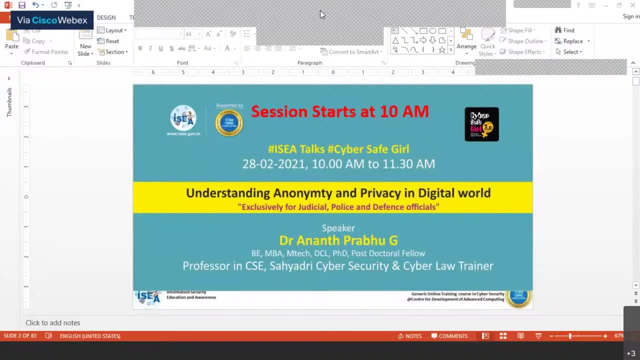 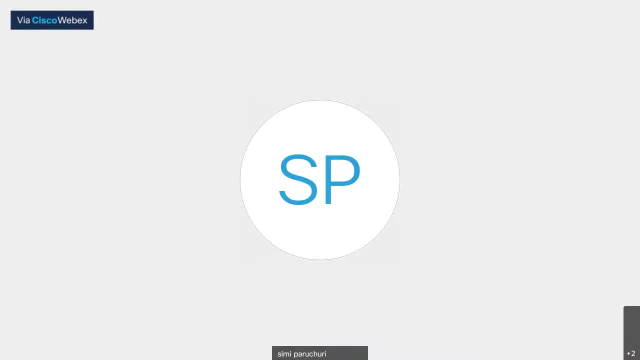 Prabhu, the speaker of today's session. dr Anand Prabhu did his PhD in computer science engineering and he is a post-doctorate fellow in computer science and technology. his current job profile is: he is a professor in department of computer science and engineering. 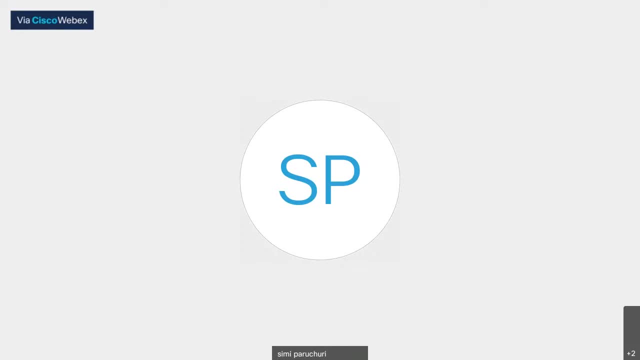 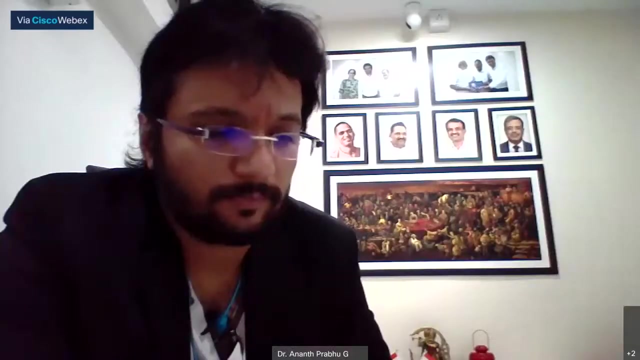 Sahyadri College of engineering and management. his areas of interest include cyber crime investigation and cyber law, and he has conducted more than 1,000 workshops. yeah, he's a trainer for Karnataka Judicial Academy, Bangalore, Karnataka Police Academy, Mysore police training school, Gulburga, Bangalore City Police. 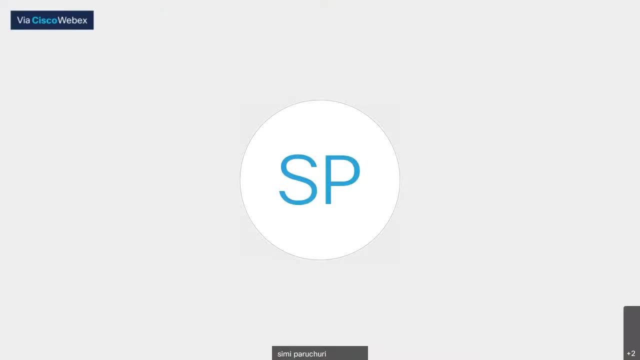 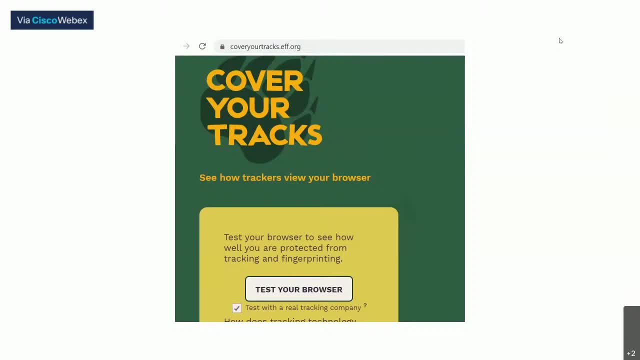 Karnataka police training school: Gulburga, Bangalore City Police. Karnataka police training school: Gulburga, Bangalore City Police. Karnataka police training school- Gulburga, Bangalore City Police thing. i want you to go to google. okay, i want you to go to google and just type cover your tracks. 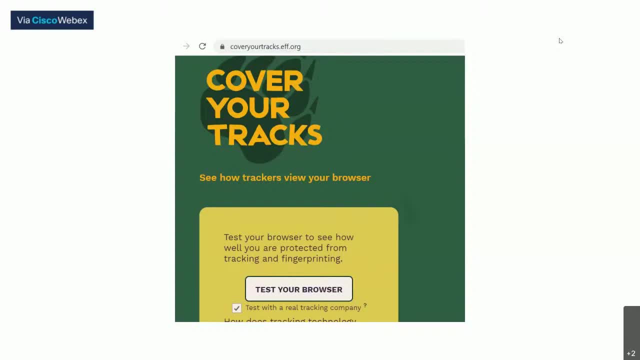 okay, you just type cover your tracks. or you can also type panoptic click- p-a-n-o-p-t-i-c-l-i-c-k. panoptic click. or what you can do is cover your tracks. you just put that. you will get one beautiful website called cover your tracksorg. click on that. now, there you have an option called as test. 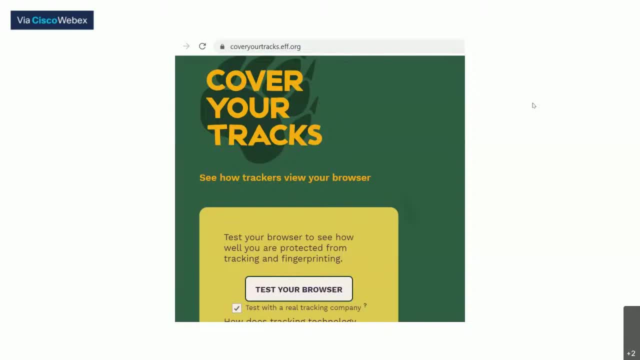 your browser. okay, test your browser, because your browser is a culprit. your browser is the, the tool which gives away so many details about yours to these websites. so you have to be very careful about the browser that you're using, and i tried this today morning on a browser. 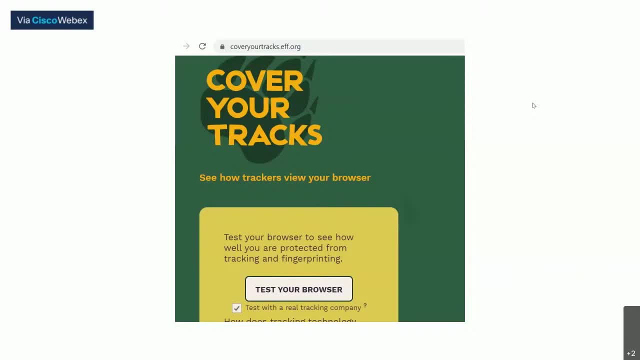 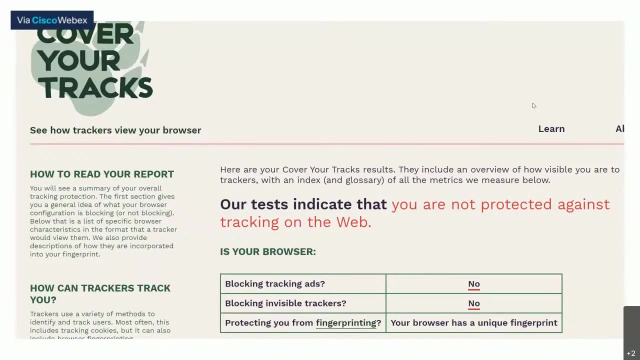 which was from my friend's computer, and see the results that i got. does my browser block tracking ads? no, that means my browser aids for the tracking ads. does my browser block invisible trackers? no, that means my browser is giving away so much of my information from my system to the websites. third one: does your browser protect you from? 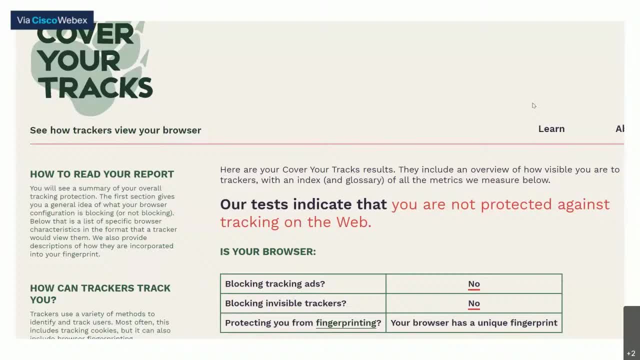 fingerprinting, my browser has a unique fingerprint. when i'm having a unique fingerprint, it means that the websites- whichever websites that i use- they know it is me, because my browser has a unique fingerprint, just like when you log on to the internet, you'll have a unique isp- the internet service provider's ip address. 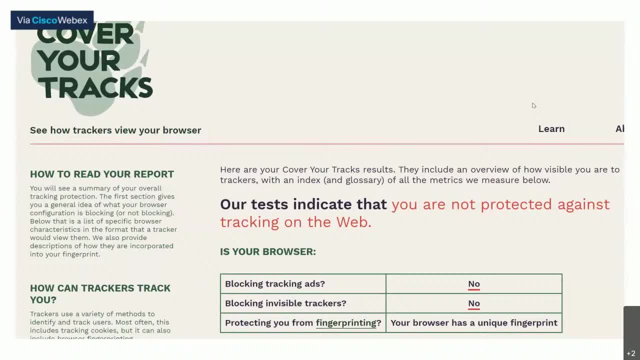 isp, ip address, how it is going to be there. similarly, you will also be having the unique finger print. so please go to this website, all of you, and type cover your tracks. i mean, go to google and type cover your tracks. you will get this website. try it. so this website is going to be a unique fingerprint. 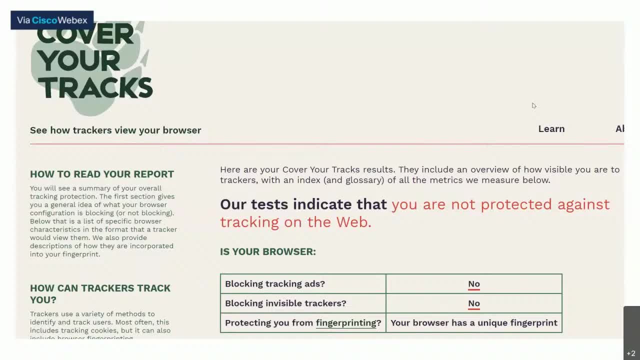 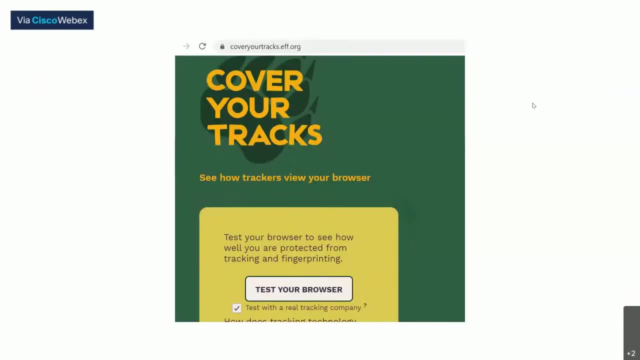 that has the same number of traces as my browser, which means it can be used to do a lot of things apart from tracking the internet. so these are the two assignments that i want to want you to try. this being a one-hour workshop, i'm unable to show everything step by step, but you can do it no big deal here. so the 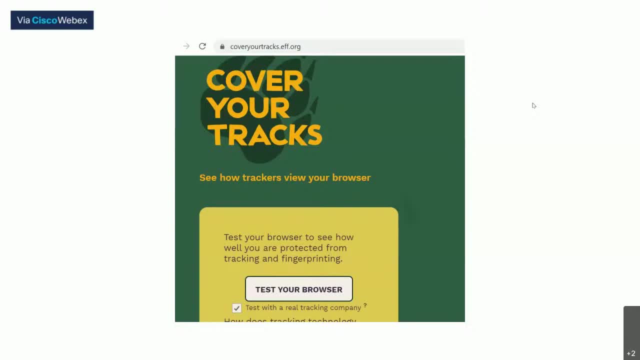 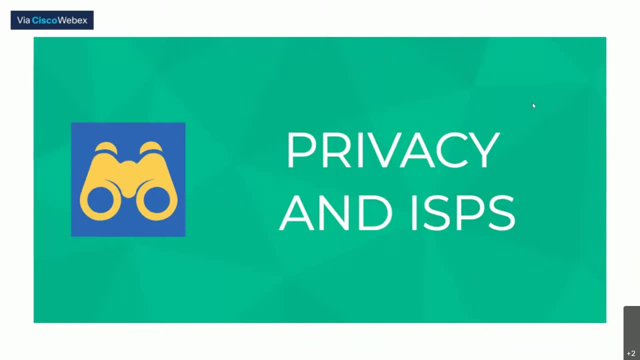 first one was: apply magic sauce. apply magic sauce and you will be seeing it. and the second one is: cover your tracks. cover your tracks will tell you whether your browser is safe or not. all right, okay, very dangerous, my dear friends. they're very, very dangerous, because what your isp can see, if your 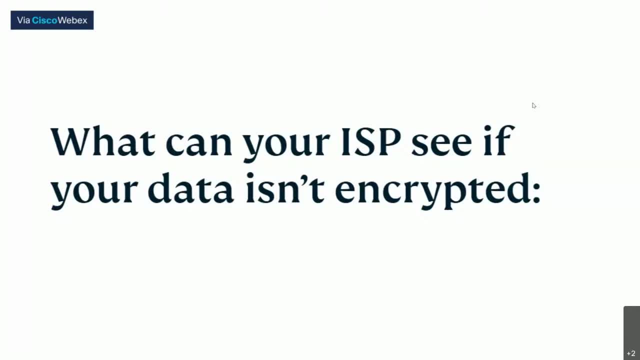 data isn't encrypted. you know that there are two types of data that can go from your computer: one, data as it is, that is, the data that is not encrypted, and the second one, the data that is encrypted. encrypted means you cannot read it. the the decrypted data or the plain text data. 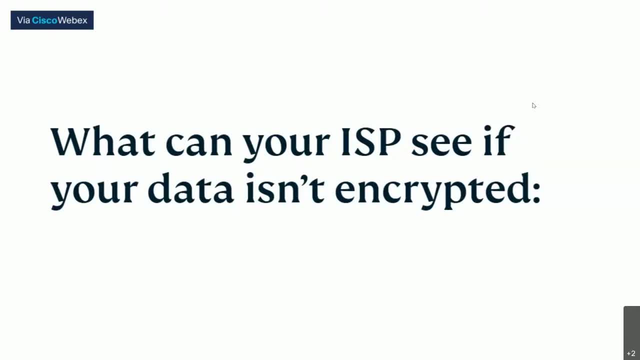 which means anybody can read it. so if i'm going to type my password, my password, if somebody can read it, it is called plain text when i type my password. if, when the data goes from my system, if they're unable to read it, then it is called as encrypted. so as simple as that. so if your data 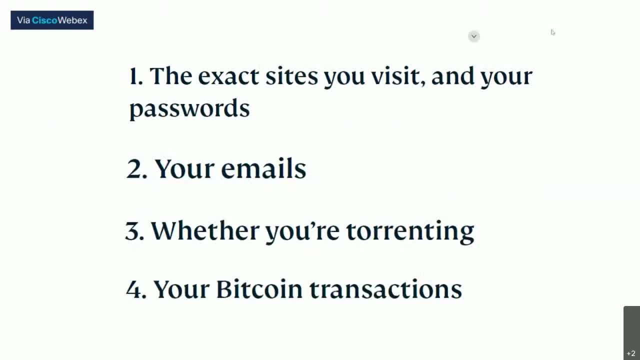 is not encrypted. your isp can know which sites you're visiting, my god, it can know your emails if your email is not transport layer security enabled. and remember, my dear friends, not all emails are tls supported. so if you ask me anand which is the best email service provider in the world, then i would vouch on proton mail. 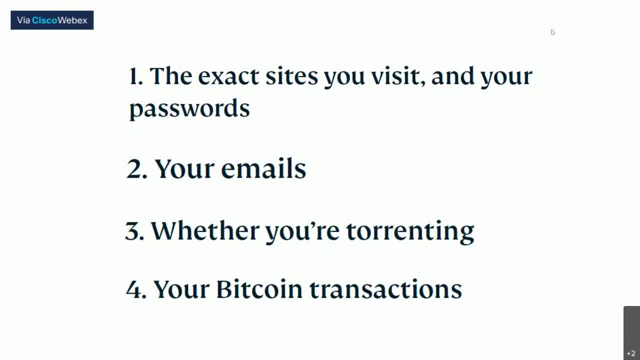 proton mail, okay, and then, uh, vinit prasad. yes, you have rightly said that. i, i appreciate it, okay. third one: if you are using torrents, your isp will get to know that you are using torrents. and, and, my dear friends, even if you are using bitcoins, don't think that you are safe. your isp. 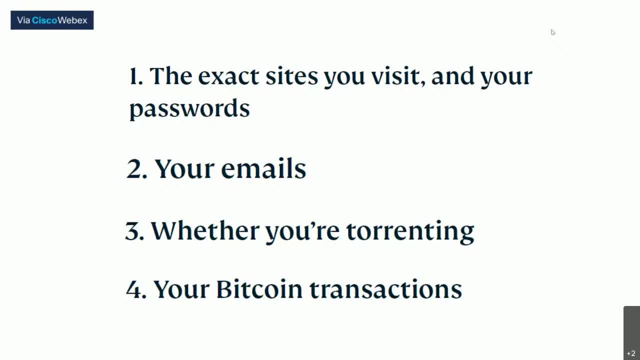 would get to know that you are using bitcoins, because many a times we have understood that people are using bitcoins, who are using bitcoins? criminals are using bitcoins and when you seize their system, even if they tell that they don't use, we know that they are used. so this is how this is, especially for the judicial officers and the police officers. 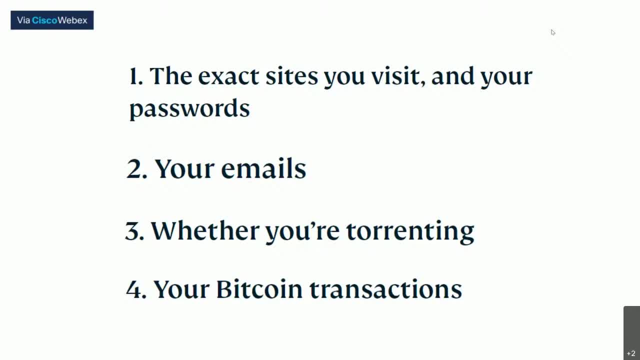 remember, isps get to know all these things. okay, now, now you may be thinking: what will happen if the isp? uh, what will happen to the isp if the, the communication between the, the system that is, the isp, and the server is encrypted? so what happens? but before that, i know that many of you think 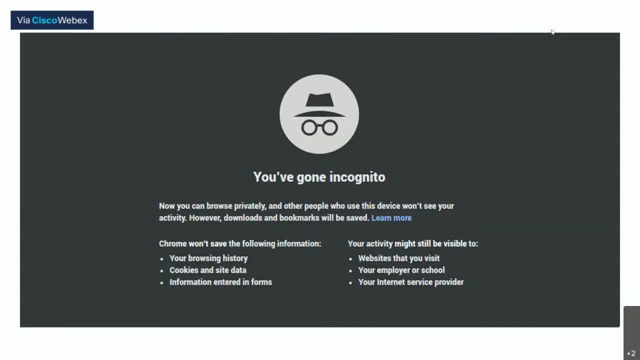 that if i use this- uh, incognito mode on chrome, because chrome is the most favorite browser by most of us, so what we do is we can. we can just press ctrl shift and n- okay, ctrl shift, n- and automatically this black color browser comes, which is called incognito. remember, this is useless. 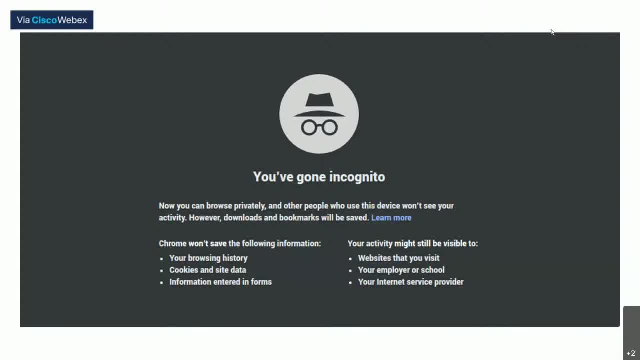 useless mode of the chrome. only thing that can happen is your parents will not get to know what you have done because your browser history does not remain there. that's all, because many times what happens? we browse something and we go out. your parents or your better half or your best half, whatever you call, they can always. 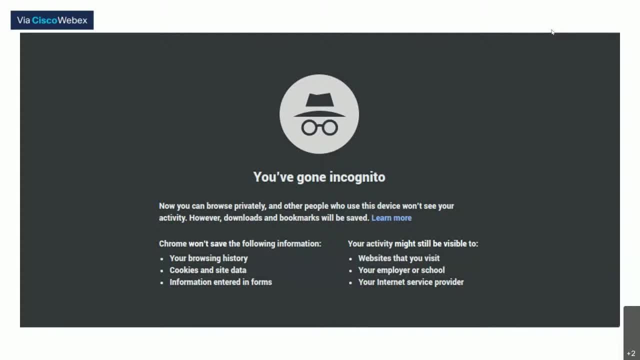 press ctrl h and they will find out which are the sites that you have visited, isn't it? because in the browser history it is going to be there, but here what will happen is browser history is going to get that's all other than that, nothing at all. all right, so now let's see what happens to your isp. 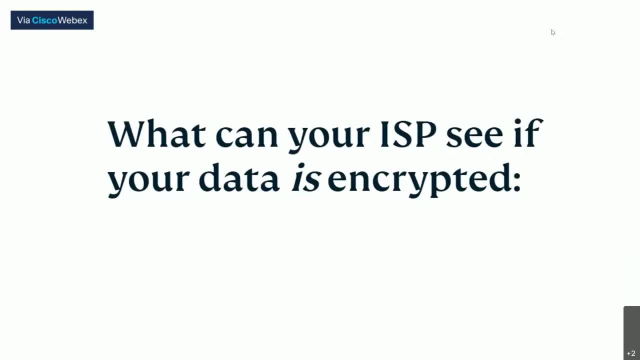 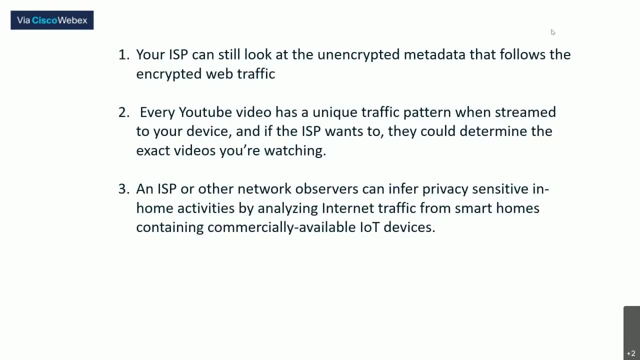 what can they get to know if the data is encrypted? so, if the data is encrypted, if you are under the assumption that if the data is encrypted, the isp gets to see nothing, my dear friends, you are wrong, because if the data is encrypted, still the isp can see the metadata of the websites. you know that data. 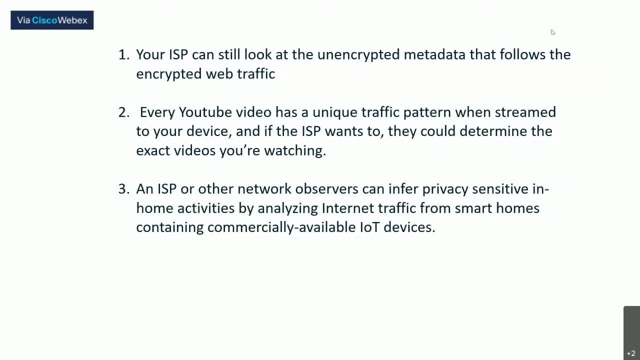 and metadata. data about data is called as a metadata. so, for example, you take a photo- that is example- which camera was used, which was the geo location, what was the aperture, what is the focal length, what is the feather flash was on or off, what is the iso. all these details about that photo data. 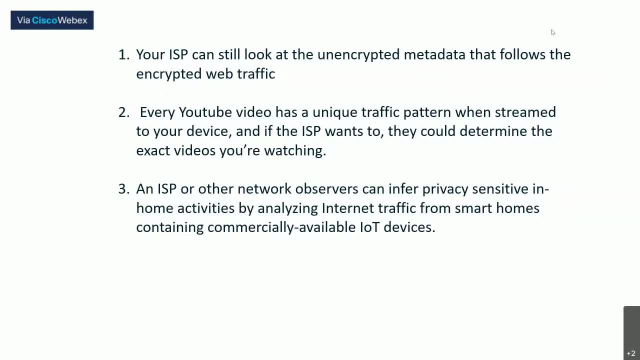 about data is called as metadata. and this metadata, my dear friends, uh, the isp can get to know and they get to know whatever second one, youtube. now, even if you are using youtube, youtube has a very peculiar way of streaming the. youtube has a very particular way of streaming the. 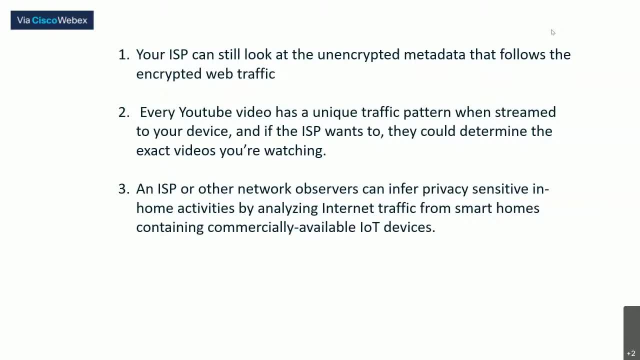 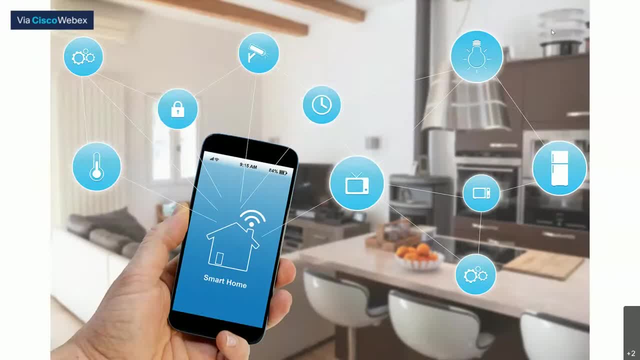 Encrypted content and the can also get to know which is the video on YouTube that you have changed and other sensitive information. because most of us are using smart home and I always tell you know, uh, using smart home is dangerous. Because I feel- I still feel, though I'm in this field of cybersecurity and research for the last 14 years- I still feel we have not reached that level where the smart appliances and everything is absolutely secure. 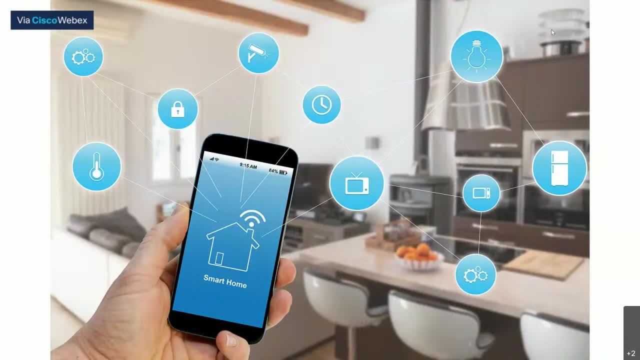 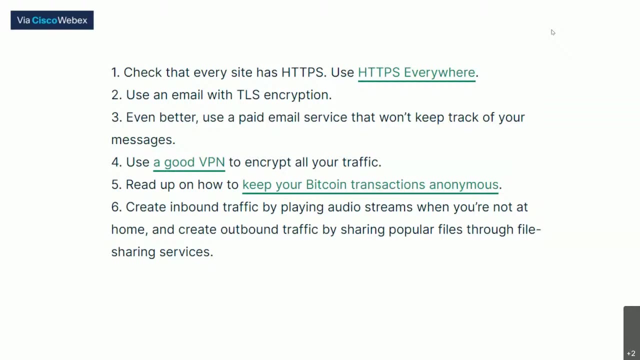 No, we have not. So we are always compromising a lot of things. and the data coming out from the smart homes also can be viewed by the Internet service provider. Okay, So how can you stay safe? So, on your regular way, if you want to stay safe, number 1 is there's an option on a browser called use everywhere, because you know that. 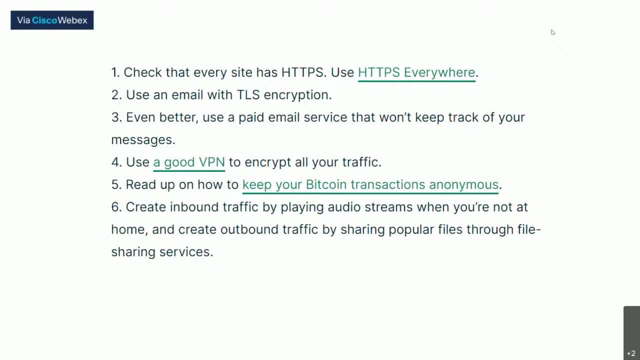 Hypertext transfer protocol and hypertext transfer protocol Secure. so we have these 2 types of this: 1, so use a secure 1 and you're somewhere somewhat protected. Okay, 2nd 1, I said use email with the DLS encryption, but remember both should have, otherwise there is no use. 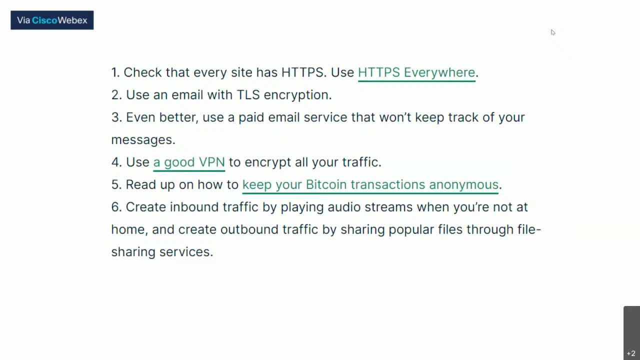 So Uh is transporting security. if possible, use paid email service my difference. because why are emails free? so that they can read your data, so that they can send the advertisers the uh, your uh, what is that? All your details and what you want. 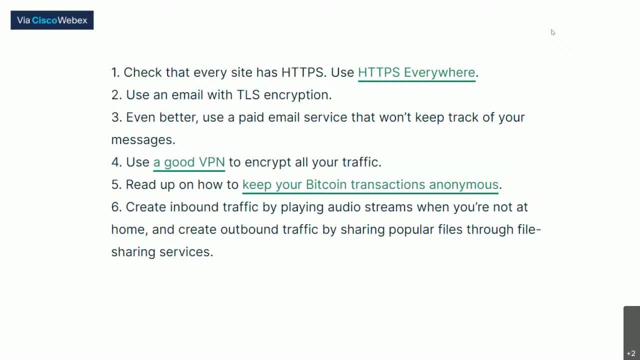 For example, you send an email to your girlfriend telling that let us go for a vacation to Maldives, and the email service provider gets to know that you are interested in models and they will send it to make my trip for booking dot com, or who? uh, what is that? 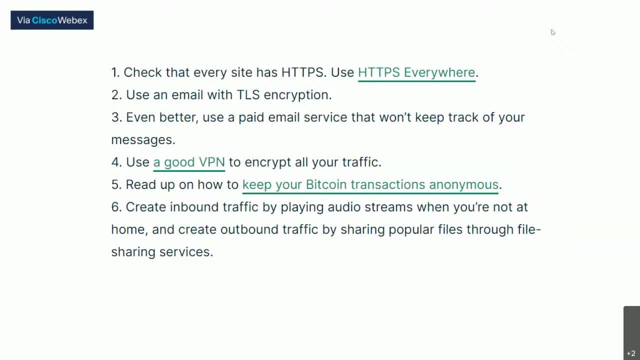 Or your Airbnb and tell that: see, this bugger is interested in models. Keep sending your ads. bomb in with your ads on models and you will keep getting more details. Okay, thank you, Thank you. Thank you, Yes, sir, isn't it So, then? or you can also use a VPN, virtual private network. again, There are 2 types: free and paid. my dear friends, Don't use free, because it is again Very good. 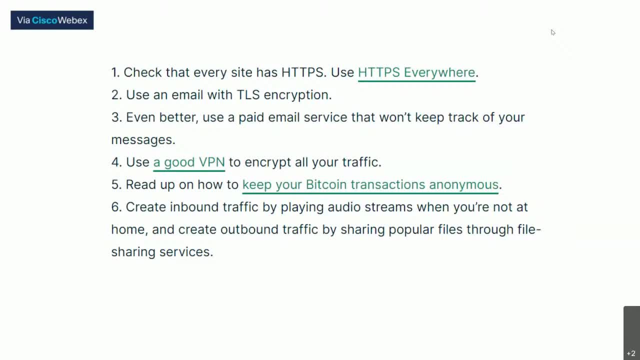 The 3rd. 1 is the 5th. 1 is how to keep your Bitcoin transactions, and all of us will have to check on that. And the last is: keep putting some junk data on your Internet service providers- Always some junk data, because they will not get to the phone and you can play movies. 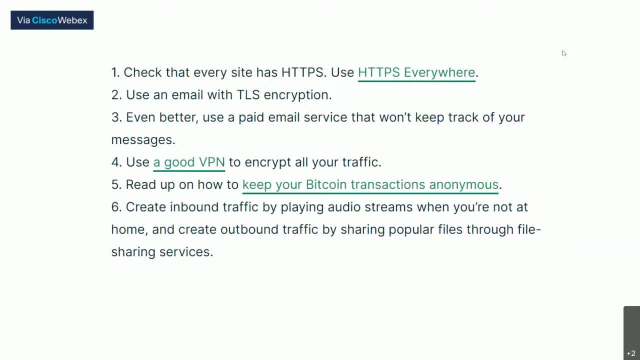 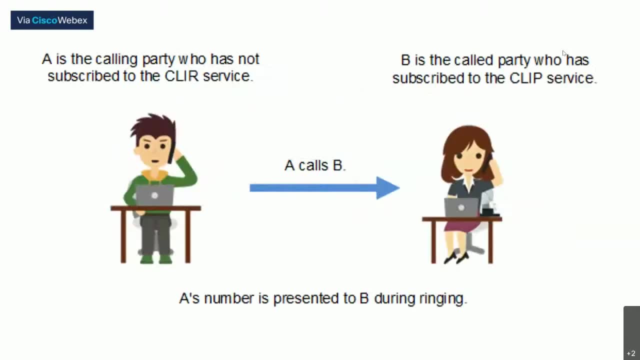 You can play audio, something or the other. You keep on putting Along with it so that the data starts getting not. VPN is very good now you can use. Now look at this. Okay, Look at this. Uh, a calling B. Okay, Is making a phone call to B, so the A's number comes on these phone. 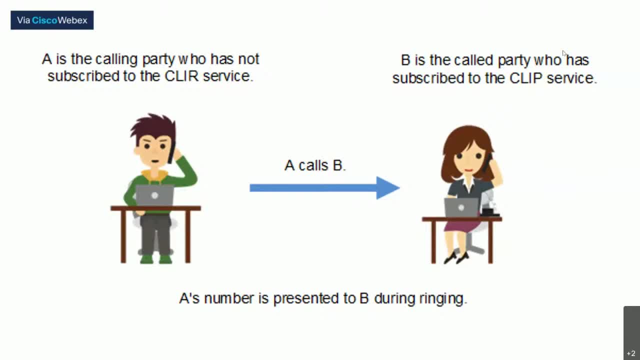 Isn't it? so if the A's got, then it will come as a private number calling. Mr got many times call from private number calling while the he is using wipe, He can show whatever number he wants. If you want to, You can call him. 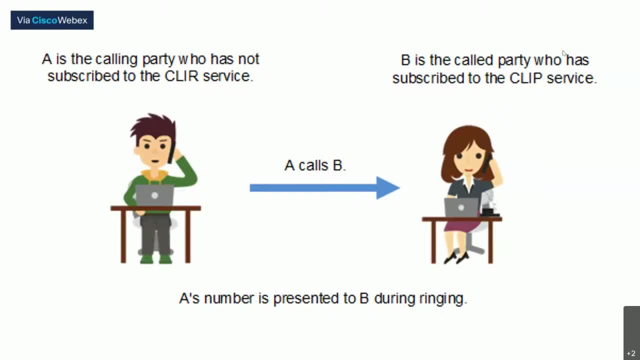 Sorry, sir, I don't know. We can, I don't know, I don't know. you can show b's number on b, only you show like b is calling b. so this can be done. but the point that i want to say is: a is calling b, so they make a phone call, okay. so when they make a phone call, 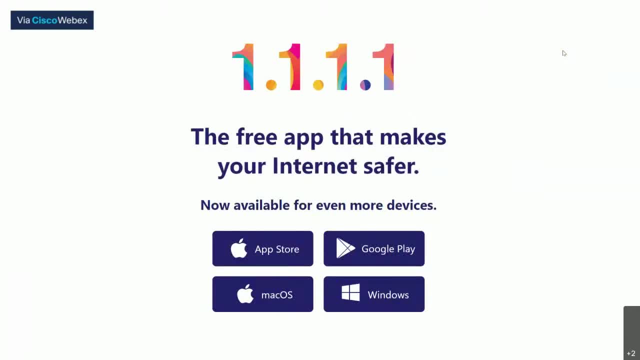 you know that. you know that when you take your phone, when you take your phone, if you say anant prabu, okay, anant prabu is easier to remember than anant prabu's mobile number. okay, in my case, i know my mobile number is very easy for you to remember because, uh, that's a fancy number. but 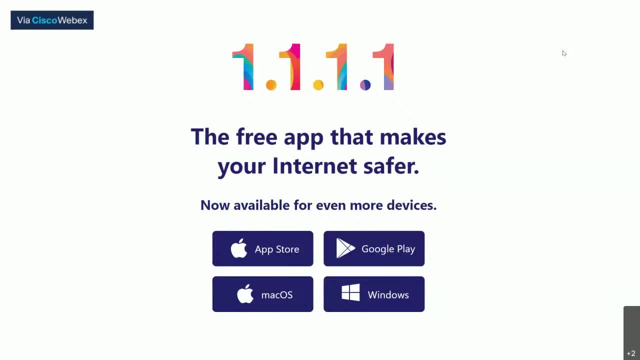 otherwise. otherwise, let us assume that my mobile number is double nine eight, six zero eight nine one, nine four. this is my mobile number now it is easier for you to remember, anant prabu. or double nine eight six zero eight nine one, nine three. i know that it is easier to remember. 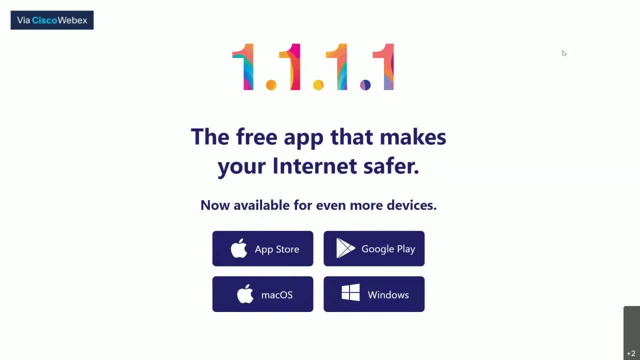 now, what will happen is, my dear friend, for you to remember my name, anant prabu, you have to go to the contacts in your phone. go to contact, search anant prabu. when you search anant prabu, you will get the mobile number and then you press call button and the call comes to me. a to b. 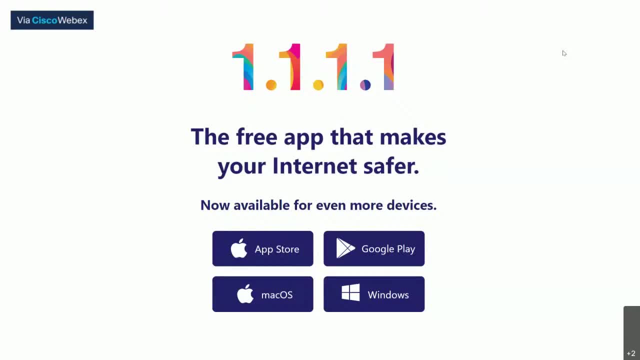 similarly, if you want to go to facebook or google or yahoo or any of the websites, you want to go any website. you don't have to remember the ip address, because connection between two computers is my ip address. connection between two phones is my cell phone number, isn't it so? 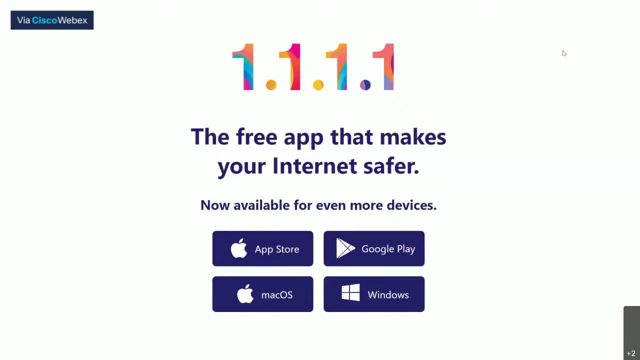 so ip address you can't remember. therefore, there is one computer in your network, in the internet service provider usually, or external also, which is called dns. dns stands for domain name server. okay, so now in the domain name server, what it does is whenever you want to connect to facebook, you will go to dns first. okay, dns will give you the ip address of. 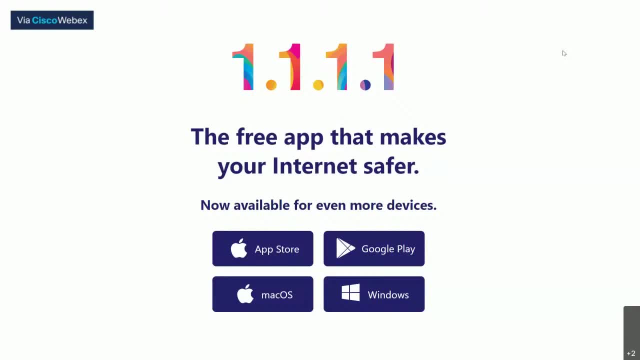 facebook and then the dns. what it will do is the dns will give you the address, ip address. using that ip address, you will connect to the server. simple as simple as that. now what if this dns is tracking on you or that connection to the dns is not usually using https? 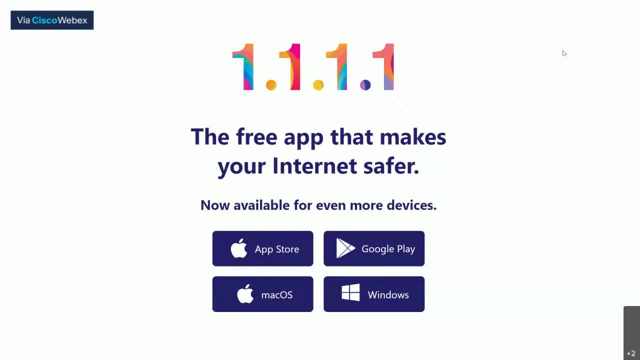 connection to the server facebook is https, but connection to dns is not https. therefore, this is one very beautiful service called dns over https, so you can all download this feature. all you need to do is go to the browser and type 1.1.1.1. okay, i repeat, 1.1.1.1. you type and they have this. 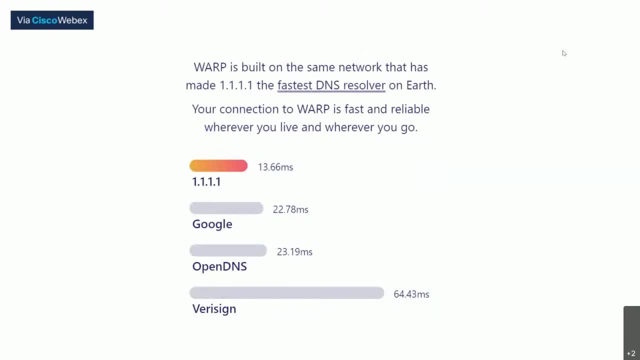 fantastic feature called warp. so warp is one of the fastest dns resolvers in the world and it's faster than google, faster than open dns, faster than very same. but the beauty of this is it is over https, yes, so it is one of the dns that is safe and secure, so i want you to use this dns. 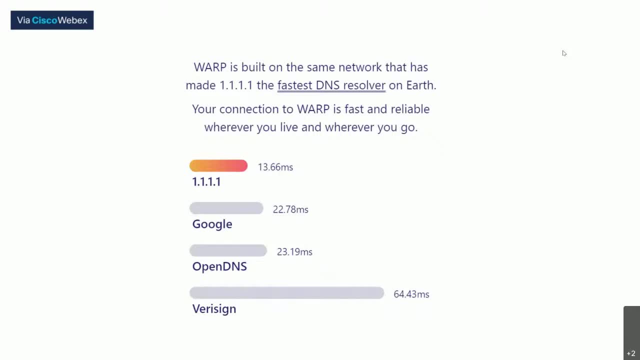 because whatever you are trying to do, if your dn is the first step policy from here, you're going from outside your house, the first step. when you keep wrong step, then what is the use? so, therefore, the first step should be proper. therefore, you need to make sure that this particular thing is what 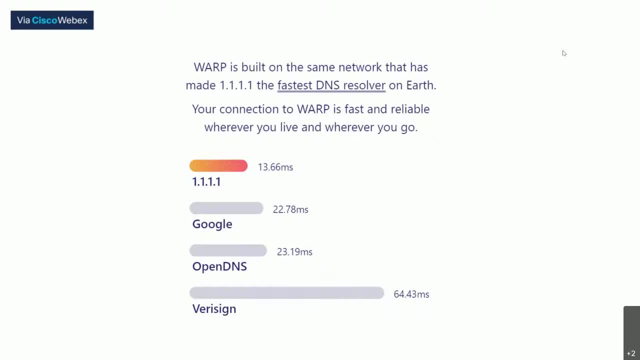 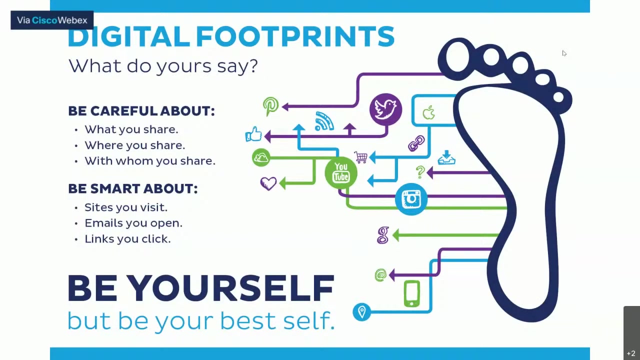 dns is over https. okay, so somebody has asked a question, md after. i think he's my friend. uh, if the same person, good morning. but anyways, if it is not no problem, good morning to you also, but then, yes, i will be sharing the ppd too. so digital footprint, so digital footprints we need. 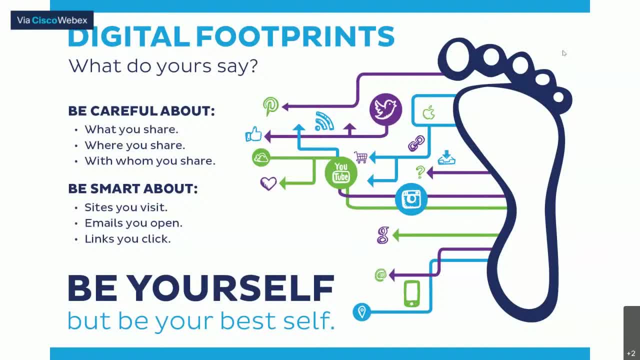 to be very careful about, because what you share, where you share, with whom you share, all the footprints are left. if you feel that, no, you are james bond. or if you feel your sherlock's own, no, not at all, you can't be anybody, because whatever you do, somewhere or the other, you will be leaving the footprints, and i want the. 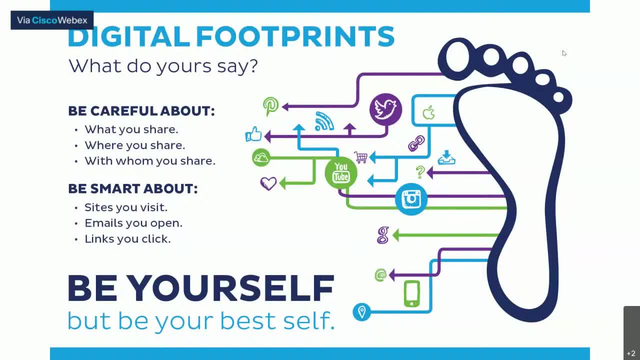 law enforcement agencies to identify where these footprints are left so that you can catch the accused. you can track the use that you can put in behind the back. so be yourself, but be your best self. so this is because you need to be smart about the sites you visit, the emails you open and the 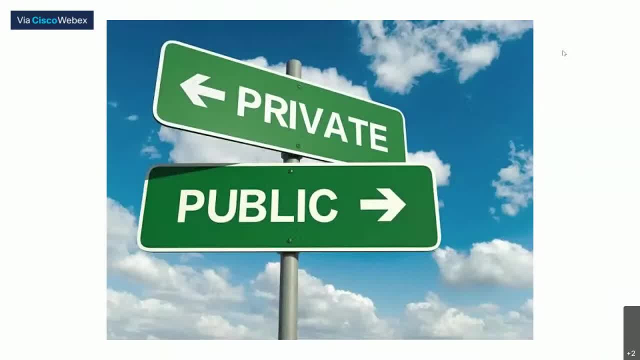 links you click, because all of us have got two lives: private life and public life. so is there anybody here in the audience? is there anybody here who can tell me anand sir, you please take my mobile phone and do whatever you want. you can open any chat, you can open the gallery, you can open any folder. is there anybody here who has 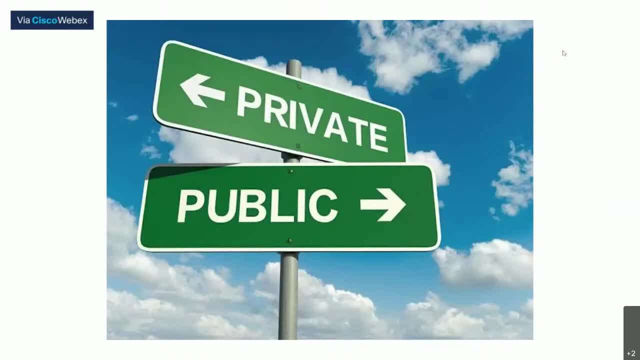 got that much, uh, that type of freedom where you can tell that my life is open. i don't have anything private on my phone. no, even i am not there. even i would not give my phone to anybody. if there is anybody put: yes, i am there, i will sit from here only and open your phone. is there anybody? nobody. 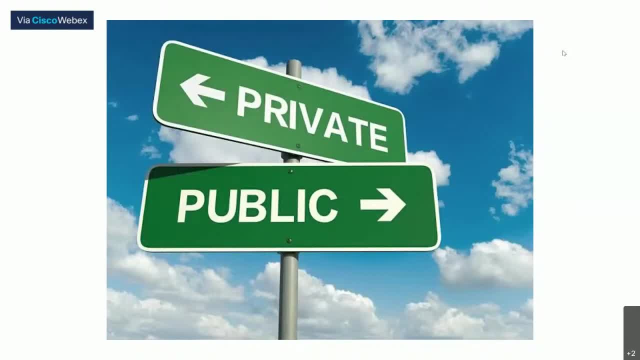 is there. so that is how it is. that is natural, because everybody has got a public life and private life, and private life is a public life and the problem happens when the public life becomes what? public only? and the private life becomes public. if the public life is public, there is no. 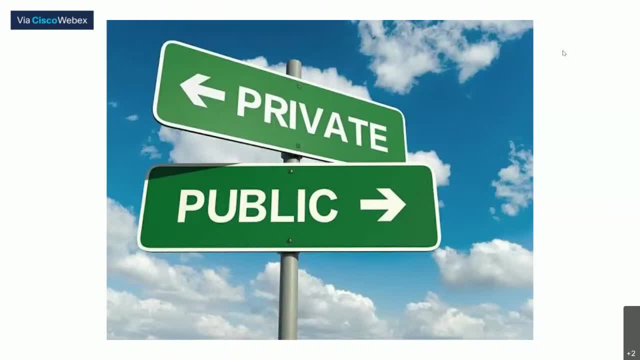 problem. but when the private life becomes public, that is where the problem starts. see one photo that you have clicked exclusively for your girlfriend. that's a private life that, if it goes on facebook, what will happen? it will become public. your life will become terrible. so you have. 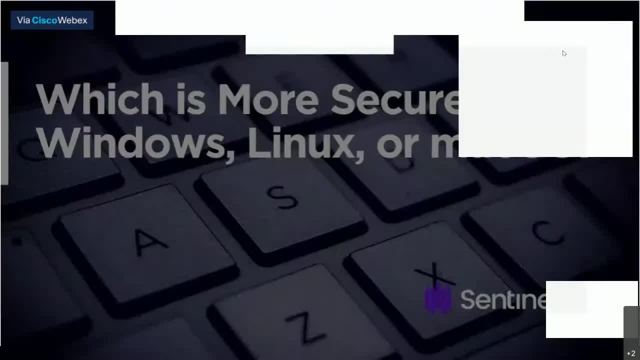 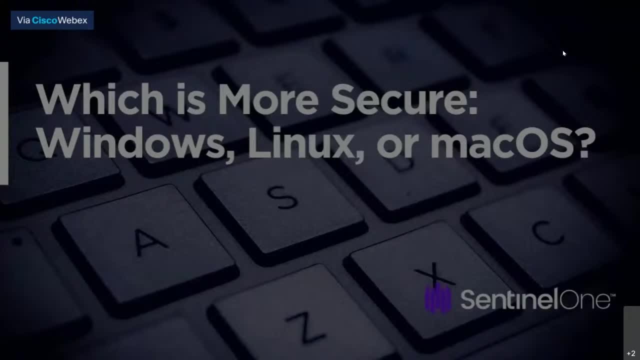 to be very careful about that, because you need to know what should be secure and what should be. all of you can answer it: which is more secure: windows, linux or macintosh? quick, let's see who's going to answer. windows- all are exposed. mac- good, okay, so i'm getting some answers. linux: super. 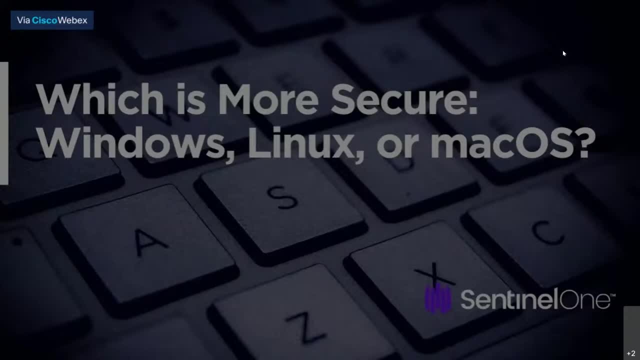 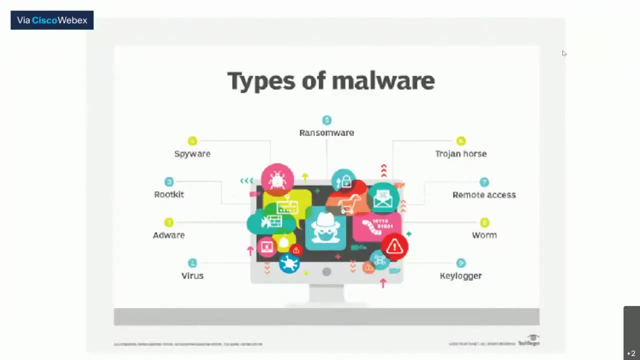 superb mac, mac, linux, windows. i'm so happy that nobody's selling windows. very good could be any. okay, let's see. because because, uh, i always tell uh the other day i think you must have all got the messages telling that, um, the good morning message that you get, you should be very careful. yes, you are right. 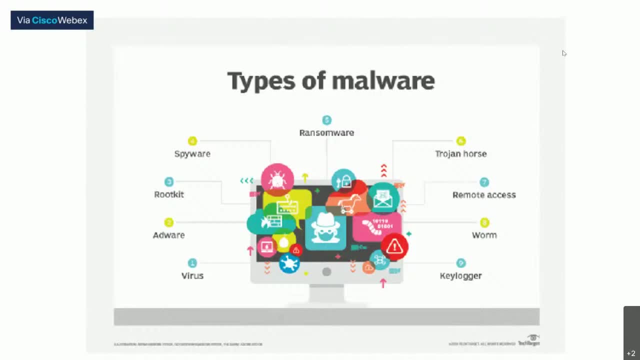 because most of the good morning messages are progen horses. i repeat: progen horses. progen horses means message looks like good morning, but inside that there will be a malware, so that that message, when it comes to your computer or when it comes to your mobile phone, if you do not have an anti-virus on your mobile phone, that virus or malware will get installed. 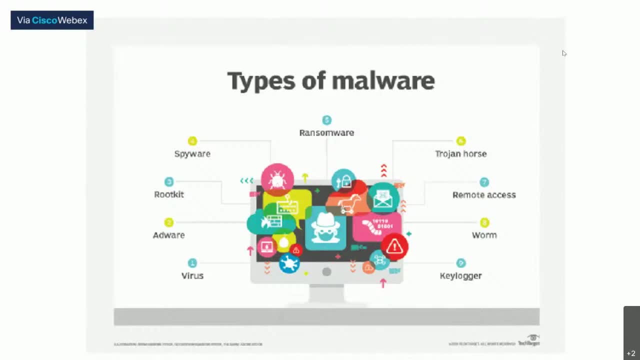 on your computer and then on your mobile phone, and then you are susceptible. so, This Trojan, you must have seen the Troy movie, where two kingdoms fight with each other, one and the other, fighting, fighting, fighting, And finally, what will happen is they know that if we keep fighting, all of us will die. 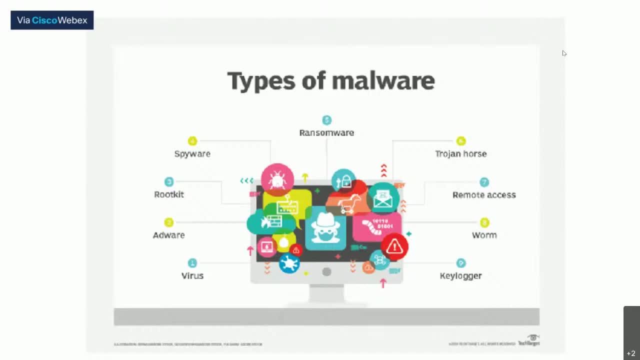 So they will come for a compromise truce and one king will give the other one a big horse, a wooden horse, and the king will keep it in the center of the city At night. what will happen? Horse will open and all those soldiers who are inside the horse will come out and kill everybody. 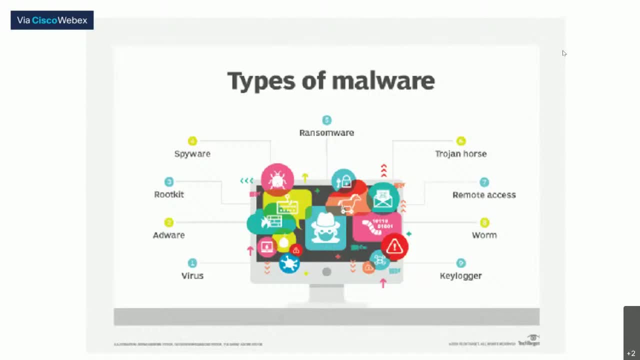 So the name of that horse is Trojan Horse is not the problem. What is inside the horse is the problem. Inside the horse, what was there? The soldiers were there. Similarly, inside this you may get a good morning message of Sunny Leone. 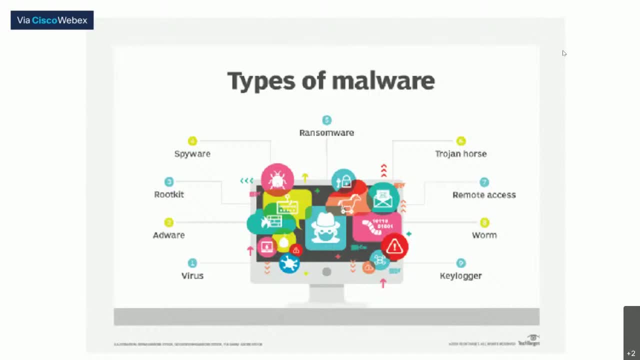 So good morning and very happy All are seeing. oh, Sunny Leone's photo has come. Good morning, Sunny Leone is not the problem. Problem is, who is there inside Sunny Leone. So it might be a malware. It might be a malware which will switch on your front camera and back camera without your consent. 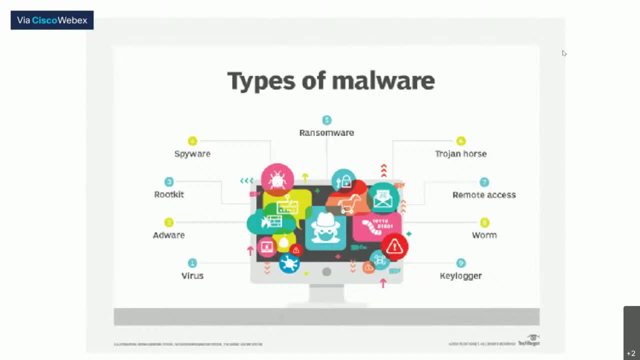 For example, you go to the bathroom, you take your phone. You go to the bedroom, you take your phone. You go to the changing room, you take the phone. What will happen? It will start According. you will not know possible, or it can be a key logger. 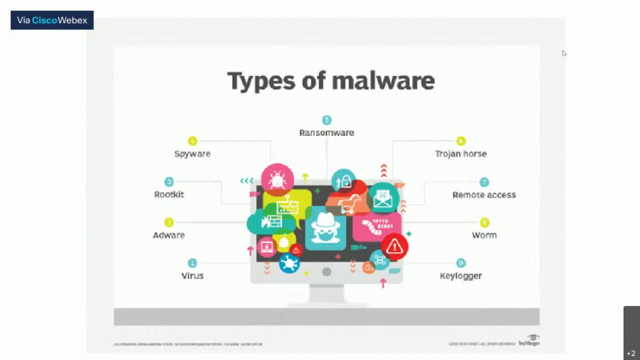 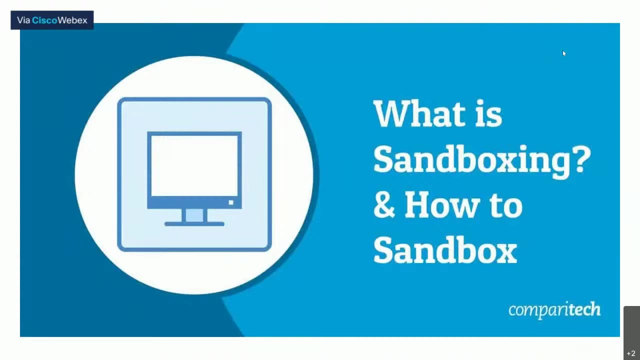 So, whatever you take, one copy goes to the person who are sending it, isn't it? You get your password, you get your UPA, you get everything. So be very careful. And why I always tell that Linux is more safer than Windows is because Linux has got one concept called a sandboxing. 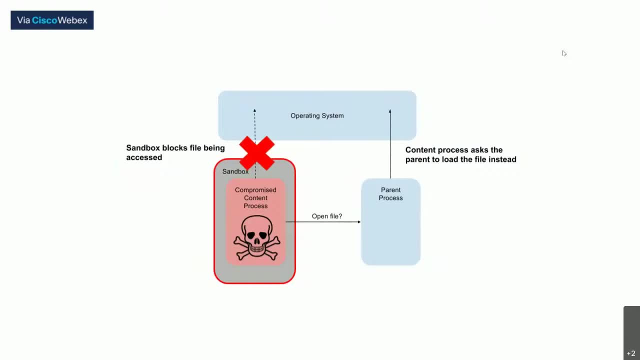 Sandboxing. basically what happens if you install something, it will give a memory to that, exclusively to that, so that even if it is a malware, even if it is a dangerous process, It cannot access other processes because it is restricted to that area only. 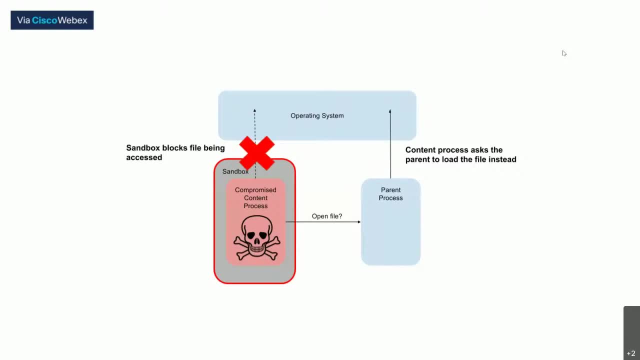 So that level of protection is called a sandboxing, which is not a many operating systems offer. Therefore, I always said: if anybody asks me, why is Linux? but I said Linux is supporting sandboxing and because of sandbox we get an extra level or the best level of protection. 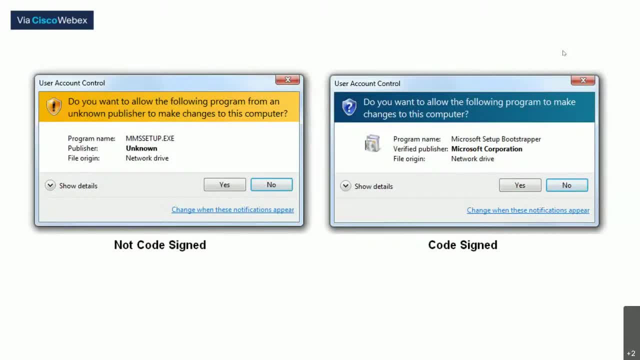 And in Windows usually you get this whenever a software is there. If the software is not signed by the software, By Windows, then you get: it is an unknown publisher. Be careful. If it is signed, it means they know that it is. uh, it has been checked by Windows. So, but how many of us check this? Uh, very seriously, You don't anything. Yes, Yes, Yes, Yes. We go on pressing Yes And uh, what will happen? 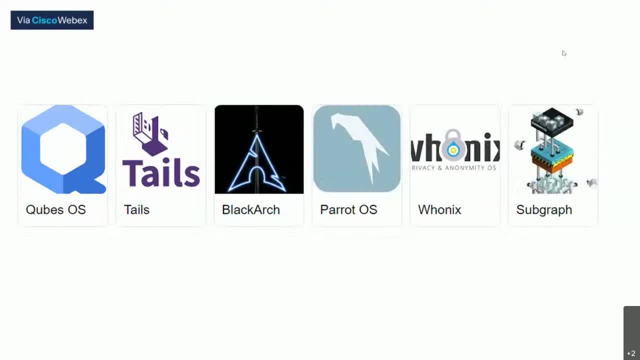 We will become the victim. so if you ask me- uh, that question again- which is the best operating system, I would say The safe and secure cubes. They use Blackhawk Who? next subject, not in any particular order, but these are the safe and secure operating systems. but today we'll be talking about 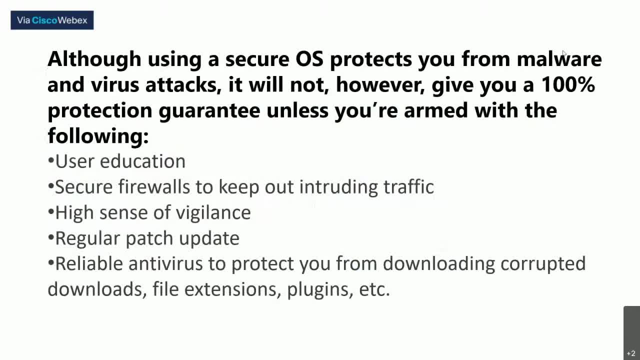 Okay after some time. so, uh, although using a secure operating system protects you, but then still, if you're not aware, if you don't use proper firewalls, and if you don't have proper vigilance and you don't have an antivirus and all that, then it is again dangerous. Only, it is like you know. there is a scene where, if there is a monkey and you give the monkey 1.. 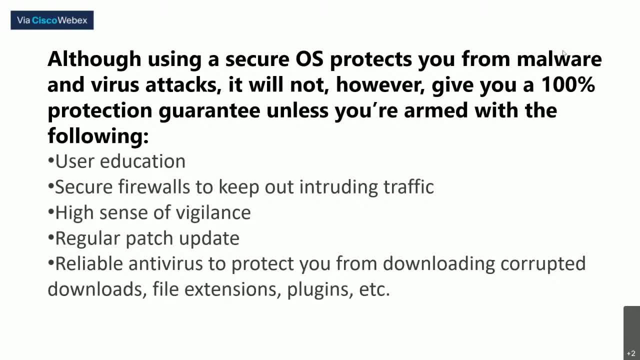 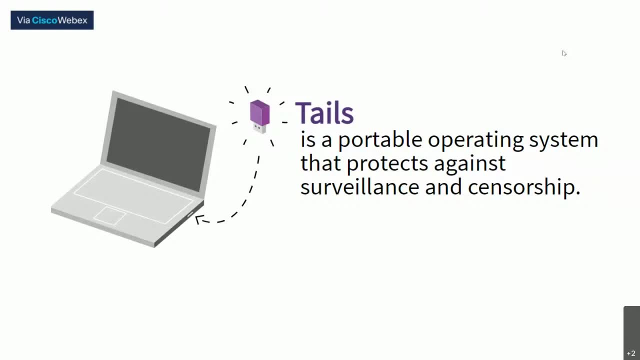 You know, you give a precious tool to the monkey- what the monkey will take and throw it. So we have to be very careful, We need to be alert and the operating system that we're going to talk about is for us. So the operating system, which is a very beautiful operating system that protects you against surveillance and censorship, Okay, And this is how it looks- beautiful It is. 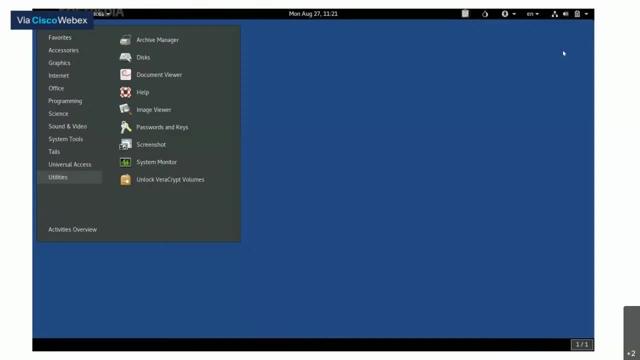 Got um. What is that? graphical user interface? Because earlier people used to not like Linux because it was um. you know the there was no good, isn't it So? so it was more of a command prompt based. command prompt based. 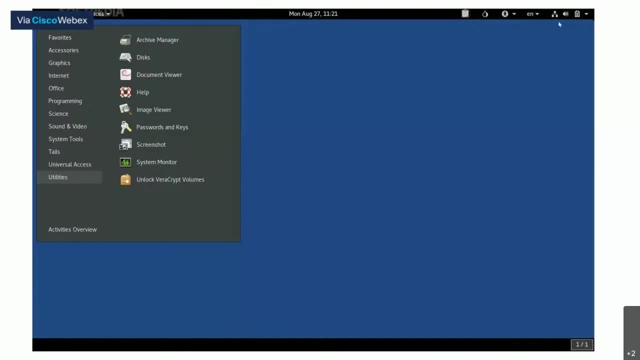 But now it is. uh, you have a graphical user interface, so it looks like Linux. Yes, it does. Yeah, I'm checking the comments, but I will come back to it in some time. But, um, if at all it goes with the sync, I'll immediately just pull it and I will tell it. Okay, So don't worry. 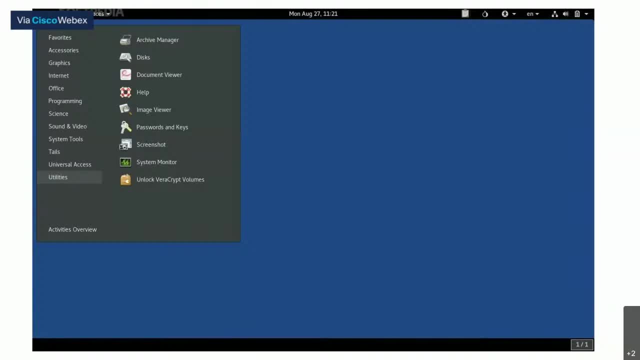 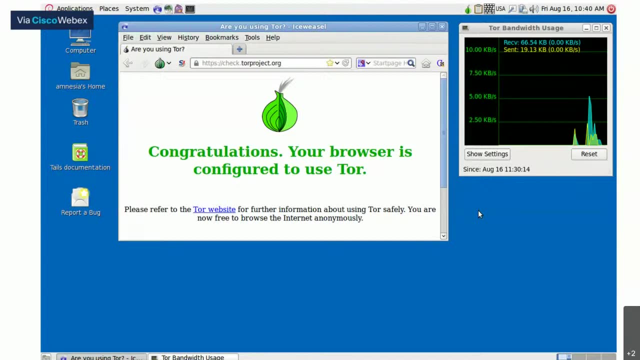 So, uh, this is um the change. operating system, beautiful operating system, Why I love it so much. I will tell you something else. comes with the top browser, Okay, And usually the activists, the journalists, the domestic violence of us. 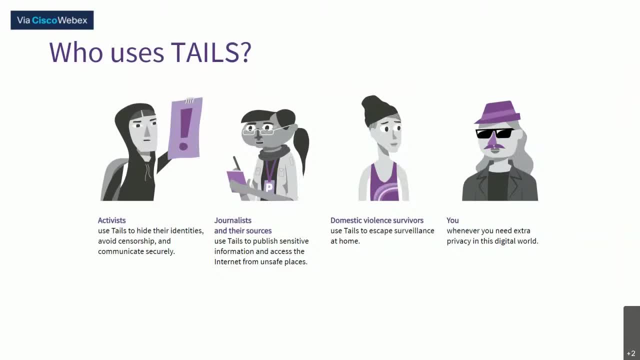 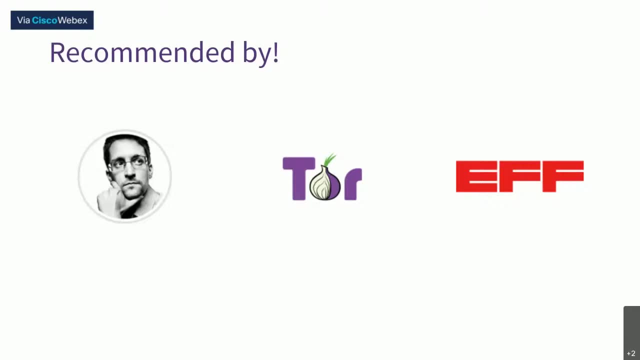 And uh, you, you can also use it. So if you ask who is the state, everybody can use it and it is recommended by the 1st year. Who's the 1st guy? Anybody? Let's see who's going to have the quick. Who's the 1st guy? 1st guy in the picture? 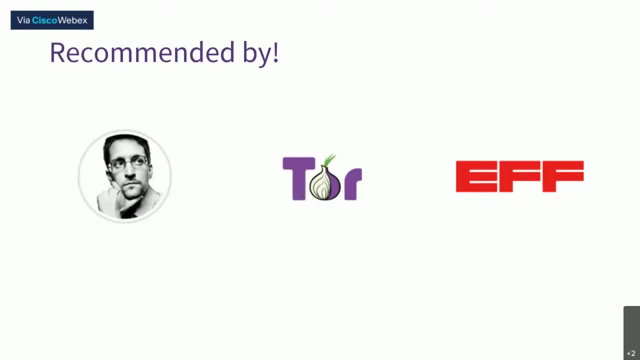 This is recommended by who? who is he not getting answers? Uh yeah, it's. it's Edward, absolutely, Absolutely, It's Edward stored in. Edward Snowden is a guy who, uh, came out with this wonderful project called WikiLeaks, who gave sleepless nights to many governments and many people. 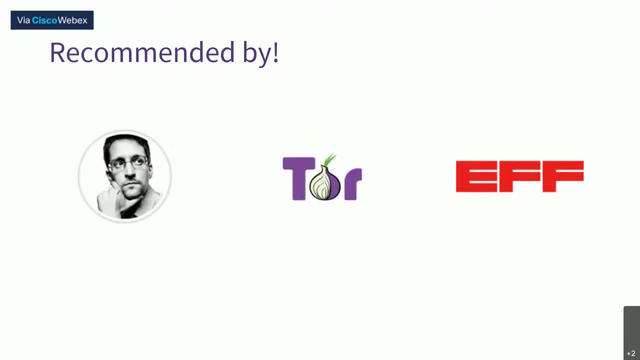 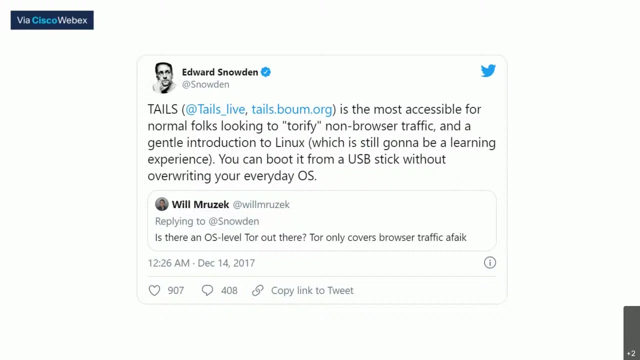 So Edward stored in, recommends it. um, it's recommended by car and it's the electronic frontier Also. So, uh see, what has uh Edward Snowden has said? Edward Snowden has said that it is a fantastic operating system And uh, somebody asked him. 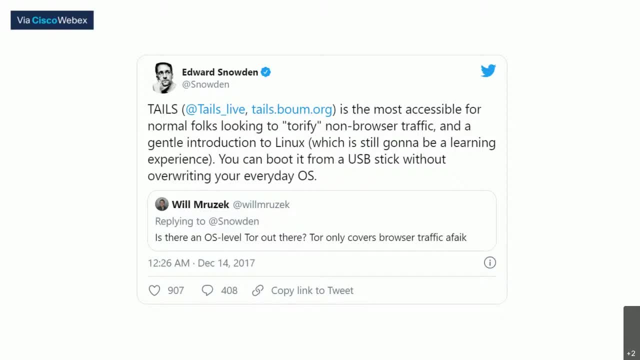 Uh, it doesn't use only top browser or all the connections from the operating system is based. Yes, it is So. uh, not only the top browser connection, but anything that goes out of uh uh days is also, so we call that as. 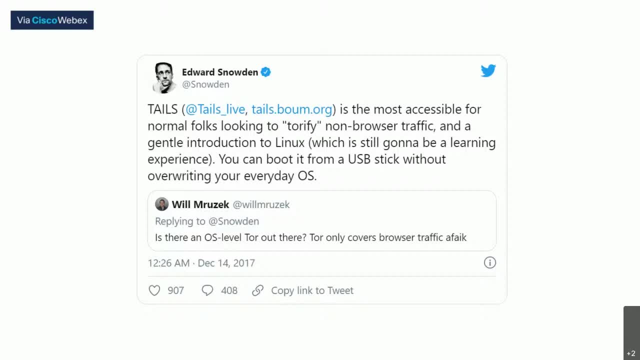 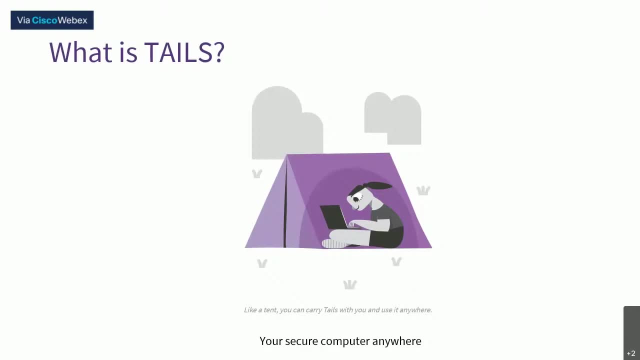 Always level. I repeat, always level. So we'll see more on it in some time. So this is a computer that you can use it anywhere. You can use it anywhere. Now why we can use it anywhere? Uh, look at this, Okay, Uh, you have. now you come to my office. you come to my office and you switch on my computer and then it is windows. You want to use case? No problem, You can still use it. 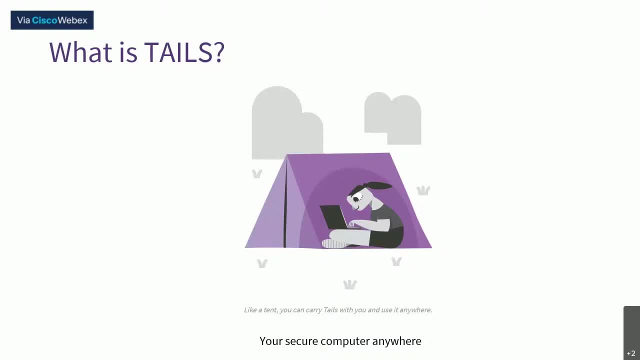 How we can in America. Okay, So teams can be used anywhere. Tails has got ammunition, which means, whatever you do with that operating system, It does not Now windows what you have done in the last session. you log in again. you remember what you've done. 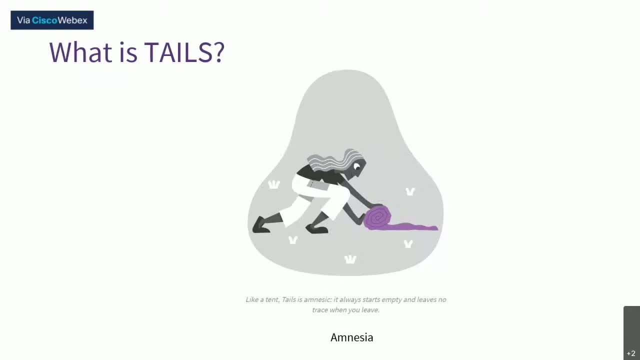 You remember which are the, what are the activities you have done, which are the plug and play devices that you've connected? Because the other day, uh the case is, somebody, uh 1 student, went to a college computer and put the pen drive and said, and uh put the question. 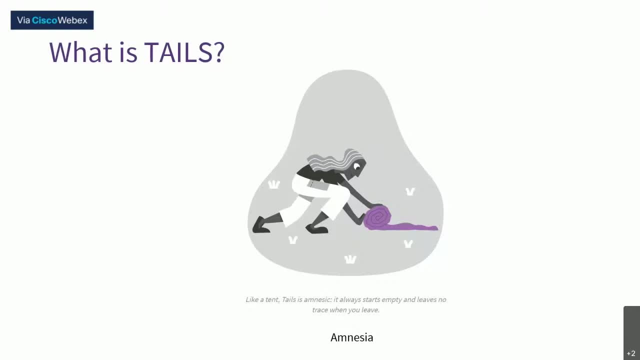 And then he was arguing that it is not him. He said yes, it is him, because we found the pendrive. So the pendrive has got a unique signature and in your computer when you put the pendrive or any plug and play device you put, the operating system remembers. Okay. 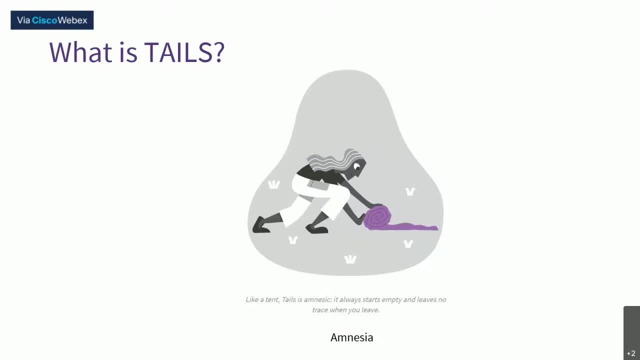 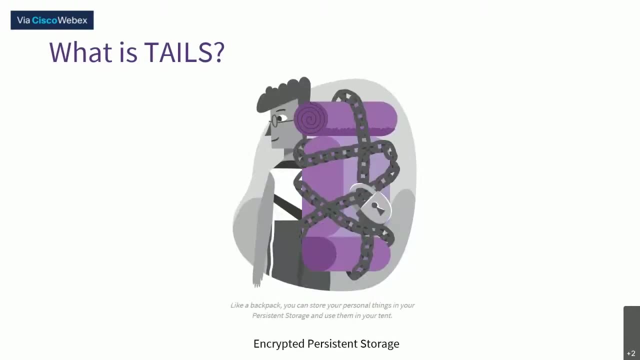 So this is how it is in most of the operating system and that is very good. But in tails it does not remember. So what you don't remember, we call that. So tails is sick And tails has got its own storage. It does not use the storage of the computer. 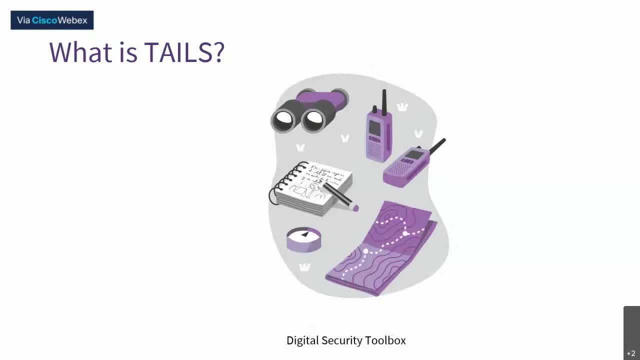 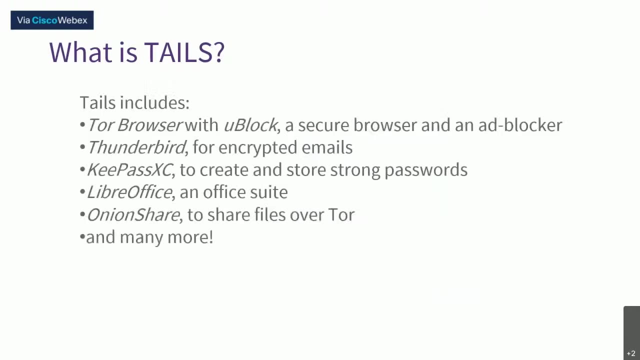 It's got its own storage, and tails is a digital security toolbox. So whatever tools you want, tails has got it. Okay, We'll see what are the tools and tails comes with the dog browser. It comes with the key pass XC for storing your passwords. 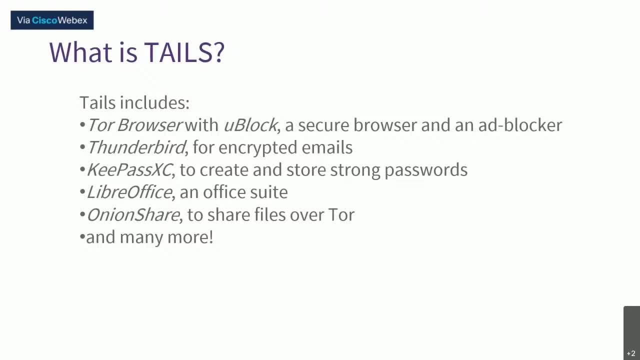 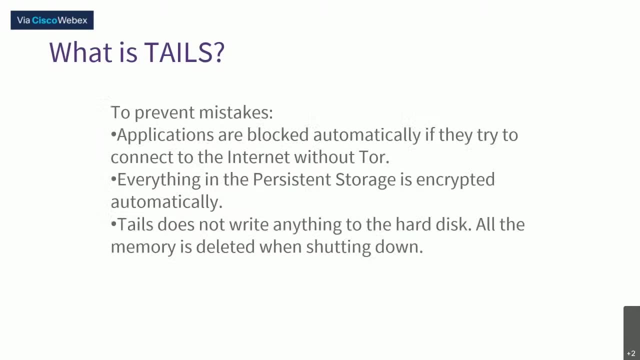 It comes with LibreOffice for you to just like windows office, and it comes with on share and all these features, Okay, And it blocks the applications If it does not try to connect without your permission, Without super. so you can't have some um background uh application which, um, without your notice, it is sending data. No, it doesn't. And it has got persistent storage which, again, is encrypted. It is by itself, only It's encrypted. 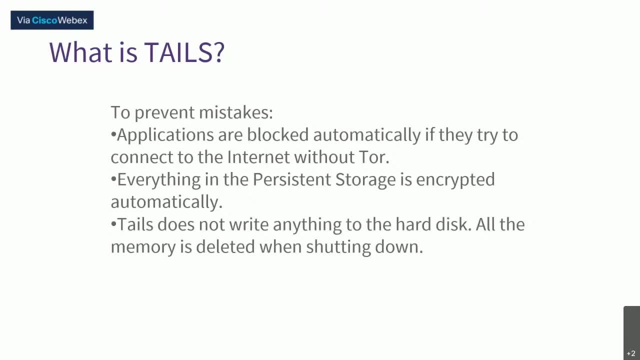 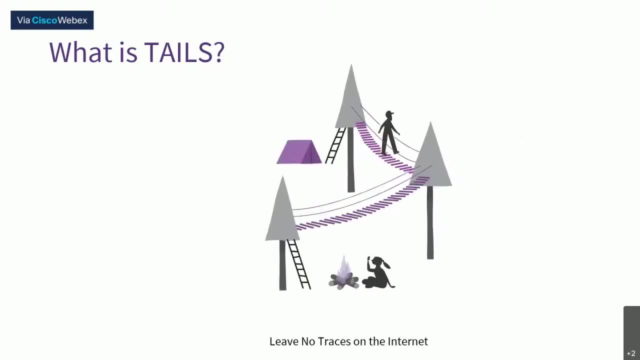 And tails does not write anything to the hard disk. So as soon as you remove this, the memory is gone. Now you may be thinking: remove. What is this? Yes, my dear friends, tails can be installed from, From. 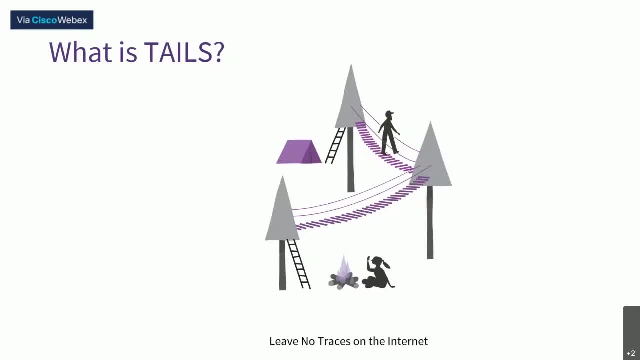 From, From, From From From. It's can be installed from a. so what you do is you have a pen, right, It has got teams in it. You take the pen drive with you. You go. any computer in the world, any computer. It should have a USB drive. 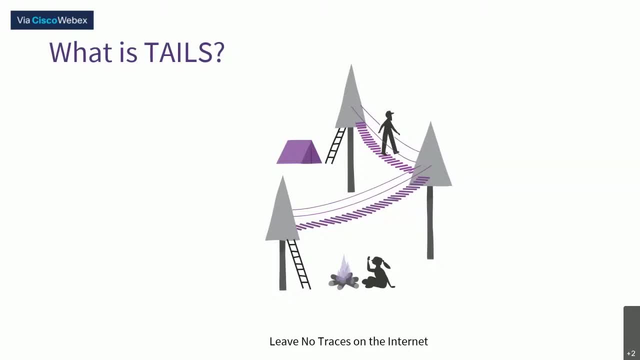 Put the USB right, Restart the computer, boot from the USB drive, Simple operating system starts. so far, isn't it? You don't have to install the operating system anywhere. You don't have to download the operating system operating system in the computer that you want to use tails. no, you just need to have the usb drive. 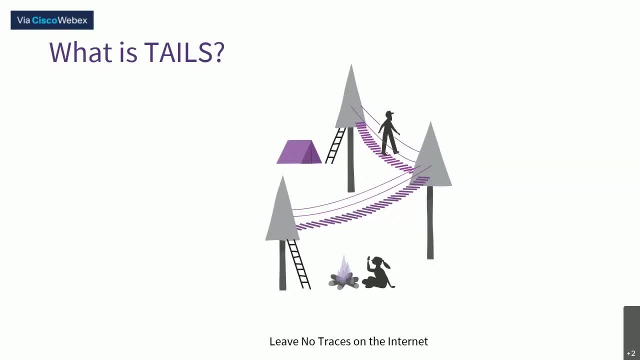 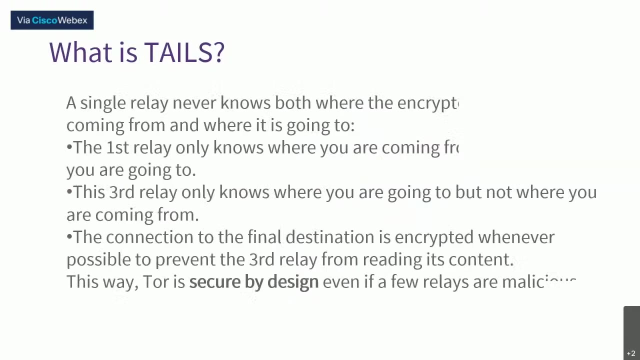 with you. take the usb drive wherever you want. connect it to the computer. now you may ask which computer it can be: any computer. connect it to any computer and tails will start working, and tails leaves no traces or internet. okay, so, uh, now look at this. tails, uh, the the benefit of tails is it? 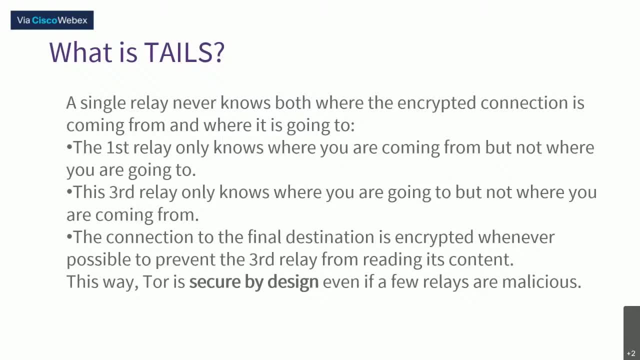 does not connect from a to b directly. no, it doesn't go that way. it is a to c, c to d, d to e, e to f. so it goes that way, through a different route and finally goes to b. a to b direct connection does not happen, so therefore, 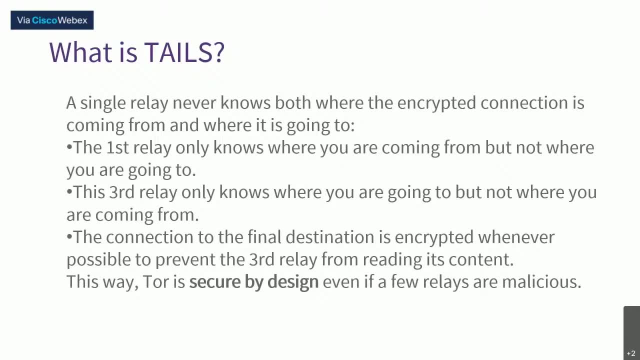 tails. the best part about tails is it is secure by design. i repeat, it is secure by design. so we have to use tails, not because we are using one operating system that is of linux flavor, but it is linux flavor which is secure by design. okay, so this is how it is now. 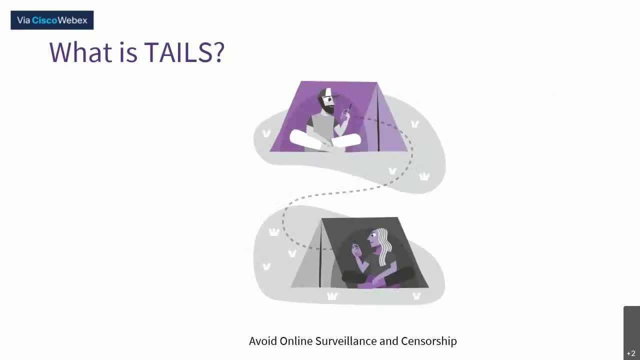 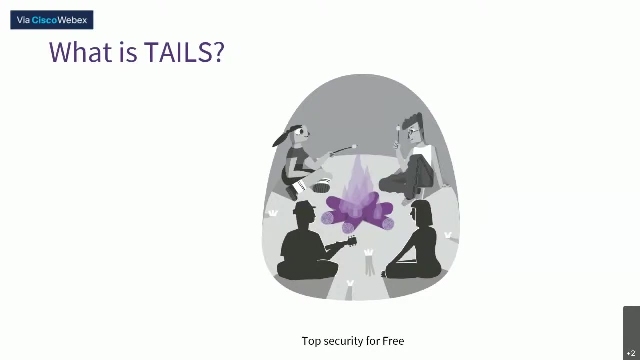 coming to the next one. so you can avoid online uh surveillance and uh, And you can censorship, because you can mask your not only IP address, you can also mask your MAC address also, And the best part is, TAILS is free. So that is how it is. And next one: 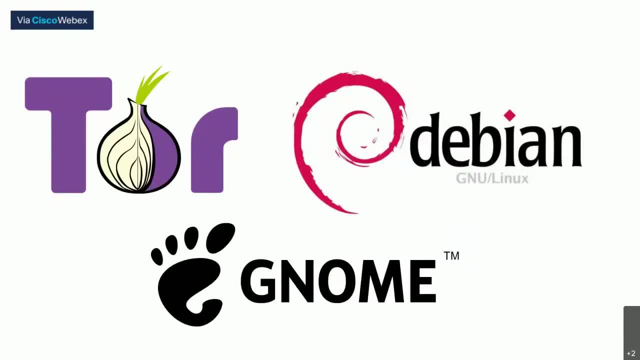 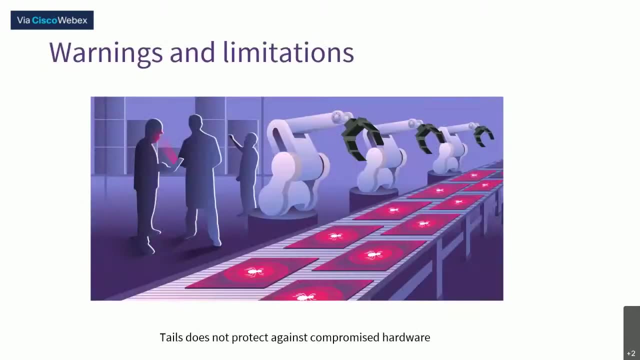 TAILS. if you ask me, what exactly is it? TAILS is basically Tor, with the TBN GNU-based Linux, and the front end is GNO. Okay, So this is how it is. So this is how TAILS work, And somebody is asking whether it can be used for mobile phone. This is a desktop operating system which is basically done for that. 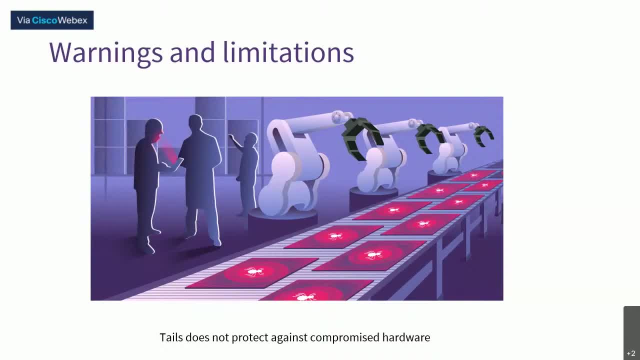 But of course you can use certain tweaks and you can make it work on a mobile phone, But it is not as simple as that. It is not as simple as how you can directly install it on a mobile phone and use it. This is basically a desktop operating system. Okay, So there is TAILS. 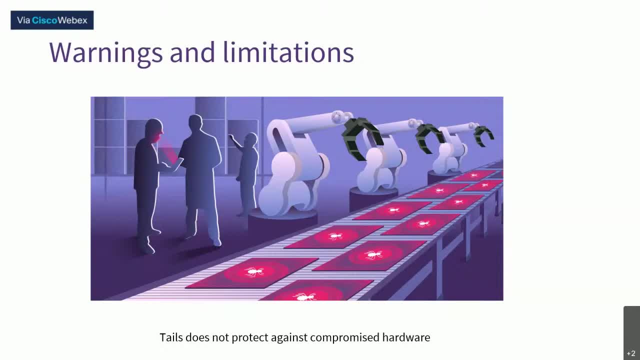 So there are other flavors also for the mobile operating system, So I will come to it in the end of the time. Okay, Once let me explain TAILS And then from there we will see what are the Android operating options for TAILS. 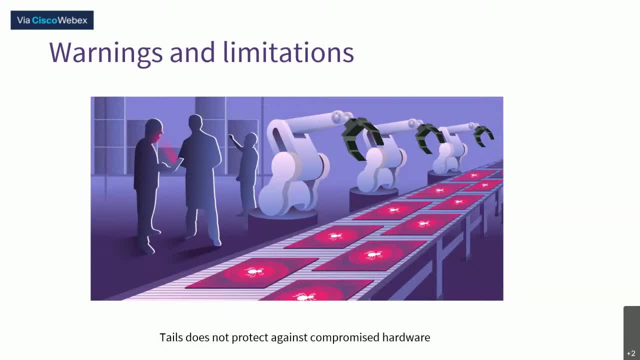 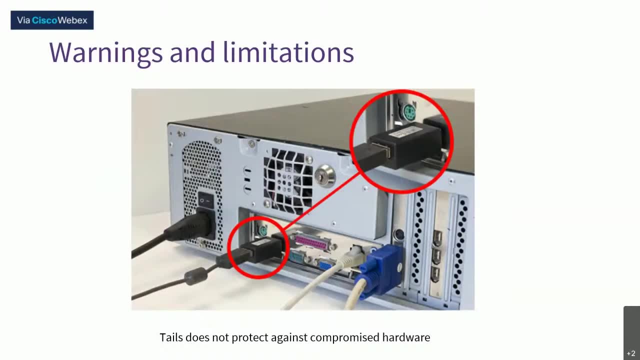 So the limitations of TAILS is if the computer that you are putting the USB drive, If that is compromised, then you can't do anything Because there can be a key logger in that particular computer. It can be a software key logger or a hardware key logger. Software key logger: yeah, it won't function because it will have. what is that your operating system of Windows or that doesn't work for the key logger? 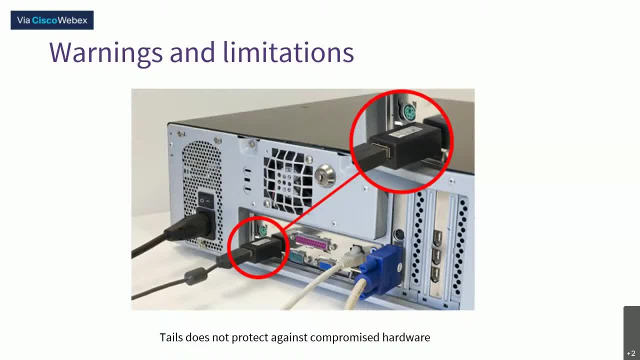 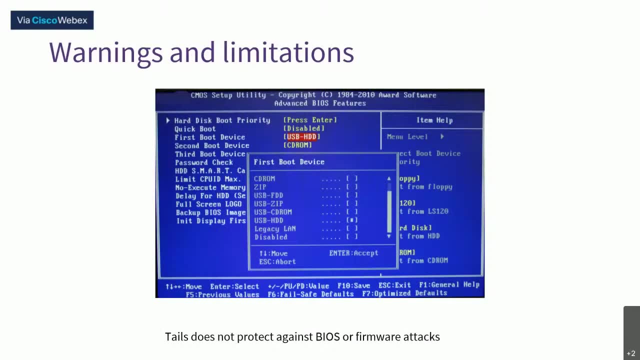 But if it's a hardware key logger, then it's a problem. Or if there is the BIOS, the BIOS is compromised, then you really cannot do anything, Because TAILS does not protect you from BIOS and it does not protect you from other firmware attacks. Okay, 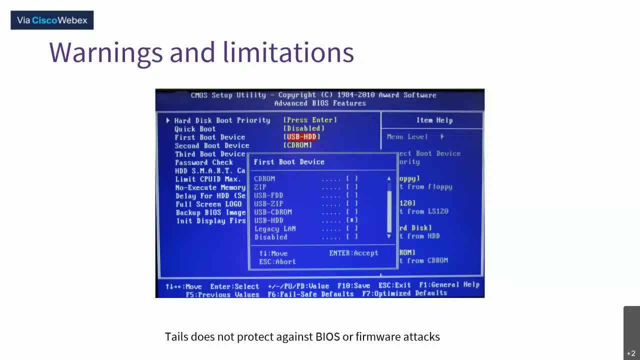 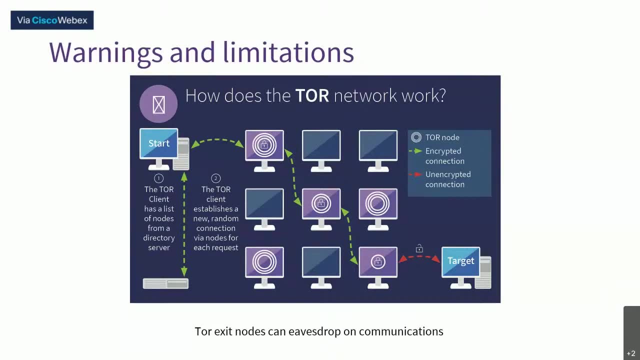 So now coming to the next one is: how does the Tor network work? So I told you, the Tor network is basically working where from A to B the connection does not happen, but it goes from A to C, C to B, D to E and finally to B. 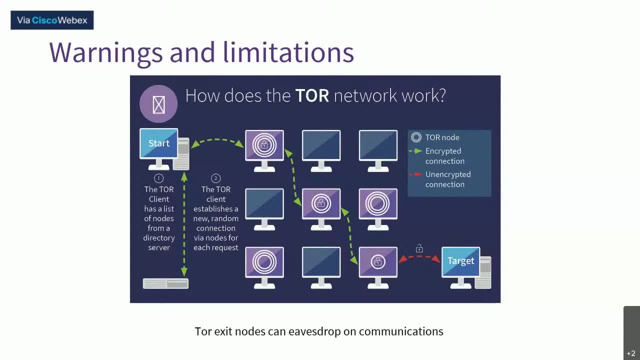 But if you see the connection, what basically happens is from A to C, C to D, D to E. it is encrypted. It is a Tor based connection. But from that last node to B the connection is not encrypted, Because anything that is on Tor network there it becomes encrypted. But if the server that you are accessing, if you're trying to access a server, and it is not on Tor network, then it won't be encrypted. 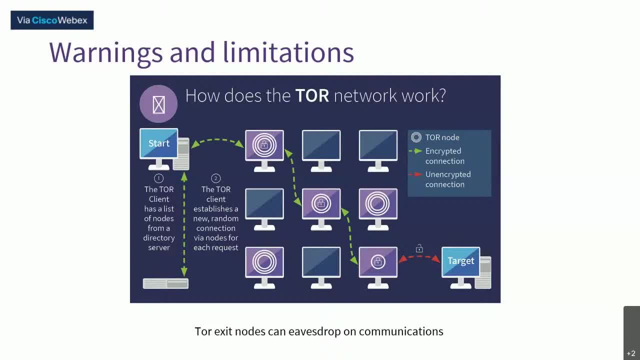 Okay. Yes, it can be HTTPS. It can be Okay, But it is not. if it is not on a Tor network, then it won't be Tor encrypted. Please remember: it won't be Tor encrypted. It can be HTTPS if it is HTTPS, not otherwise. 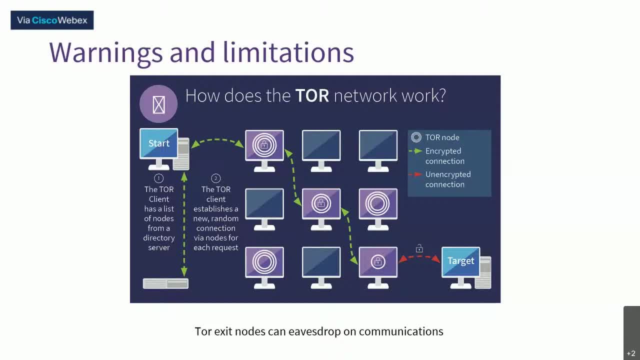 So, if you are going to ask me the question, if you're going to ask me the question whether- whether that Tor or TAILS- is end-to-end encrypted, it is not end-to-end encrypted because the last, the last relay, I should say that is not end-to-end Okay. So this is how it is Now for the ones who are interested. if you are, if you're looking for a similar operating system for Android- I'm not talking about TAILS, because you asked me if TAILS can be for Android, but there is one operating system which is called as the Guardian ROM. Okay, 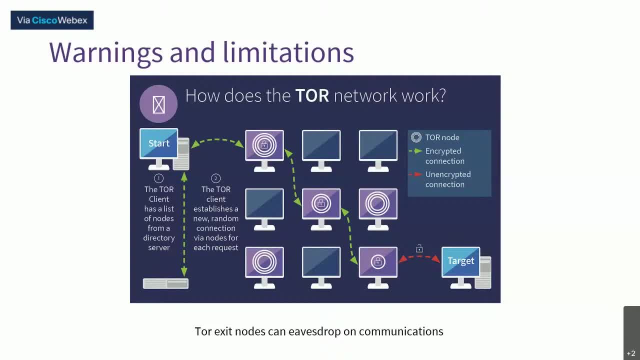 It is a secure version of Android, Okay. It does not provide the anonymity and leave no trace- mentality like TAILS, So it's not that good, but it is good. Okay. Now the new mobile TAILS which will be coming soon. 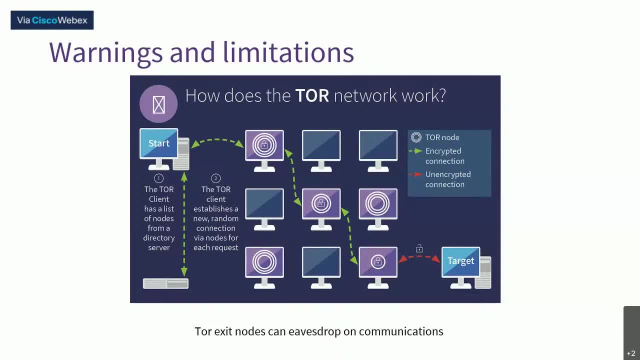 I'm not talking about the desktop based, which you're tweaking and using for the mobile, but the new one, the TAILS, which is going to come for the mobile phone. then that will have many features of Guardian And also many features of the desktop based TAILS. So very, very shortly we'll have the mobile one also. but if your question is very specific, then use this for mobile. not very easy, Okay. 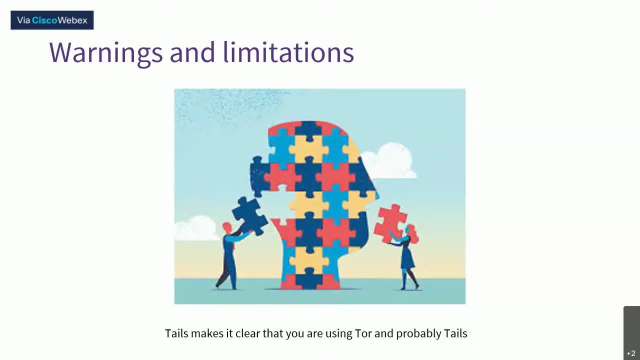 So the next one is TAILS makes it clear that you are using TOR and probably TAILS to the ISP. That is one problem. Okay, Your internet service provider gets to know that you are using TOR and you're using TAILS, So this is one thing very difficult to avoid. 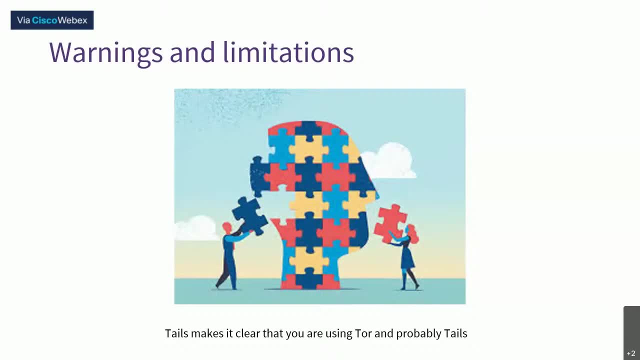 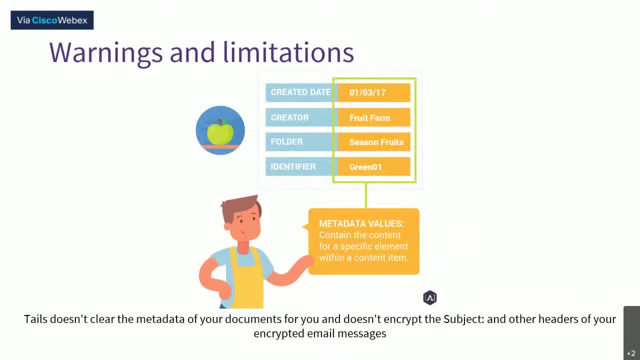 There are means of avoiding that also. I didn't explain it in some time, but they get to know- And again I told you this point that time, even if the data is encrypted, the metadata will not be encrypted. Therefore, TAILS does not clear the metadata, So the metadata is going to stay and this can put you in trouble. Okay. 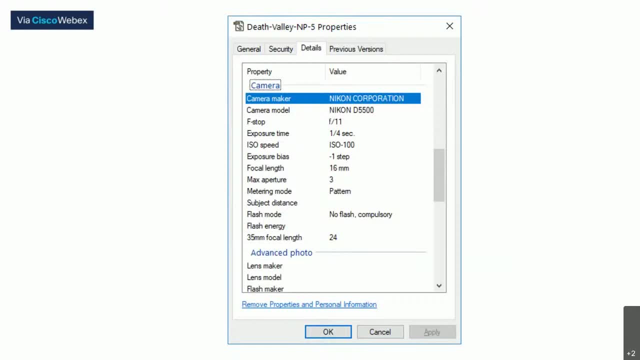 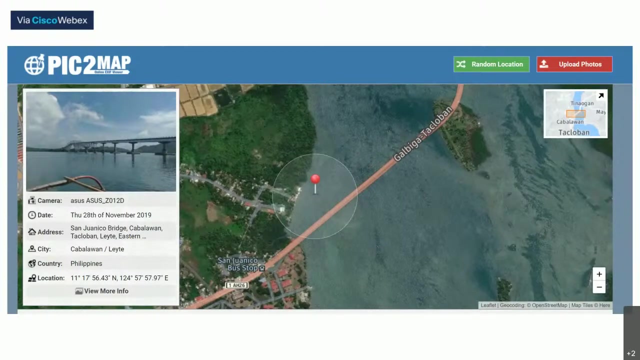 And so I told you about metadata that then on the photo, if you right click and see properties, you can see a lot of details like this Camera use, ISO focal length and all that. Yes, that can be seen. Now, look at this. You can all go to this website called speak2mapcom and you can upload any photo. It will show you all the metadata of that. photo Number one. 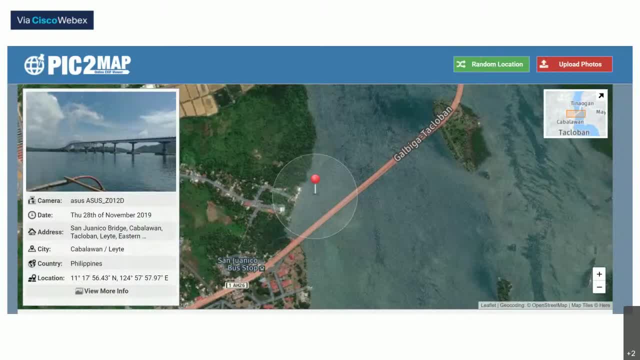 And number two is: it will also show you where the photo was taken, if the geolocation was anything. Now look at this. This particular photo was taken on 28th of November in Kerala 1,, that is, on the Juvanico bridge. 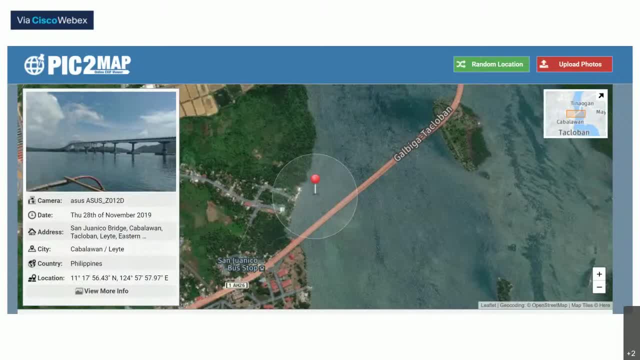 Okay, So in the Philippines, this is where it was taken, So it will show you the exact location where the photo was taken, So you can- you can- try that speak2mapcom. Okay, coming to the next part, just a second. 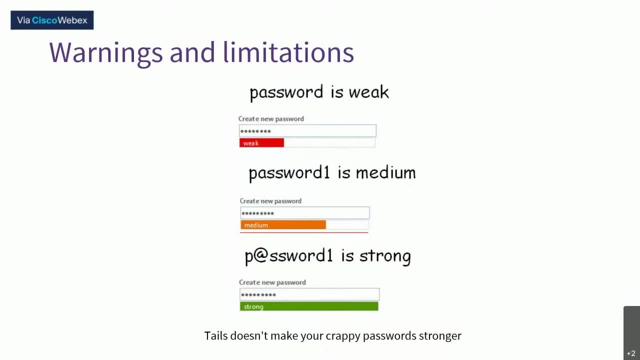 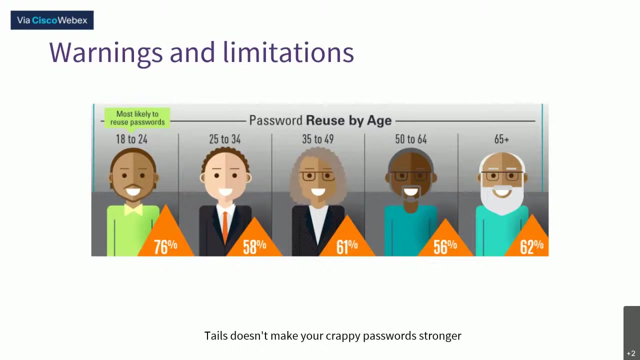 So TAILS will also not protect you. TAILS will not protect you from weak passwords. If you're using a crappy password. it will not protect you, So you have to be very careful about that. in the sense, it will not make your password stronger. your password- crappy password- is going to be crappy only. So this is how people use the same password. See, this is 1 mistake all of us do. What we do is we use the same password for Gmail, same for Facebook, same for others also. 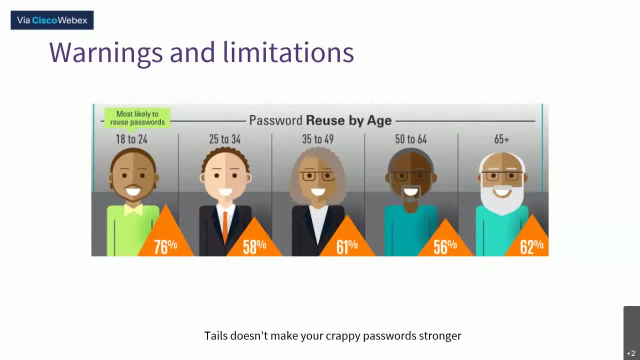 So this is how people reuse the passwords: 58% from 35 to 34, 61% from 35 to 49 and 65 and above. 62% are using this TAILS And we have to be very careful about that. 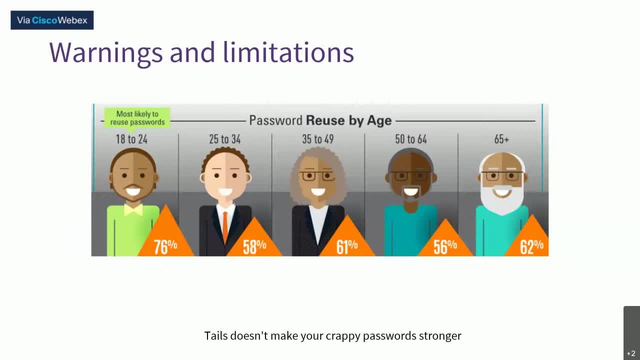 Okay, are using the same password. so what will happen is if uh you use one password for the same uh different uh site, then if one site gets hacked, the hacker can use that same login credentials for other sites also. yes, i know it is difficult for you to remember passwords. that's why i said. 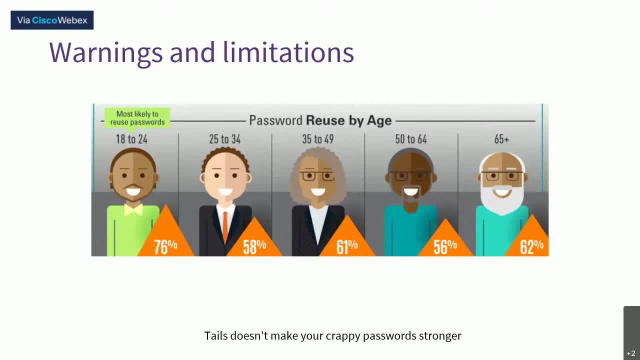 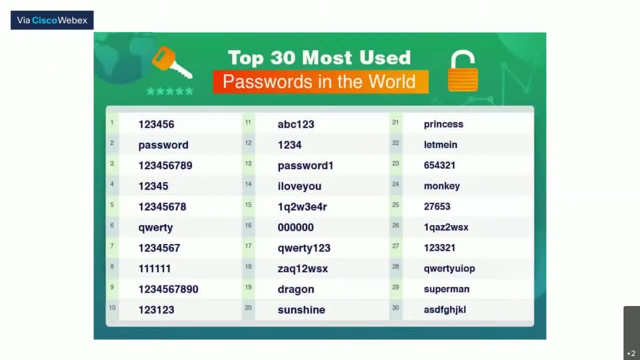 use the password manager like that: keep pass which i told you, which is there in that. that is super okay, and these are the 30 most used passwords in the world in 2020: 30 most used passwords. so have a look if your password is there, in that order. 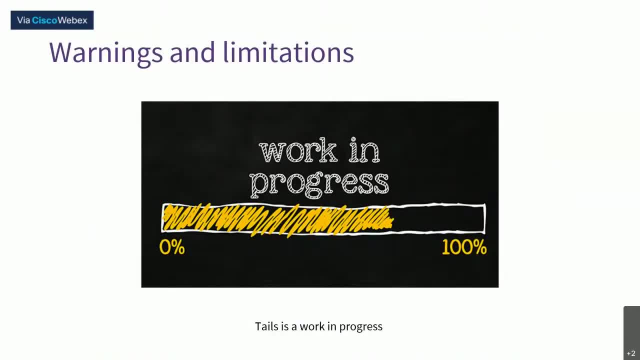 see now, uh tails again. as i said, see now the mobile tails is going to come out and all that. so it is a work in progress. so, uh, they are. they are constantly upgrading and uh, the newer ones are on and on coming, the newer features are coming. so you have to be uh very sure. 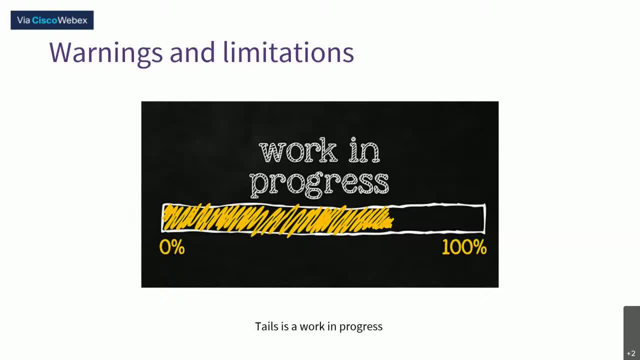 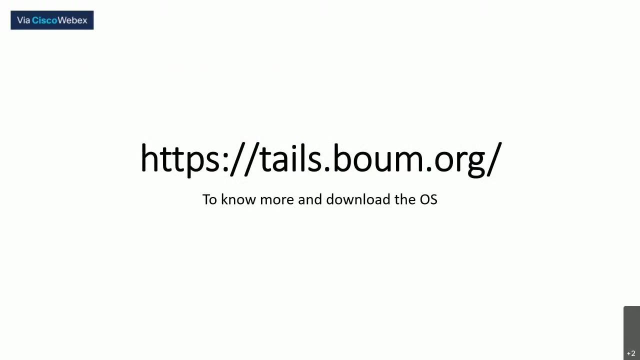 that, uh, whatever you are doing right now on tails is not a final product, so it is a work in pro progress. but compared to many of the things, this tails is uh fantastic and how to download tails it is, as i said, number one. it is free. so go to tails. dot b-o-u-m, dot o-r-g. 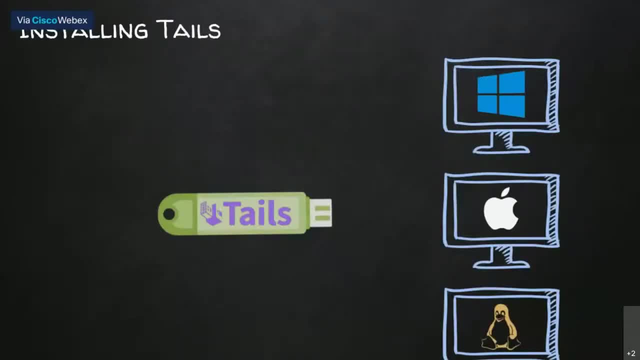 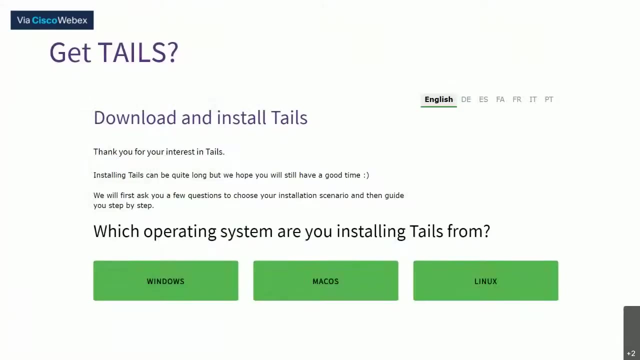 okay, go to this website and you can download tails for windows, mac or linux. it can be for anything. you can use tails or any system. number one: desktops. okay, uh, laptops and desktops. so number one. number two: how to download. go to the download page and you can download it for windows, mac or linux, but i don't recommend. 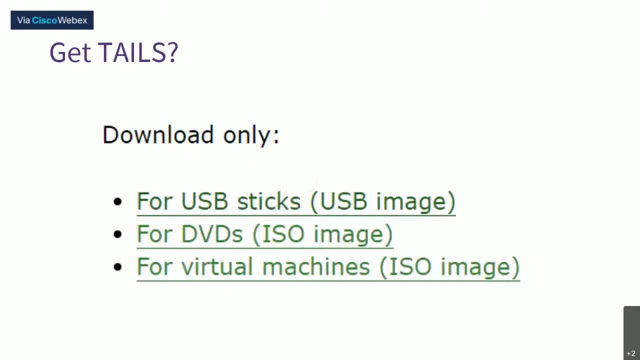 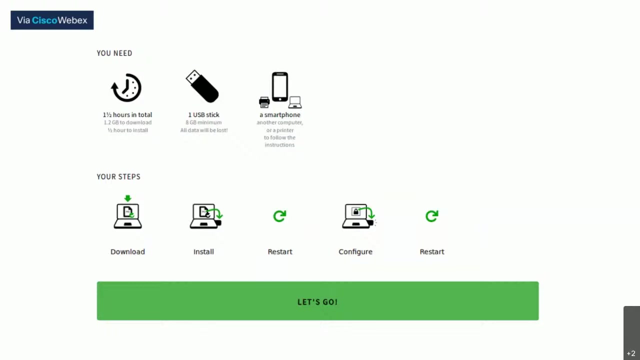 any of these, because i want you to download tails for usb sticks, because we will be using a usb stick, so it should be minimum 8 gb usb you can take. in this case of mine, it is a 64 gb, so you take a usb stick and you download the usb stick tails, which is about 1.2 gb. okay, so get a 8. 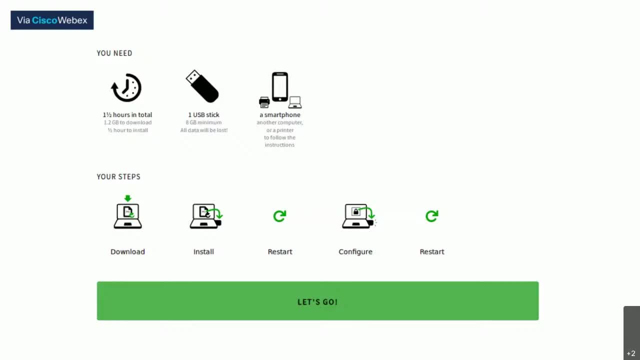 gb minimum usb stick and use a. you need a smartphone just to follow the instructions, okay, so once you download it, you need to install it into the pendrive. it is not simply copy and paste into the pendrive. what you need to do, i tell you and then just restart the system, put the pendrive. 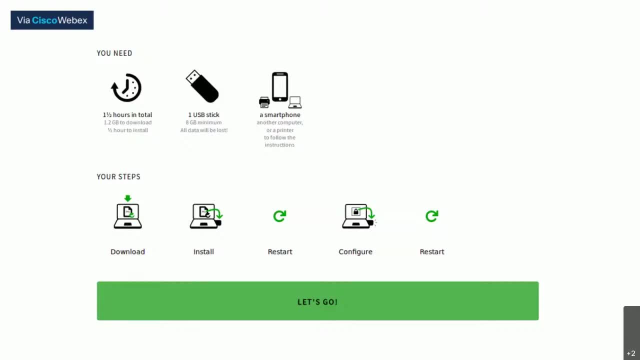 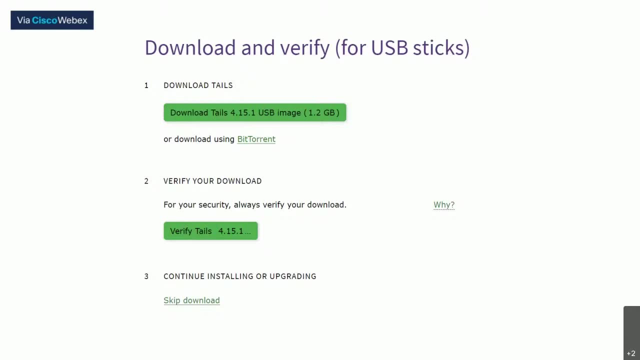 desktop or wherever you want, and then boot, boot from the usb, and then it starts loading beautifully. so three steps: first is download the 1.2 gb. second, one very important step is verify, because tails will be downloading it from different servers, different servers that are mirrored. what if one of the servers is compromised? you don't know. so you need to make sure that. 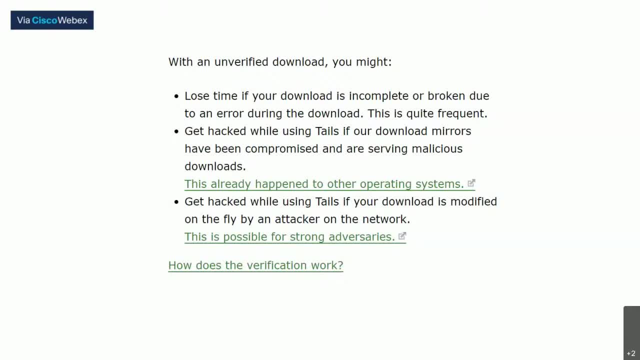 one if the server is compromised. second, if somebody has hacked it. or the third one is: uh, while you are downloading, uh, if the download is incomplete or a broken download, you're going to waste your time. therefore, all you need to do is the second part. there is an option. 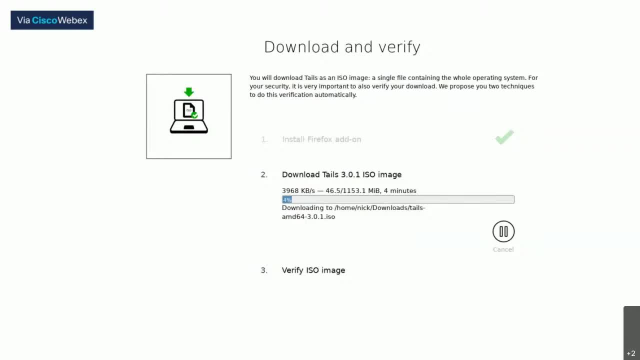 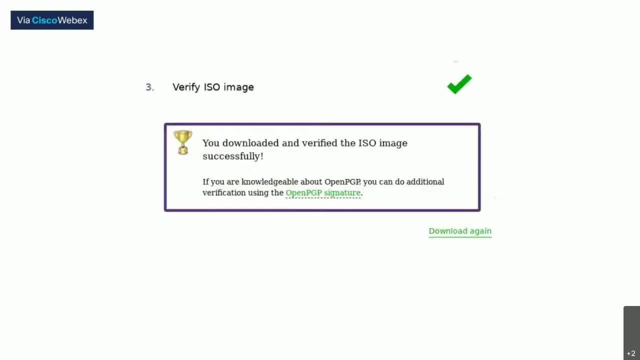 called as verify the download. so just click on that. it will install one browser extension and it will verify your download. if your download is verified, it will say you downloaded a verified iso unit successfully. once that is done, i told you, the third step is you need to take the 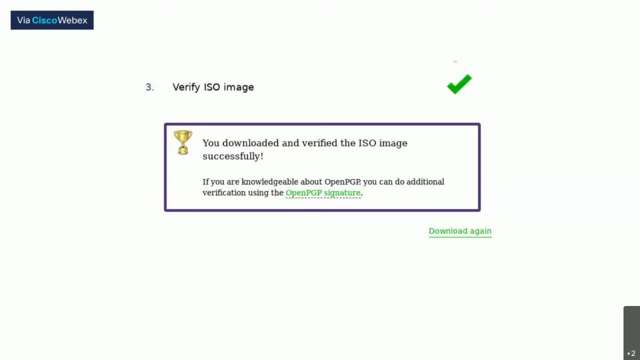 files from the desktop where you have downloaded and put it into the usb. but directly you can't put it into the usb, because you should make that usb as a live usb because why you are going to boot from the usb? so because you are going to boot from the usb, or if you are going to 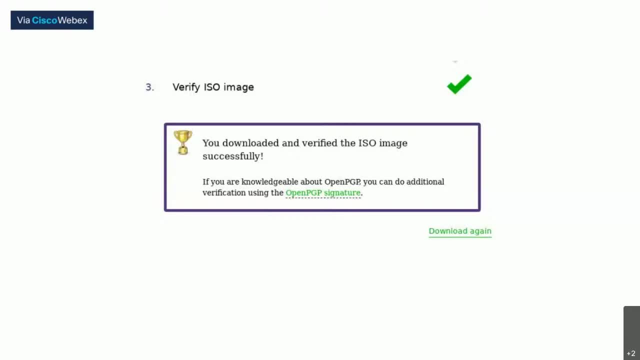 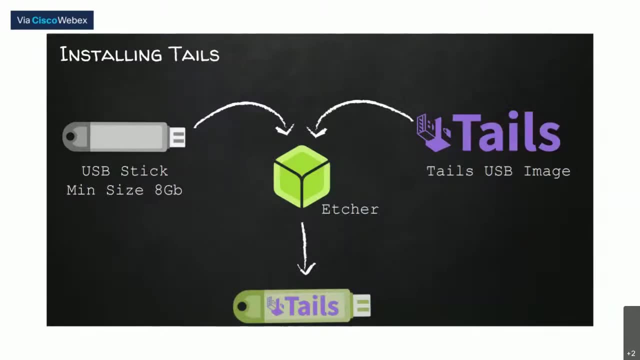 boot from a dvd. you are going to make it live dvd or live usb. for that there is a free software that is available, which is called as etcher. i repeat, the software is called as etcher. so all you need to do is take the usb, connect it to the computer, open etcher and select the usb. 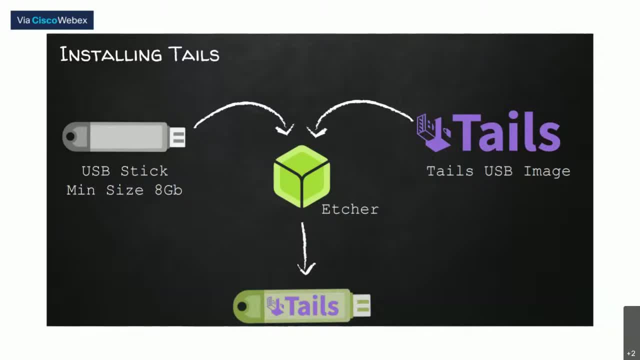 put the downloaded 1.2 gb file into the etcher within 10 or 20 seconds. etcher will make your usb into live usb- simple, nothing else to do, but you need to remember: all the contents that were there in your usb will be formatted. therefore, you have to ensure that your usb, all the contents are. 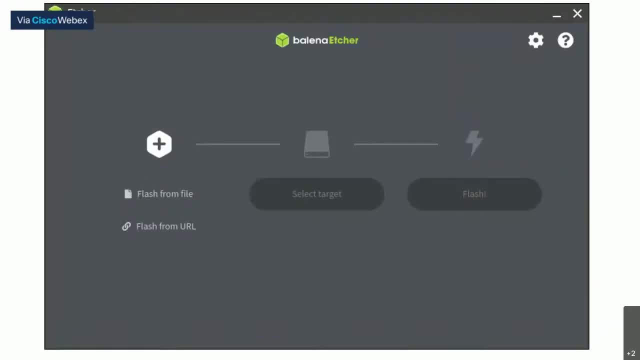 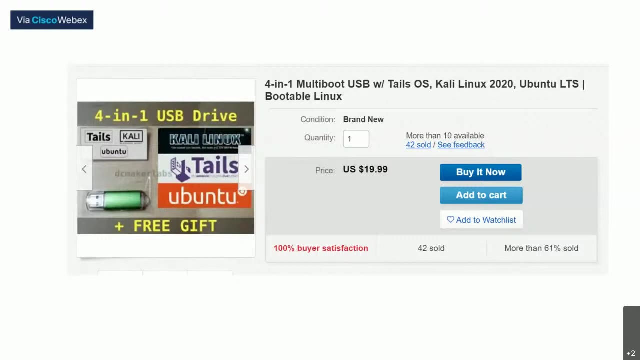 once before you use it. okay, so this is how it looks: select the file and select the target- the usb- and just flash it. the usb becomes live usb. so, or if you are very diff, uh finding it very difficult to do it, then you can go to uh ebay or any of the websites and you can download one. four: 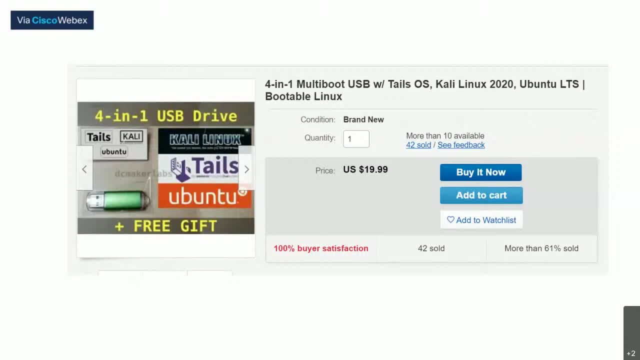 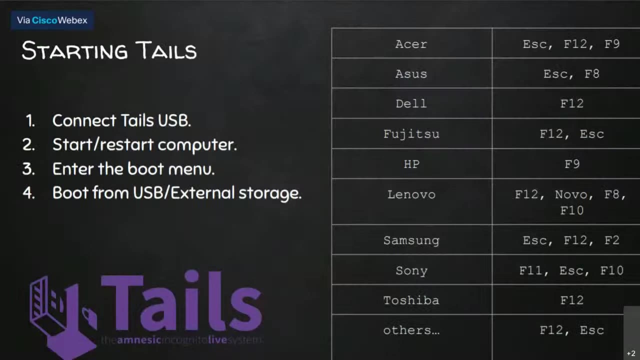 in one usb drive which comes with pre-installed tapes. but why would you pay 20 dollars for something like that, where you can just buy one pen drive and uh download etcher and download? yeah, it's costly, so you can. you can just do it, uh, without any any problem. okay, and once you install, you need to boot. 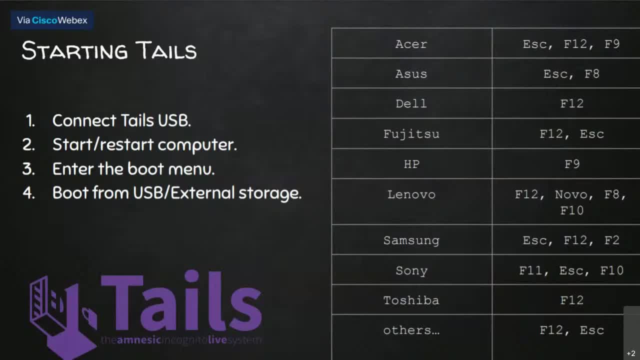 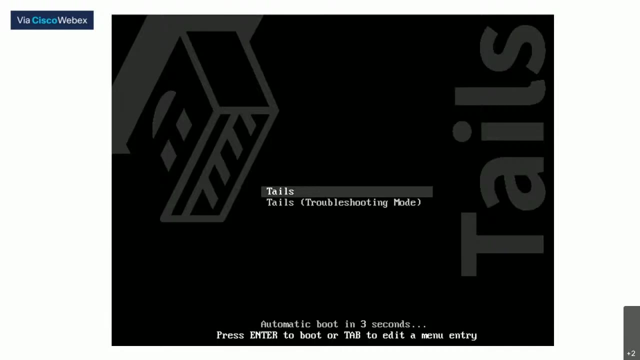 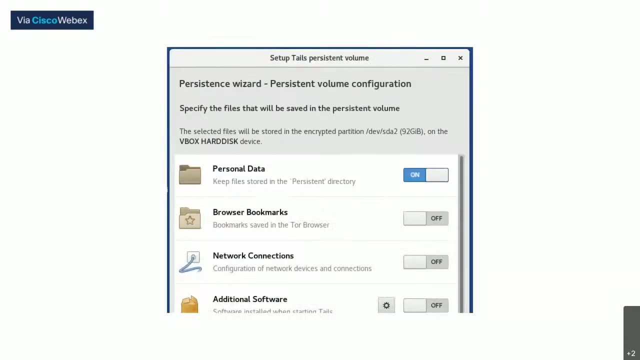 so there are different. uh, you can press escape to go to boot mode f2, lf2, depending upon the systems. you can see how to restart and boot menu in the boot menu. select usb. simple tails will start. as simple as that. okay, so tail will start. once tail starts, select the language, keyboard format and all that. now there is an. 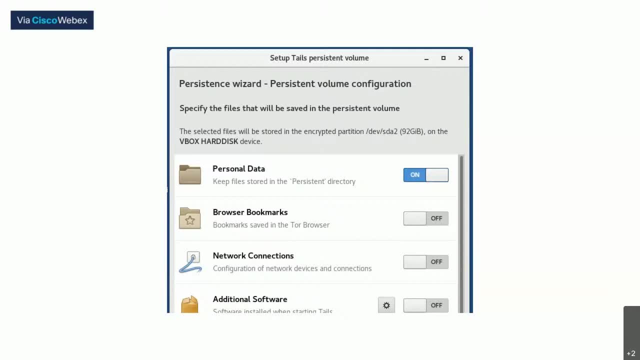 option that i told you know: persistent storage, persistent storage. what we need to do is, i told you, once you put the usb into the keyboard, into the laptop or the desktop, the hard drive of the laptop or desktop will never be accessed, never. so any files you download while you are using tails. 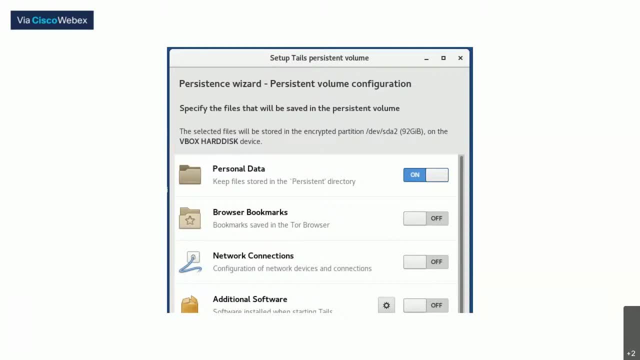 it will never get stored in the hard drive. if you want to save that file, you need to store it in the pen drive only, and that pen drive data where you're going to store it, the area where you're going to store it, is called as persistent storage. and remember, my dear friends. 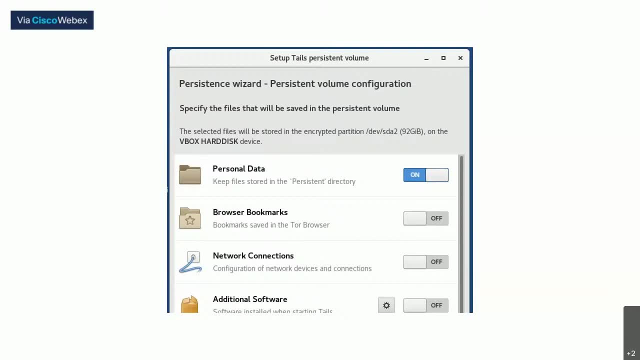 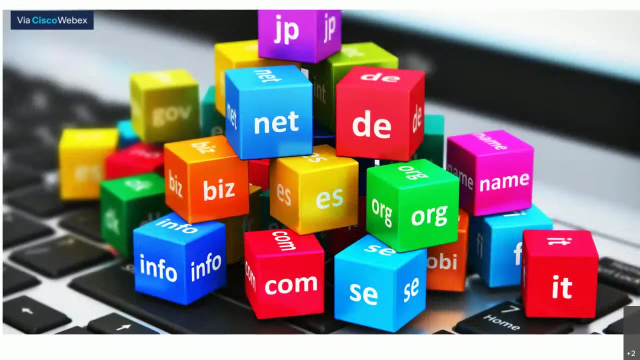 persistent storage is encrypted and persistent storage can be password protected. okay, so this is why you need to make sure that persistent storage is there. so more persistent storage. if you want, make sure that your pen drive is 64 gb, 128 gb, things like linux, uh, you can check the graphical user interface and you know, you know that there. 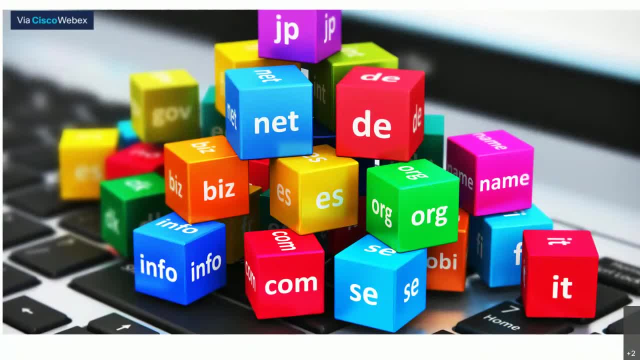 are about thousand four hundred top level domains. now, what is top level domains? dot info, dot com, dot org, dot net, dot biz, like that thousand four hundred? are there newer ones have come? dot shop, and all that. now, okay, how to find the boot menu in the laptop? it is simple, yeah. you uh just have to. 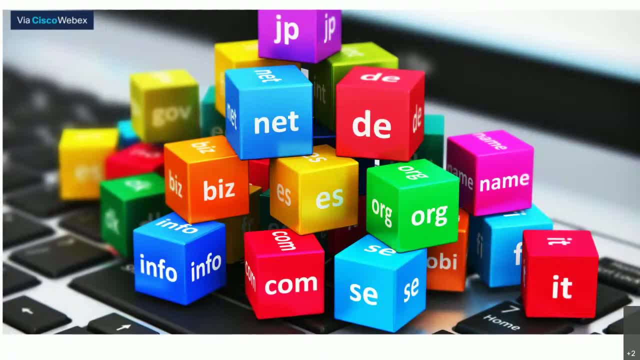 uh. type for the name of your laptop on your on google and type which key to press to go to the boot. so as you start your computer you have to go on pressing that key. sometimes it will be f12. go on pressing f12 four or five times it will go to a black screen and the boot menu will come there you. 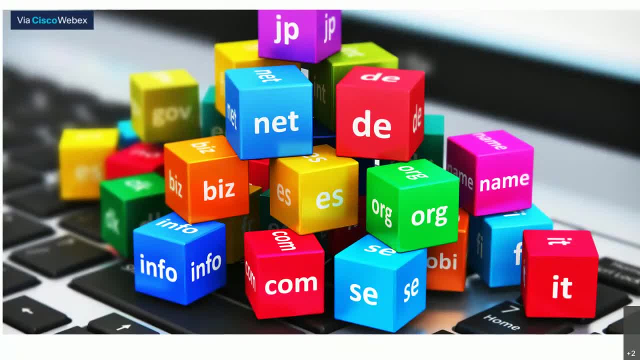 need to select boot from. usually it will be boot from hard disk, because your hard disk has got the operating system. just change that to usb. so simple step. if you are finding it difficult, anyways, i will send you the ppt on how to boot from usb. all right, now you, uh, you can see this. uh, there are. 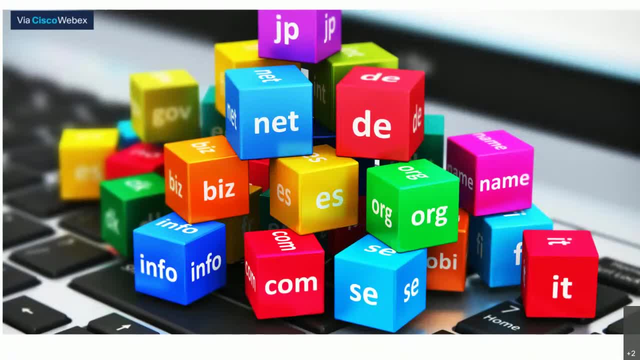 different types of uh top level domain names, tld, we call it. now you're going to use top, you're going to use star browser. now i told you tor, if it is on tor network, if it is on tor network, then what you need to do is: uh, it will be ended to end encrypted. if 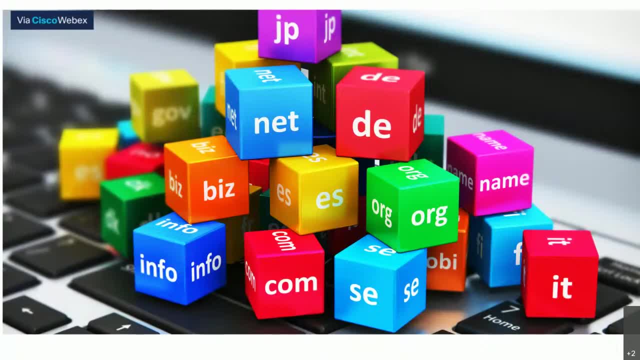 it is on tor network. if you're not on tor network, that last relay will be not encrypted. now my simple question to all of you is- i don't know how many of you have used this- if you have used tor network, if a website is on tor network, what will be the extension? whether it will be dot. 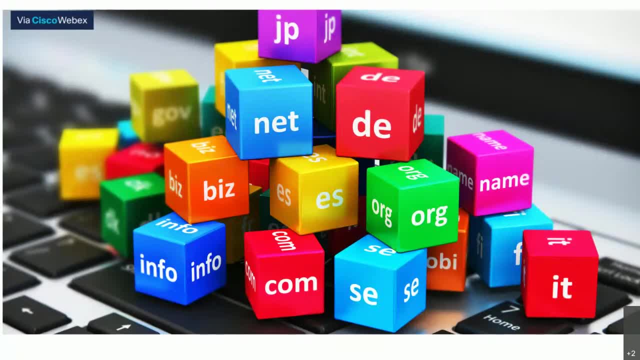 com or dot info or dot org. what is the extension of a tor network website? please answer, dot tor, dot onion, absolutely, absolutely onion is the answer. you. you will have like wwwgooglecomonion. yes, mr dananjay bandara, you are right. okay, so, uh, this, 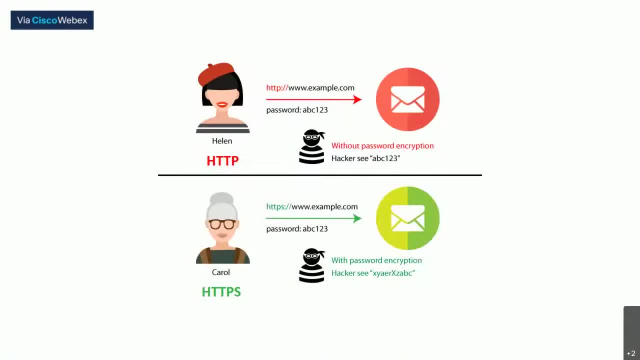 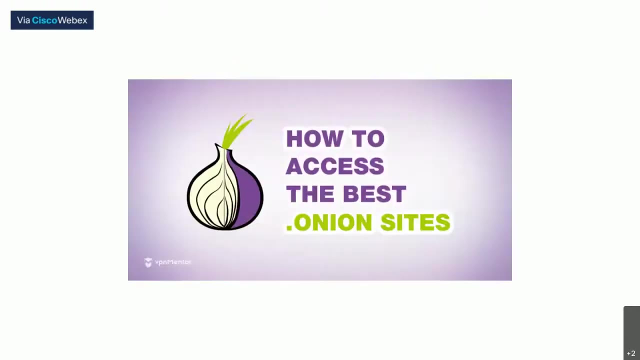 is on the dot onion network and, uh, you know that i told you that http and https. i told you. please make sure that you are always on https, so always https. you need to switch on so that whenever you type a password it cannot see. so how to access dot on your websites? try to open a dot on your. 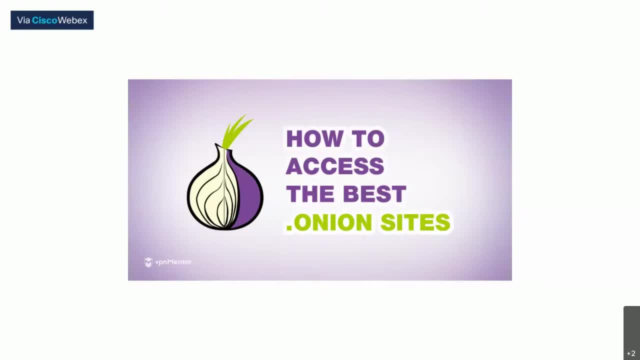 website on google chrome. try to open a dot on your website on mozilla firefox. try to open a dot on your website on internet explorer or the the newest microsoft edge. it will never open. exactly no visible. it will never open. if it, if it is a dot on your website, it will open only on top. 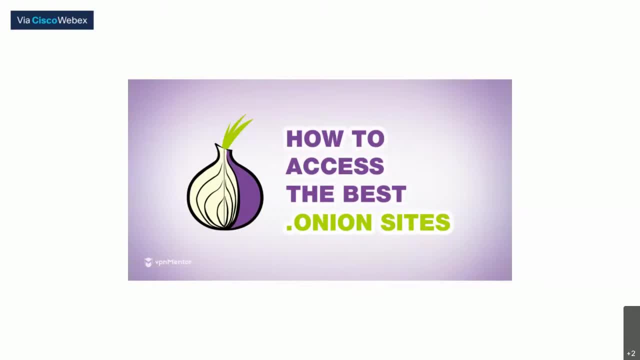 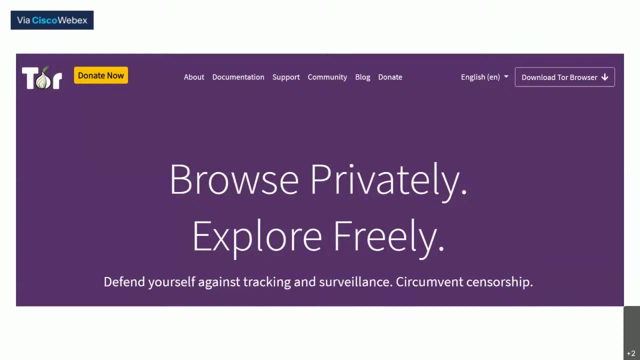 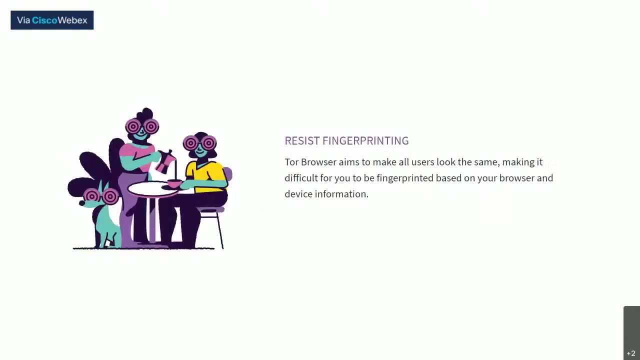 so you need to make sure that you have a top browser, tk. okay, so number one so top browser is to browse the internet privately and explore freely. it will block trackers, it will defend you against surveillance, it will resist the fingerprinting. okay, my question once again to all of you: which? 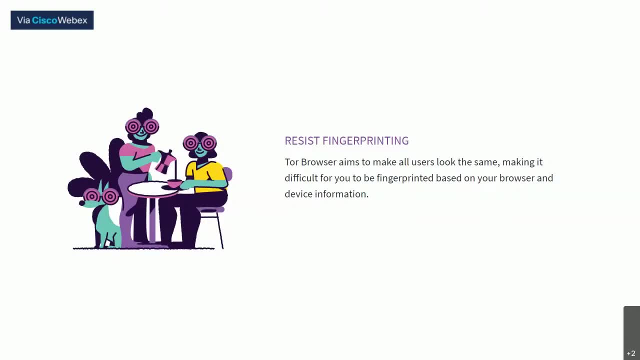 is the website i told you to check if your browser fingerprinting is there or not, how to check whether your browser is secure or not, how to check if a browser is tracking you or not, which is the same i told you that time. cover your tracks, exactly. cover your tracks panoptically cover. 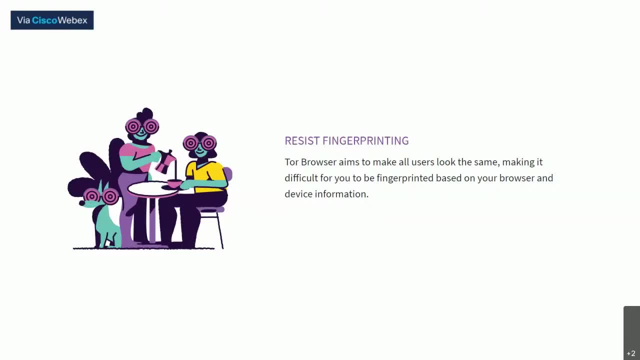 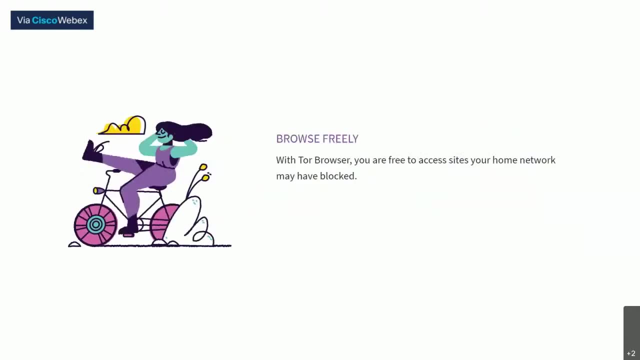 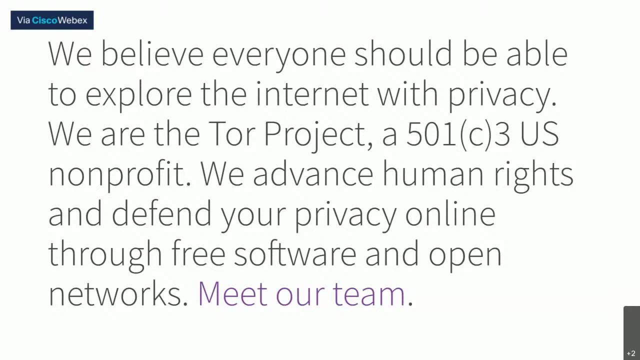 your tracks. absolutely super. okay, so you can register fingerprinting. it has multi-layer of encryption and you can browse freely. and they believe that tor is a not-for-profit and it is only to defend your privacy online through free software and open networks. so this is how tor is and 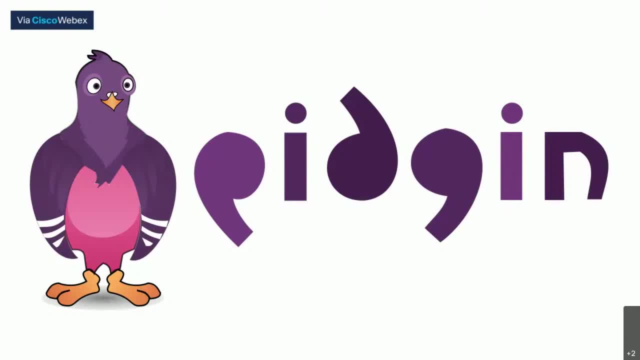 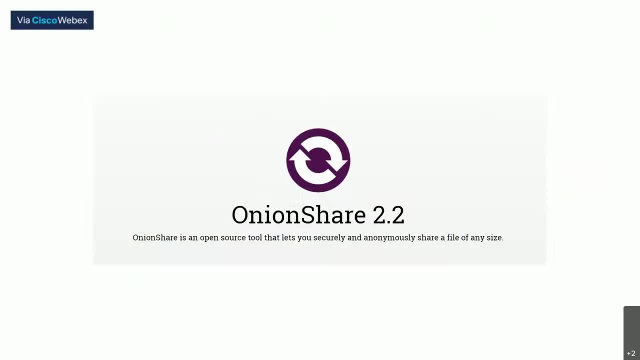 then it lies, the drop down of a tracker. so� or has got this erg nice pidgin. pidgin is a messenger, so different, different messengers you can have it under one. pidgin is there and i'm not not told, sorry. the the tails, then tails has got one superb feature called onion share. now what onion share is? 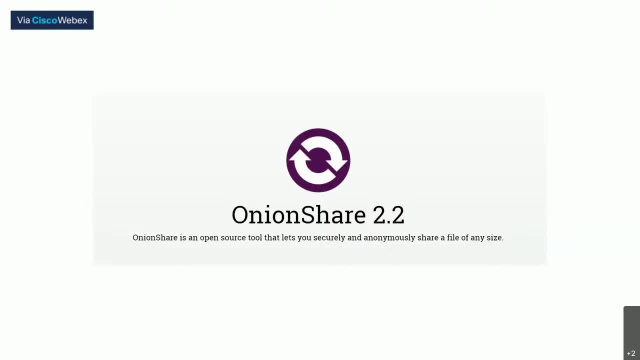 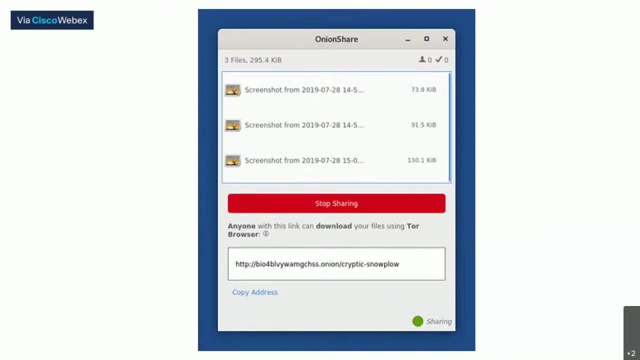 tomorrow somebody will ask me: ah, ask me, sir, please send the ppt. tk. i will send the ppt, but how to send the ppt securely do is i can take the ppt and drop it into onion chip. when i drop it it will create one link. it will create one link which is a dot onion link, which is a private link, a tor link which i can. 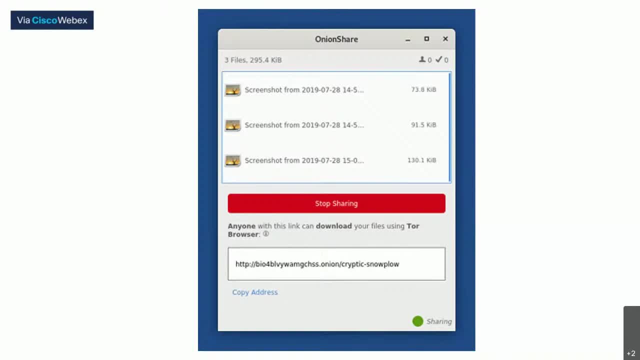 send it to after g. you can click on that using door browser and you can download. look what a safe and secure way of ensuring that- that the file that i'm going to send will be safely reaching after g. so this is how we are going to use it. so onion share is one feature, and then thunderbird is. 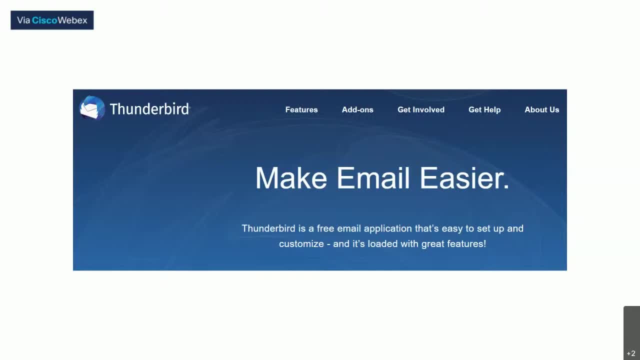 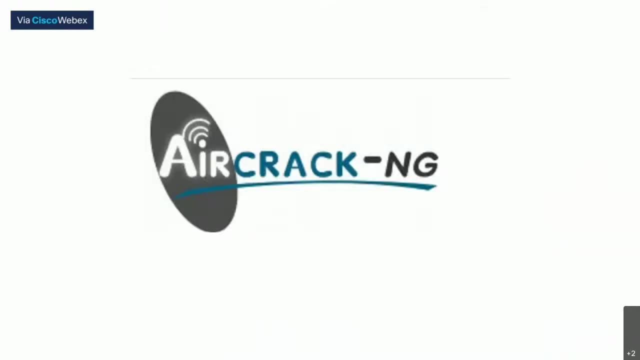 there, which is a secure uh email aggregator, or we can say that as like how you have uh microsoft outlook, so you get that. yeah, garlic clearing is also there, and then thunderbird you can use it. so then there is also aircrack ng for hackers. if any ethical actors are there you want to hack. 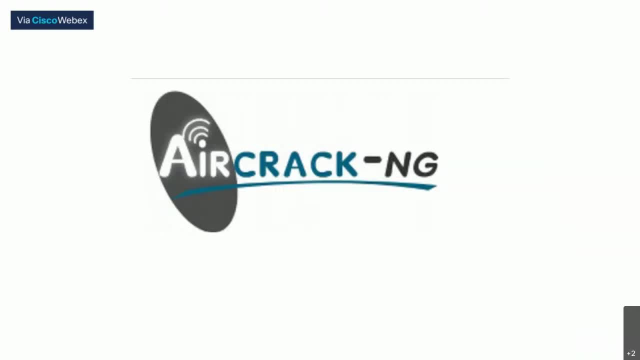 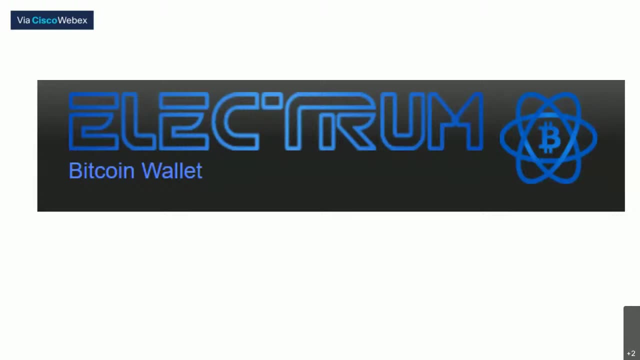 into the wi-fi systems or? uh, you want to check out some details. you can use aircrack ng, then electrum for the rich friends of mine who are there right now, my rich friends who are having bitcoins. okay, so if you're having bitcoins, to make sure that your bitcoin transactions are private, i told you your bitcoin transactions. 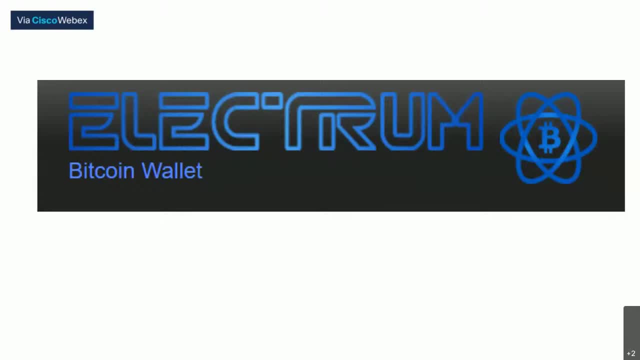 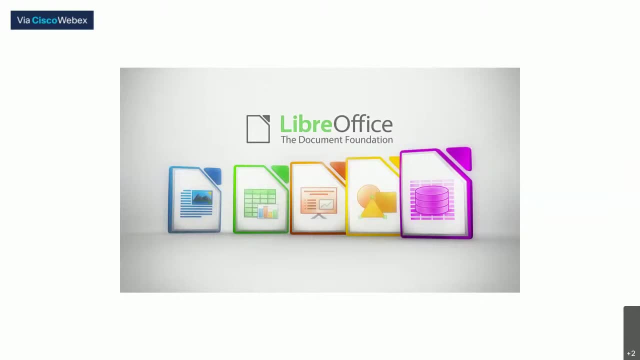 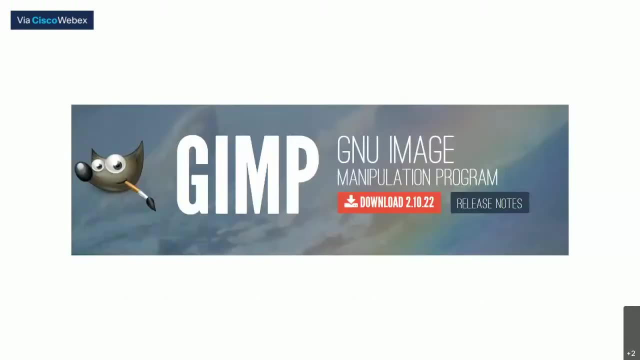 if you have to make it private, if your isp should not get too low, then electrum, the bitcoin wallet that is on tor network, super okay, libre office is there for you to use. uh, open the ppt access excel word and all that gimp is there. if you've got any images, to manipulate, that image like 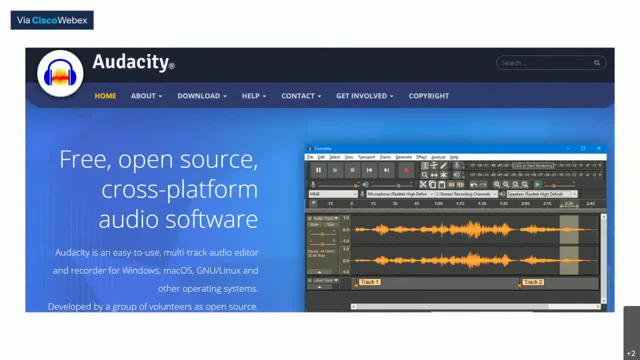 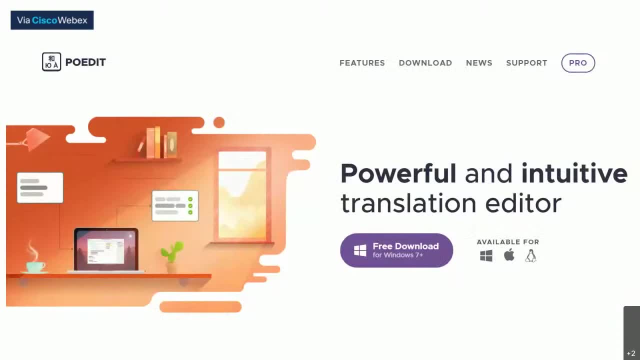 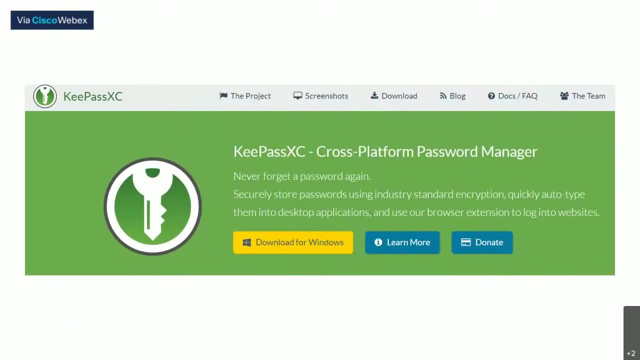 photoshop, then audacity is there for you to, for the sound, voice recording, voice editing and all that, then a very nice point. it is that, uh, quite, it is translating software. then scanner, simple scan, is there, keep a sexy, because this point, somebody asked me the attempt, sir, what if, uh, i can't remember many. 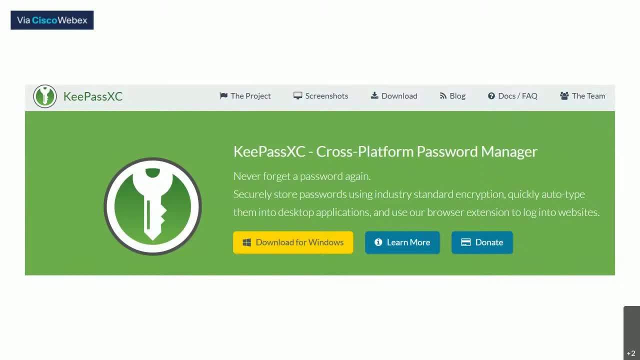 I'll use this. keep us sexy. You'll never forget your passwords again because it is securely going to store your password. You just have to remember 1 password of the key, pass 6, and then it will remember different. It will create different, different, uh, very secure passwords, because when we talk about passwords, password should have 4 features. Number 1,: it should be minimum 14 characters. Number 2,: it should have uppercase, lowercase numbers and symbols. 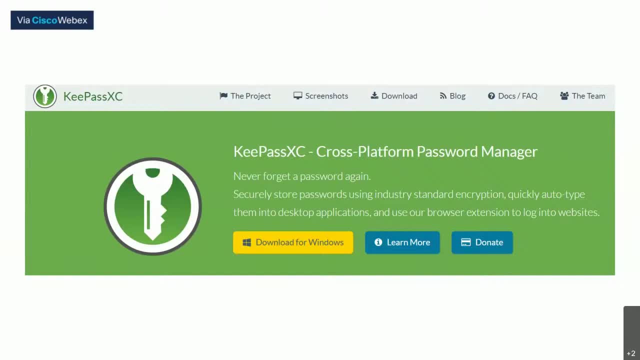 Number 3, you should not reuse that password again and again at different, different places. And number 4, it is better to use a pass of phrases than passwords, So so that, uh, the the dictionary attacks or the rainbow tables will not be having your common passwords that you're using. Therefore, past phrases are better. Now you may ask what is fast phrases? It's simple, Yeah. 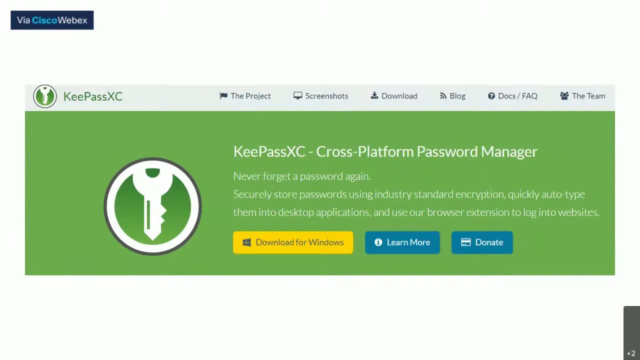 What do you need to do is: uh, like, it's like, and then he's wearing black coat today, Okay, Simple So. and then a, a, n of, and then he's is Wearing W? E, Uh, black, B, L, C, O today. So you come, all these words and make 1 phrase, put some numbers, put some, uh, special characters, uh, and uh, create 1 big pass phrase. 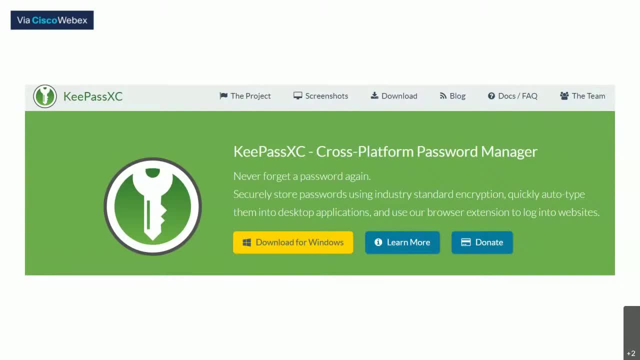 So this is how you can remember what: if our password manager is happy, I can't do anything. But, uh, as I told you, if you're using tails, your password manager will not be happy because, uh, any thing that is coming inside and going out the sandbox. 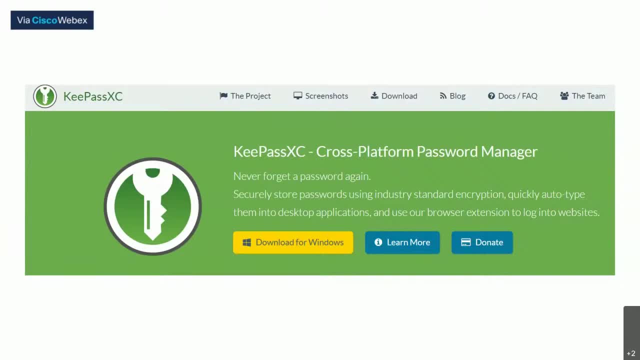 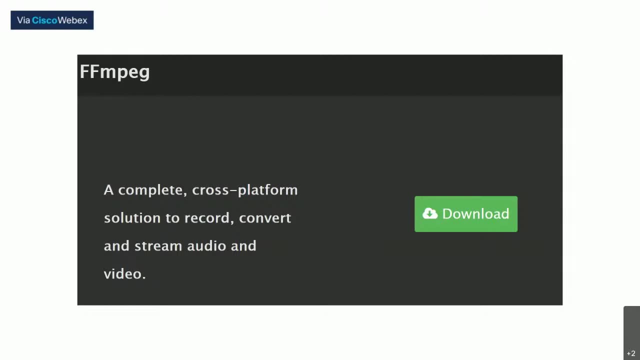 Then you will know that, uh, your tails is, uh, safe and secure. Okay, So then there is a uh uh impact for you to um stream the videos, and uh, audio and video together, And you can also upgrade your teams, because, as newer versions of it, you can upgrade it. 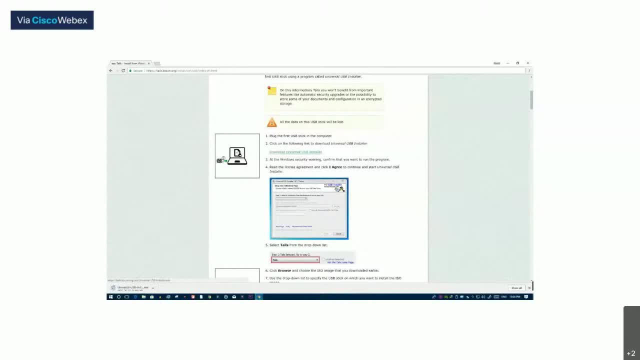 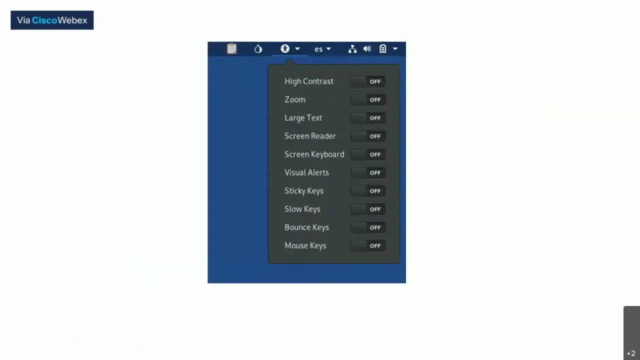 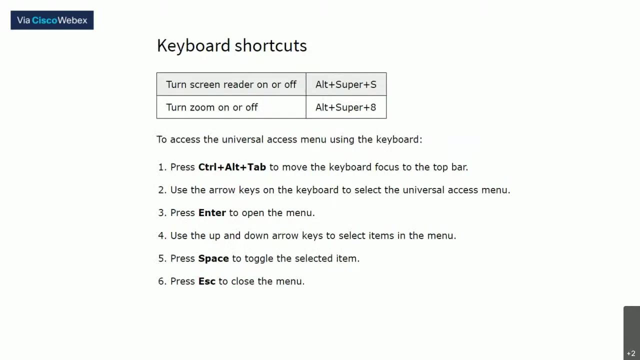 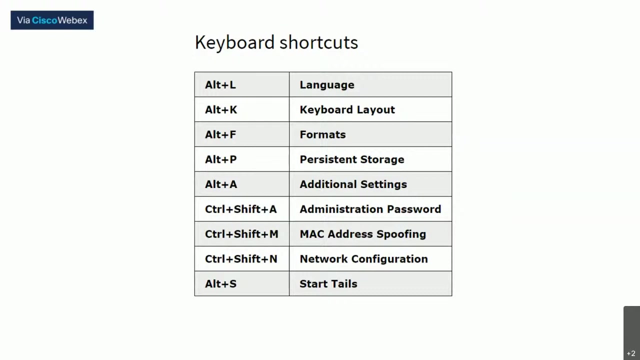 And uh, yeah, uh, after upgrading the next 1, uh, then the deals also has got all these features on the top: uh, contrast, zoom screen, keyboard, sticky keys, bones keys, most keys, all these things are there- and keyboard shortcuts. So look at this. uh, some keyboard shortcuts for you to make your uh tails browsing faster. Anyways, I'm going to give this to you So you can uh check these. uh, uh, this one. 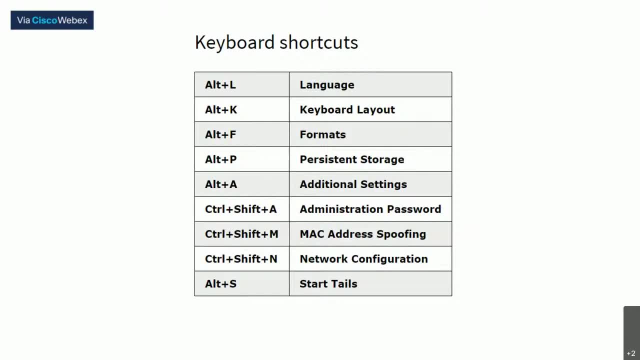 Okay, So, uh, if our live pendrive is lost, nothing will happen, sir. If your pendrive is lost, uh, there's always that. follow again. but persistent storage you will not be able to get, because persistent stories are encrypted and it'll have a password. 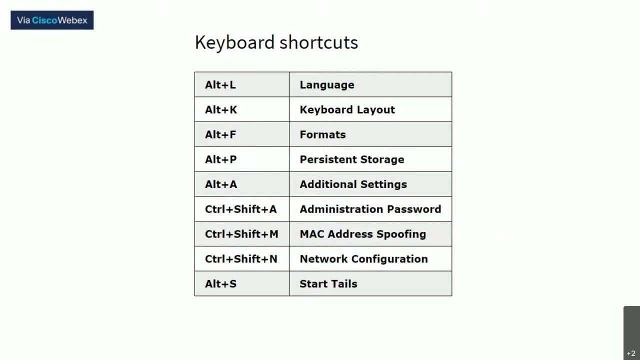 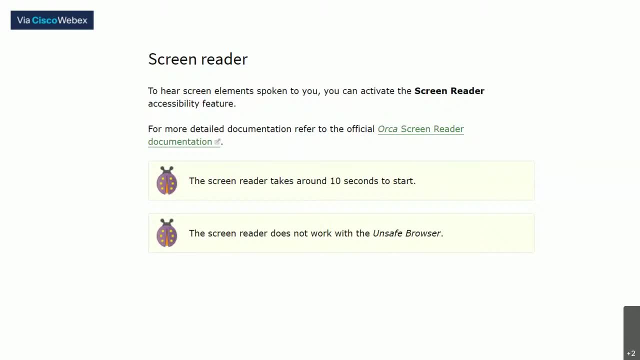 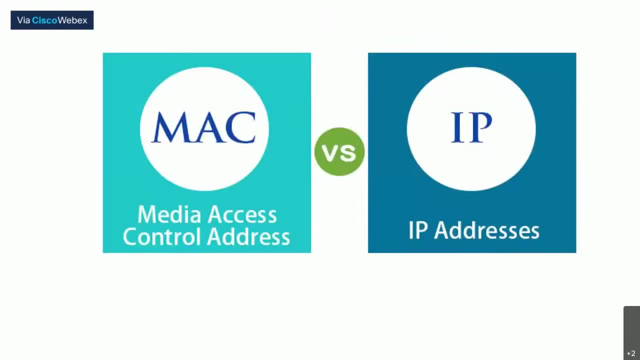 So if it doesn't have the password, you will not be able to break it. So your data is safe. The screen reader is there for you to read the data from the screen screen. The keyboard is there and uh, this is 1 feature. Okay, You know that there are 2 types of uh addresses in your system, What is called IP address. Another 1 is called as Mac. 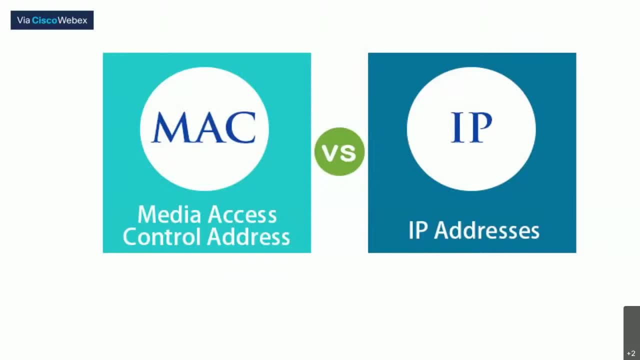 Can anybody tell me what are the 2 types of IP address? Which are the 2 types of IP address? anyone? Yes, and IP v 6 IV before is 32, big is 128. okay, So IP v 4 and IP v 6 is then number 1, and number 2 is these IP addresses, whatever you have when you are connected to the Internet: IP. 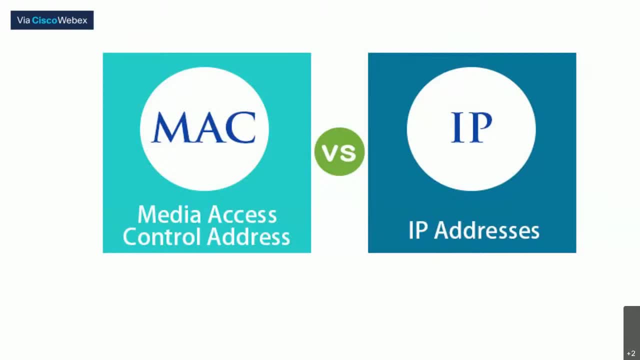 But if you are on a local network, then it does not use IP addresses. Basically It uses Mac. So Mac stands for media access control. Some people tell me you know some uh, uh, uh, uh uh. 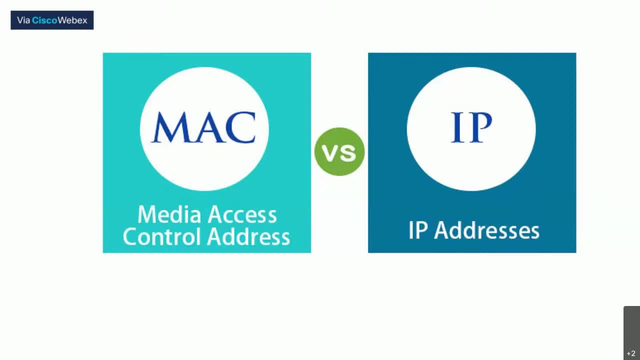 people where what they tell is: sir, my laptop is lost and i don't know what to do. i have the mac address. can you track the laptop and give it to me? is it possible to track a laptop using mac address? anyone? yes or no, quick, no, no, no, no, no, yes, yes, no, okay, so no, you're not able to. you're. 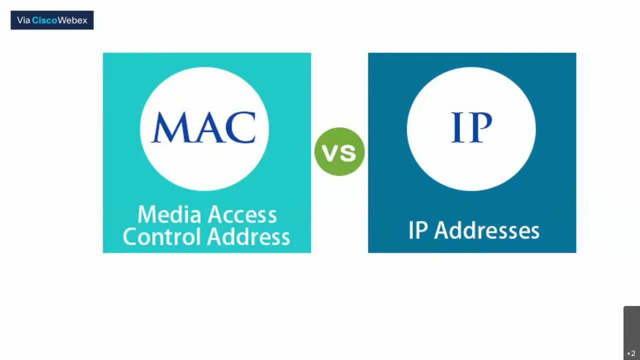 not able to uh track a laptop using mac address because mac address, the media access control, does not go beyond the local area network, exactly. mac is not sent over the network, so outside the network it will not go, so it is only within the network. outside the network what goes is: 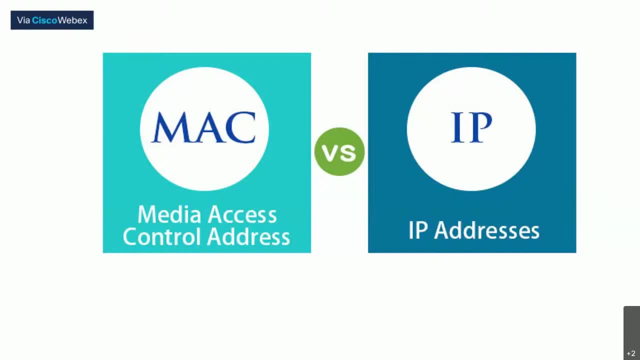 only the ip address so you're not able to track, but but the system admin. if the system admin has got access to the router, he will get your mac address because he knows the router, knows the wi-fi router, knows which are the laptop it has got connected to. okay number. 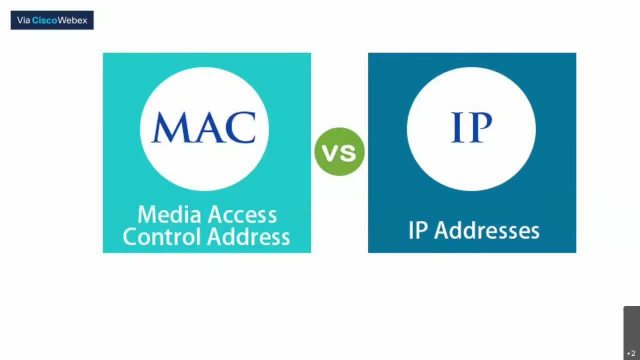 one. let us assume that there is a system admin who has got, uh, some 20, 30 routers, okay, different or 100 routers. he will get to know on which are the different routers that you have connected. so if he gets to know which router you are connected to what he will get to know what mac address he'll. 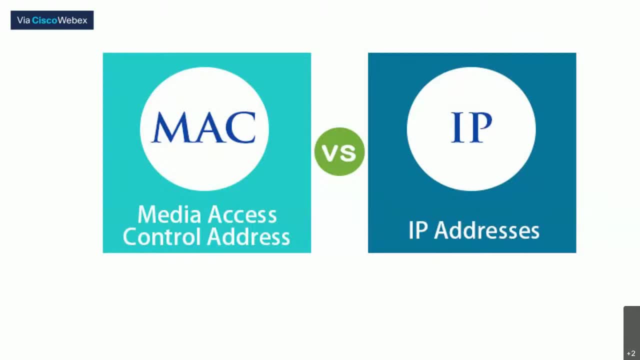 get to know what is the second thing he'll get to know. erp is all uh, ip to mac, mac to ip, not that, what, what is it? uh? erp, reverse erp? oh, exactly, shut up told, shut up told. he will get to know the location. 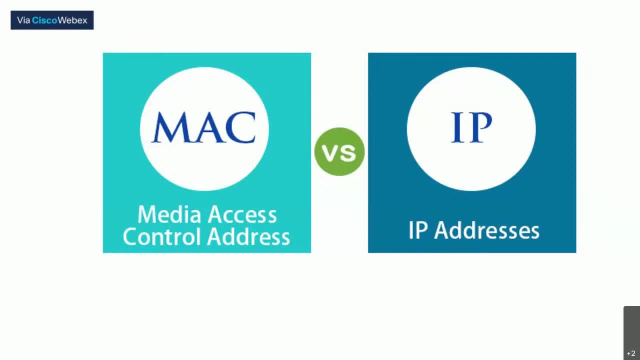 because he knows which wi-fi you are connected means he knows where you are. so your location, your geo location, they will get to know. therefore, if you don't want to uh, make the router, get to know your mac address, if you don't want the person to know where your geo location is. 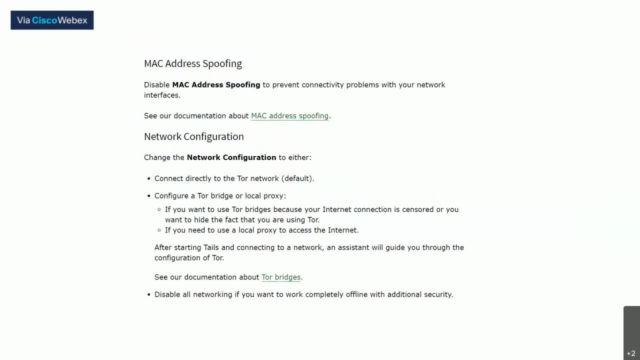 there is a feature called mac addresses spoofing. exactly max in a lot of uh, exactly, there is a mac address spoofing. so in mac address spoofing what happens is you can make sure that every time you are connected to the wi-fi network, a new mac address. 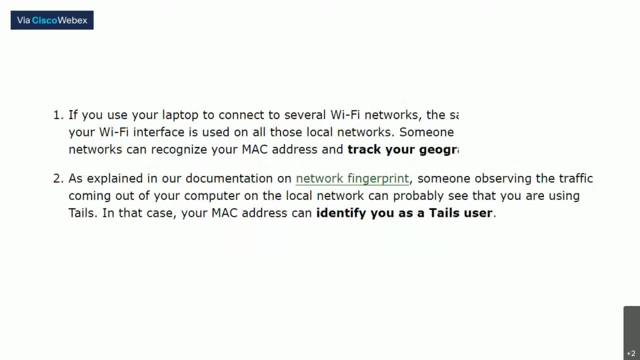 is shown. so the wi-fi router will not get to know your real mac address. mac address is a 48-bit address. uh, it is illegal to change mac address? yes, it is, i know that, but then i'm talking about surveillance here. so basically, what is happening is you should not change your mac address, you should. 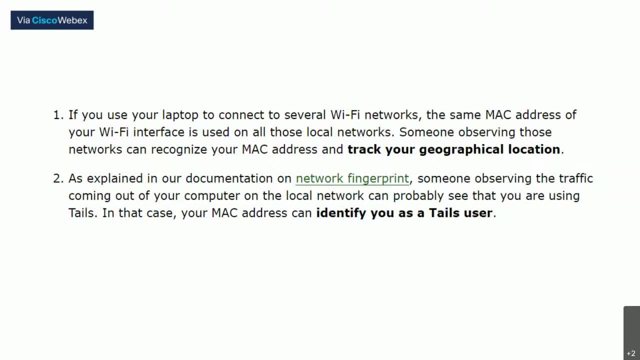 not be. if you are using it on your private network, then what will happen is you are not changing the mac address of your physical system, but you are changing the mac address of through the software to stay protected. all right, so your network fingerprint cannot be, uh, very easily. 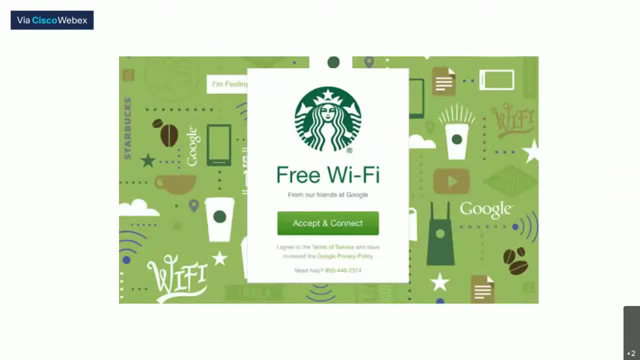 accessible. and uh, one more thing. what is this? what is this screen called? as anyone, if anybody tells the right answer, i will give this uh uh drive with the free installed uh tails to that person. no, no, starbucks is correct, but what is that screen called? i want the exact name of the screen where, whenever you're connecting, 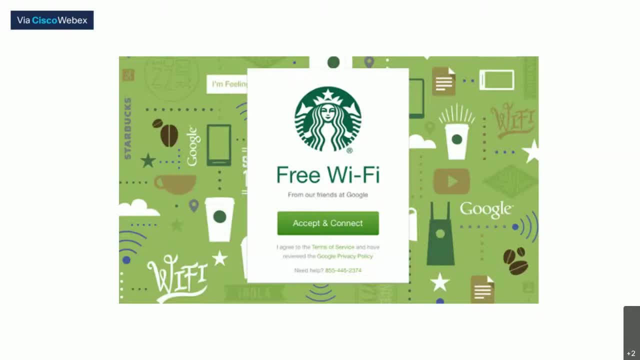 to a computer- free wi-fi. you will get one screen to enter the username, password or agreement. railway station free? yeah, but what is that? what is the name of that? anyone can, anybody. what is the name of that? what is the question? captive たう. この鑼都是你的. 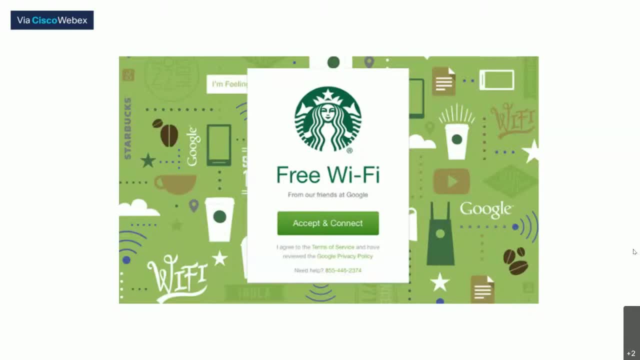 I hope you have pronounced your name properly. It's called a captive portal, Super captive portal. Okay, Alan has also told it right, But only 1 price was there. So, anyways, captive portal is the name for this. So in captive portal, basically, what happens is uh. 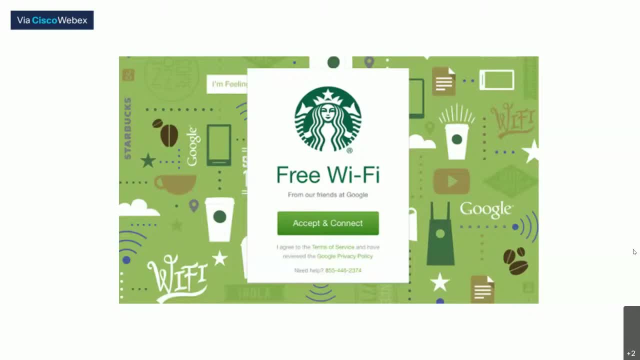 You get that 1st screen. 1st screen you get, and in the 1st screen you enter the username and password. You feel that is Internet. That is not Internet, My dear friends. It is an intranet based web page. 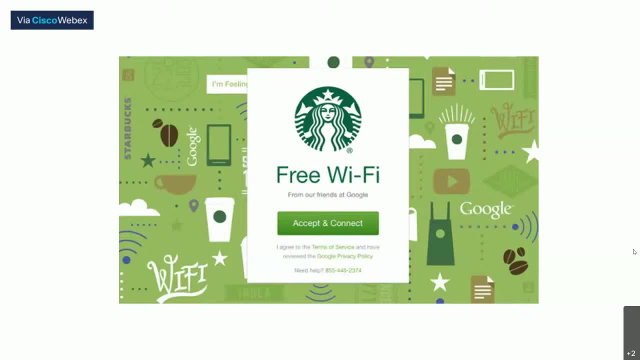 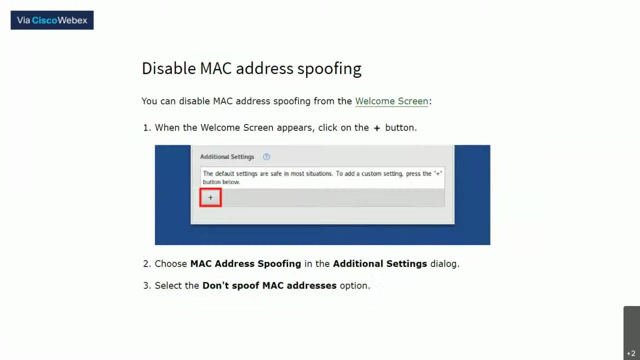 And on that web page, if you're accessing the person who has got control of that captive portal, he will get to know your. Okay, so this is how it works. Uh, anyways, anyways, uh, let me go on. So so you can also disable Mac address spoofing. That option is also there If you are. if you feel that, no, I should not use Mac address spoofing because, anyway, you're using IP address spoofing to Mac address spoofing, You can disable it. 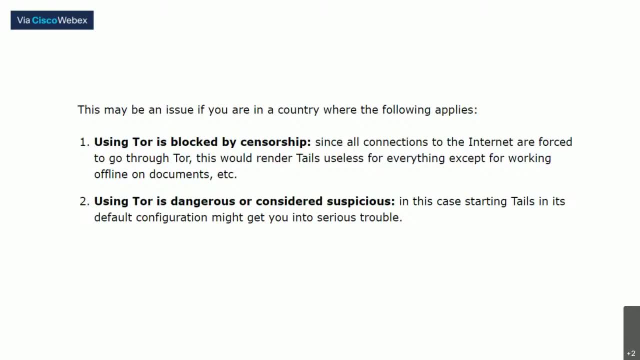 And uh is blocked by. Sometimes what will happen is some countries like China So, and some other countries also. they have blocked to talk, They have blocked up. So uh because of the censorship and uh using can be dangerous and suspicious at times. 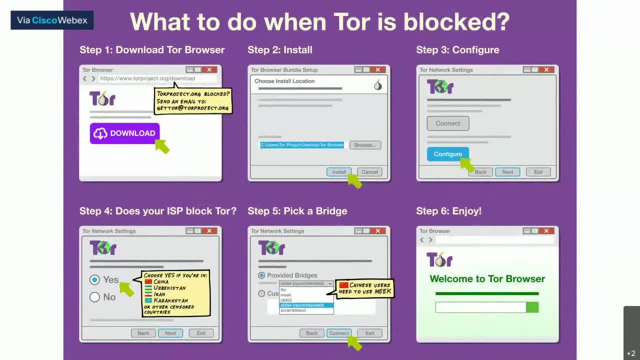 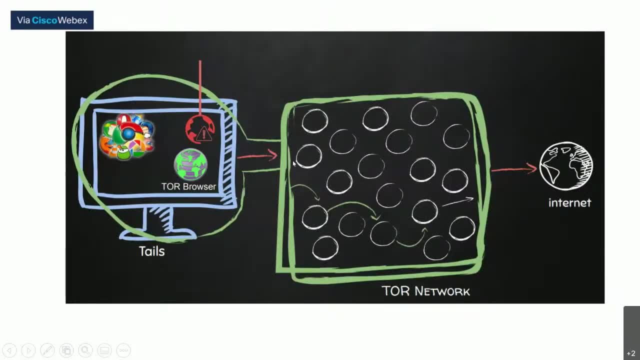 So in that case, there is an option, my dear friends, after you download, after you download, You need to pick a bridge, I repeat, see, directly connecting to the top network. You, you may get, uh, uh, that person may get to know that. 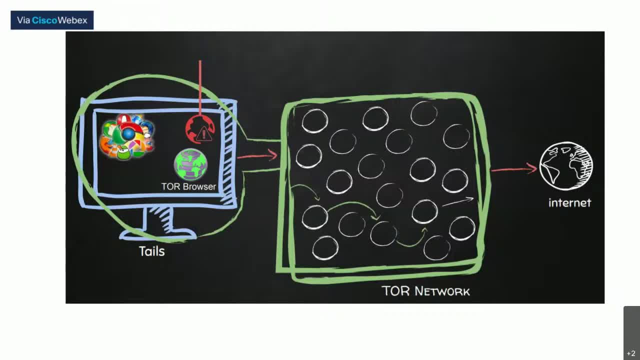 Please understand. there are certain countries which are blocked off. So if you're going to start, they'll get to know that you're connected to the top. So if you want to evade that, you can do an option where in you use something called as a bridge. 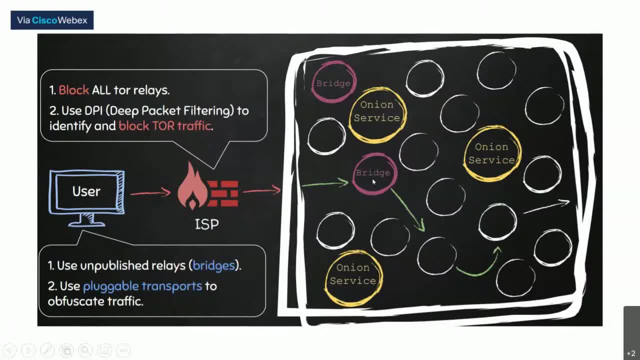 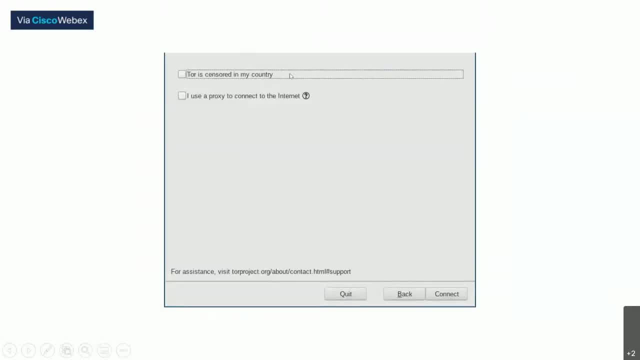 You can see the bridge here. the bridge, So you connect to a top bridge. when you connect to the top browser, when you connect to the top, there's an option that is censored in my country. Click on that, Then there is a. 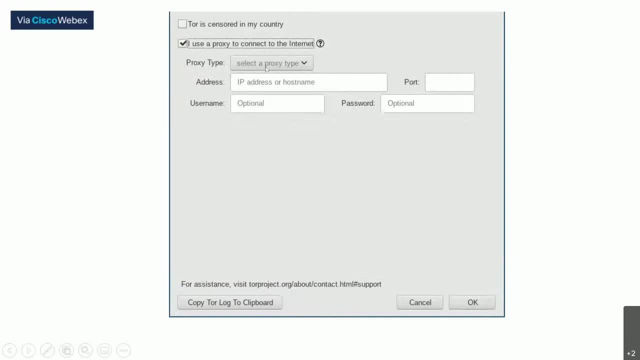 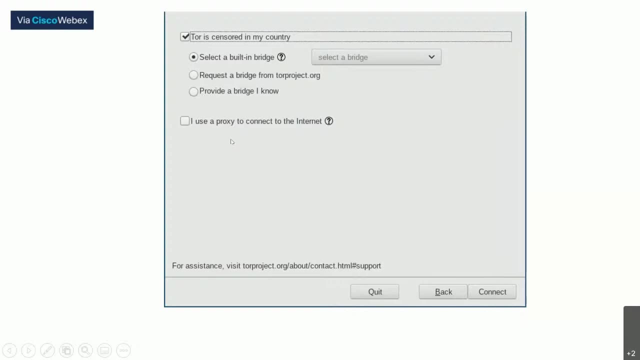 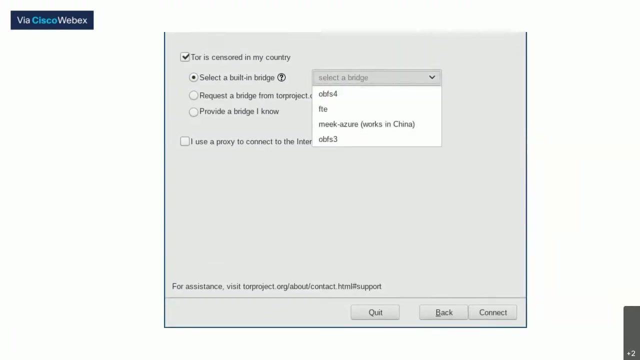 Uh, uh, uh, uh, uh. click on that. you can create one bridge. you can create one bridge. so tor is censored in my country. when you do provide a bridge, either you can use your own bridge or a bridge that you trust, or a bridge, random bridge. so once you create the bridge, what will happen is: see, there are bridges. 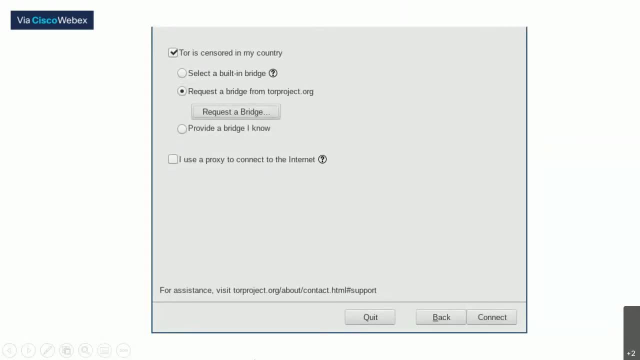 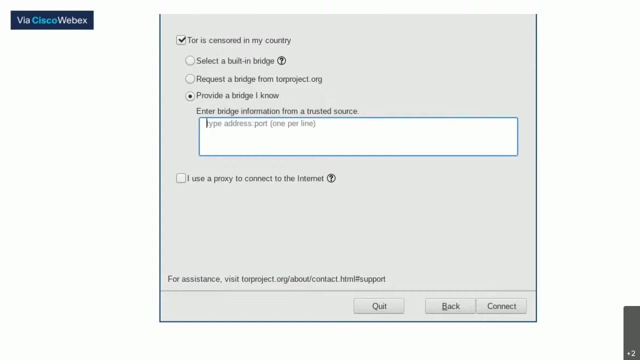 that work in china also. okay. so what will happen is, when you create a bridge, you are going to be connected to the tor network through a bridge, so that the person who is going to monitor you will not get to know that you are using tor. so this is how it is working. so, my dear friends, 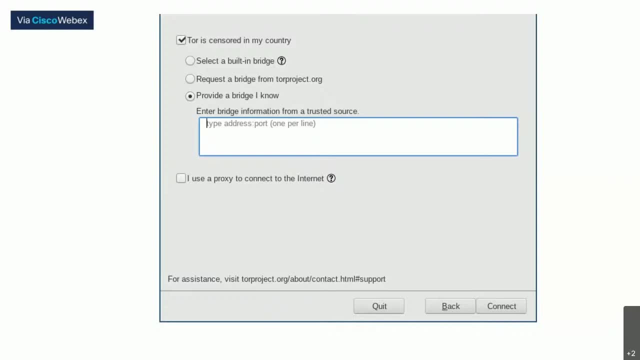 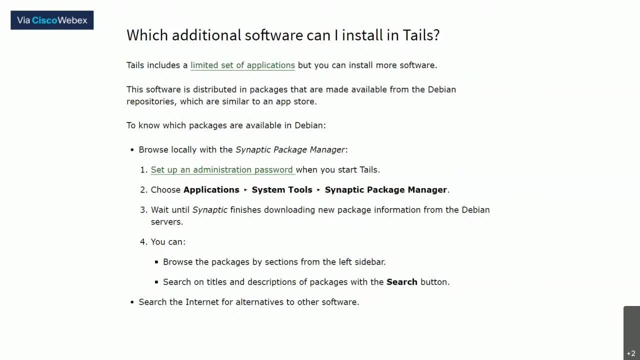 if you are going to connect to the tor network and you don't want the isp to get to know that you are connecting to the tor network, what you need to do is what you need to connect to the bridge. so this is one thing, and if you want to download some applications, please use the. 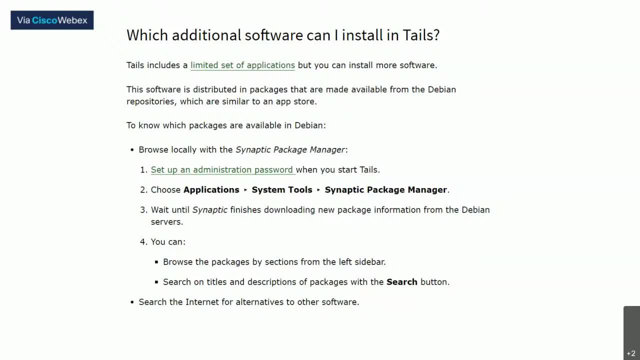 synaptic package manager. so, whatever applications and the repositories of dbn are there, you can install it. please don't install other apps because it can be dangerous, as and they will get to know that you are using, and you can also, as usual, connect to the wi-fi. 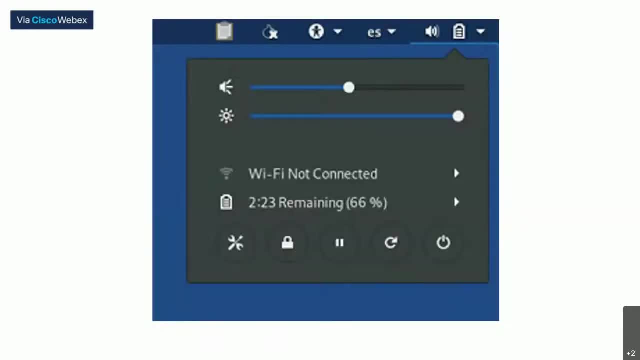 network and by using wi-fi network, my dear friends, which is the best wi-fi network to be used? encryption, wep, wpa- which one? anyone, which is the best one? wpa3, wpa2, wpa1, wep- which one? okay, now the answer. the answer is yes or no. 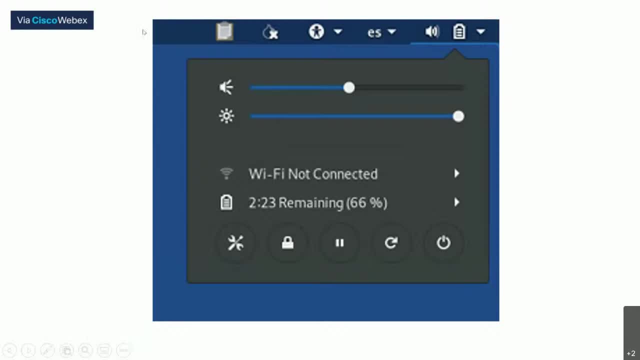 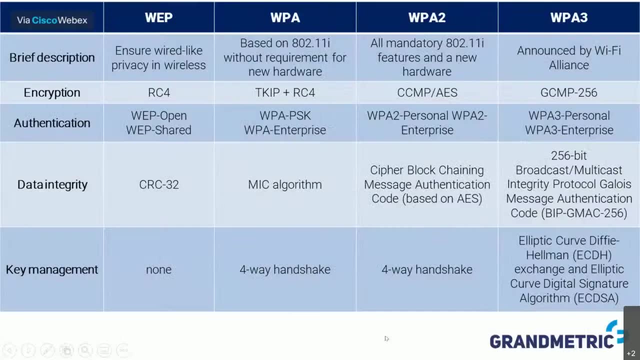 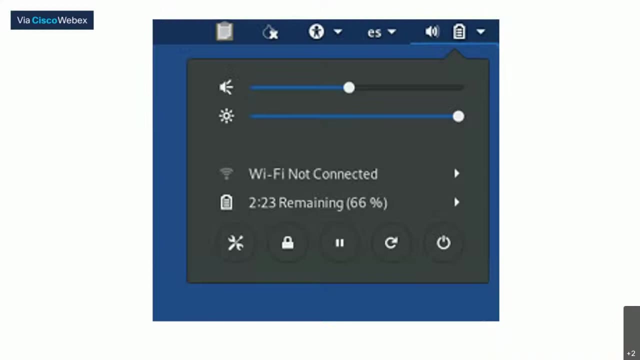 the answer is wpa3. okay, so please use wpa3 and you will be connected to the wi-fi, because wpa3 uses elliptic curve, defy hellman exchange, so it's a fantastic way of doing it. take care, and while switching off tor also, simply don't pull the pendrive. okay, because? 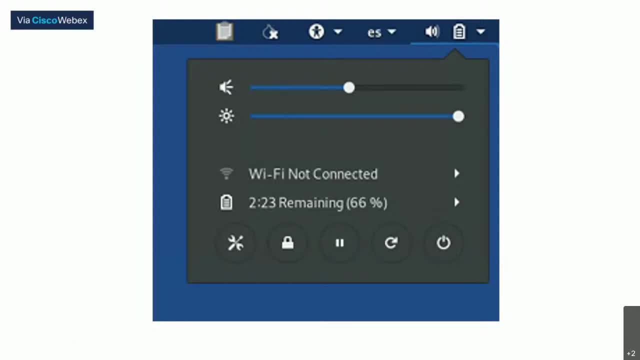 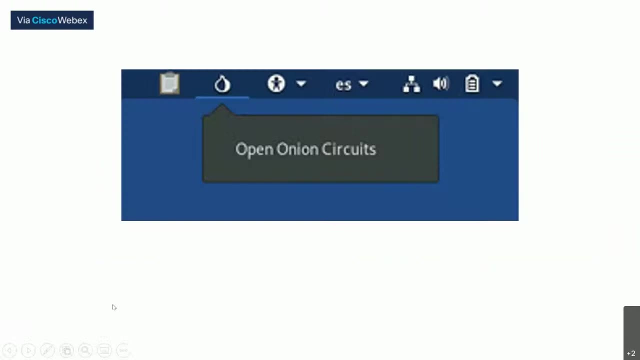 some data may be transferred and your pendrive may get conked off. so there is an option in the tor on the top, you can see at the top, there is an option which is called as switch off, so power off button. click on that and you will, uh, get logged off, okay, and then you can remove it and also, every time, use. 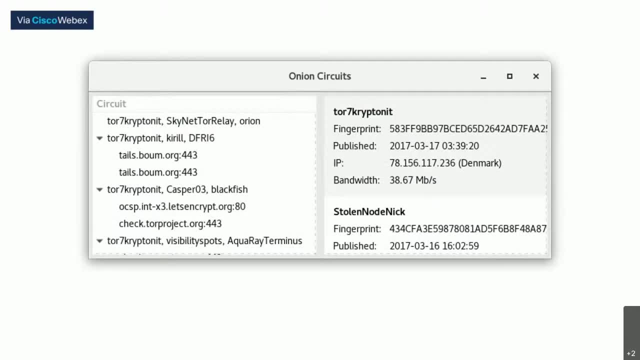 new circuits. so every time you can, circuit means i told you how the data has to go. if you're using the same circuit that the end of the last relay, he will get to know your data. so if you don't want him to get to know everything, keep changing the circuits. okay, because the exit node usually 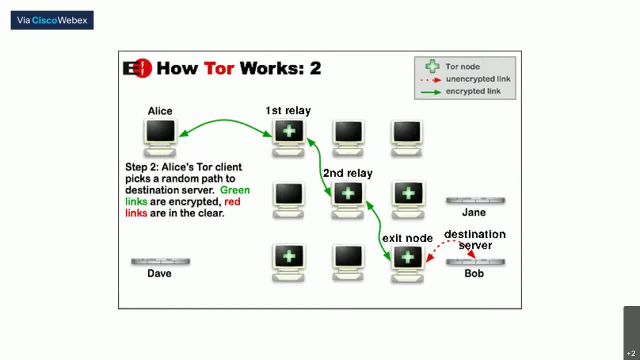 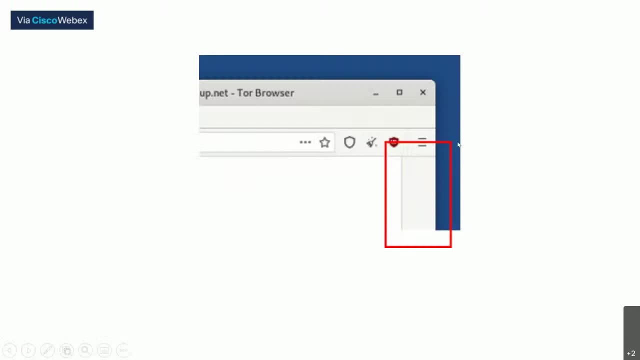 if it is a non-https server, he can sniff your data, but though you will not get to know from where it has come, but still you can use certain tricks later on. so to be on the safer side. and tor browser has no script, so most of the java scripts and anything will not work on top browser. 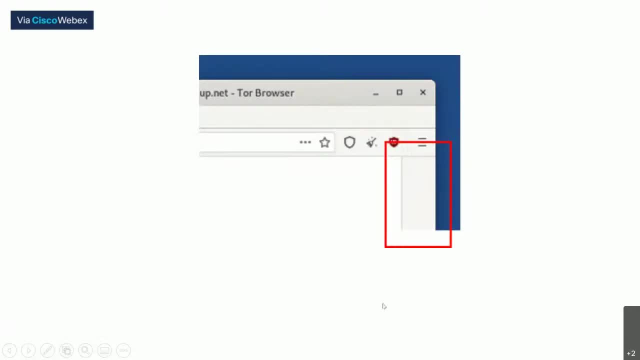 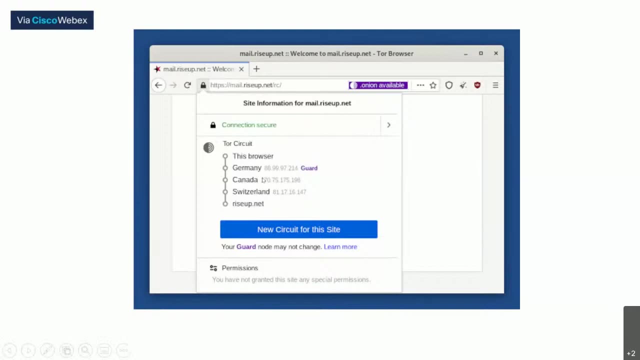 and also it will do on padding, so that your browser will your websites will not get to know which browser you are using, which operating system you are using, and all and the newer subjects make you, uh, show as if you are from germany, canada, switzerland and many, many other. 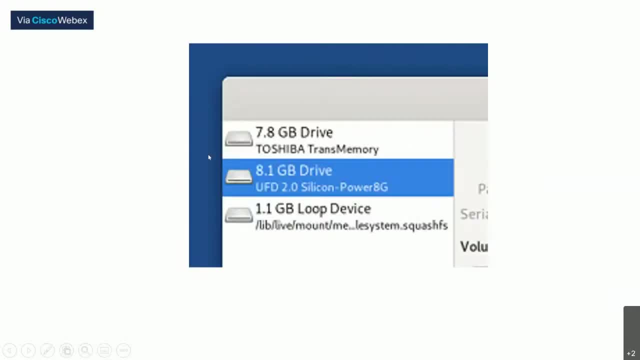 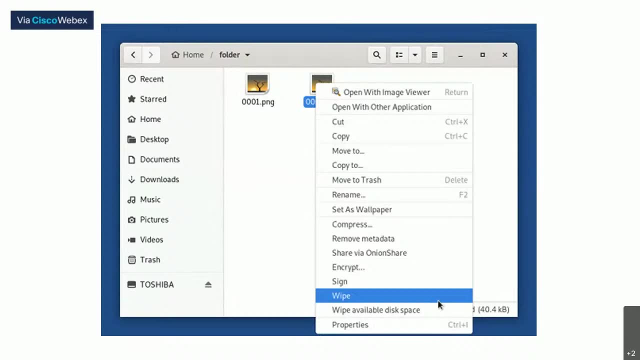 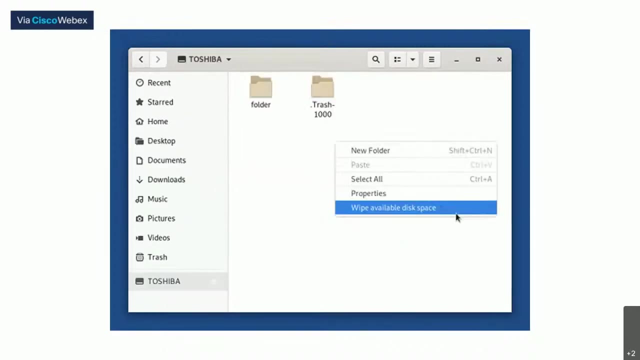 places and, as i told you, persistent storage you need to use to save the data. and if you are going to reuse that pen drive some other time, there is an option called wipe. so wipe all the data and everything is gone. so wipe the disk space and then you can use the pendrive and then there is 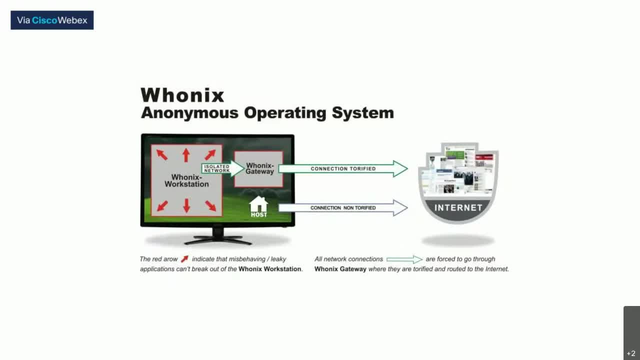 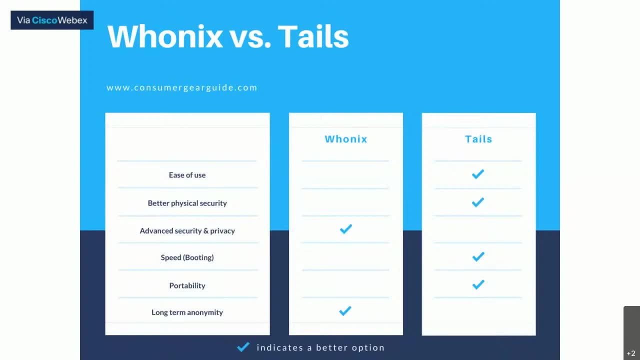 one more operating system called hoonix. so hoonix is also similar to tails. uh, they have got their own advantages and disadvantages and all that. and, uh, my uh, next session- probably next session, if you guys are interested- it will be on hoonix. so anybody wants me to take a session on hoonix? yes, you want. see, i'm so glad, i'm so glad that. 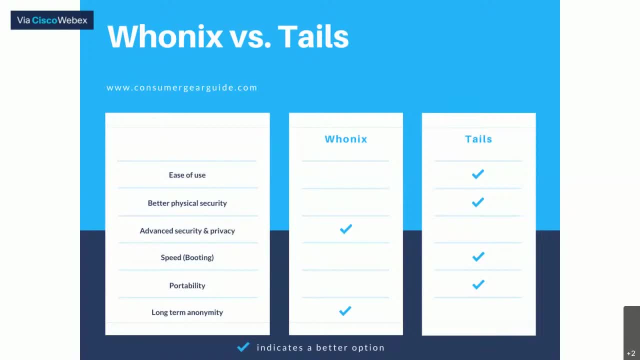 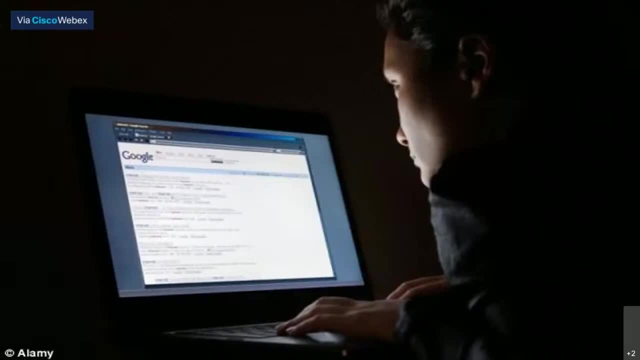 you're interested. so probably very soon we'll have a session on uh, hoonix and uh, my sincere advice to all of you is uh, don't uh check the computer when uh it is dark, it is your eyes. use a lens which has got blu-ray protection and uh, for every 20 minutes of 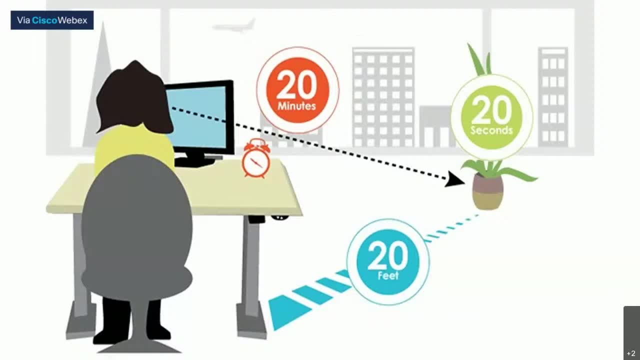 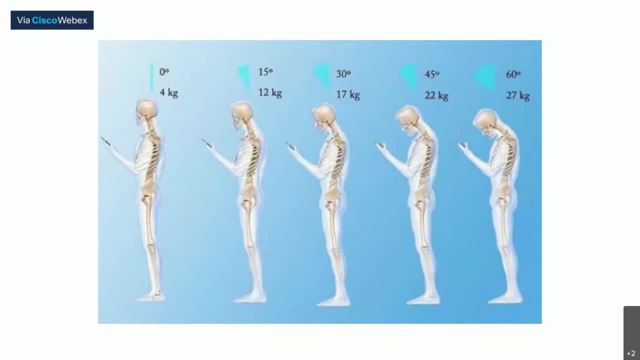 screen time for 20 seconds. see 20 feet away so that you can keep your eyes safe and when you're using your phone. also, don't bend your head too much, because head is 4 kilo and then 15 degree bend, it becomes 12 kilo strain, 30 degree bend, 17 kilo strain and, uh, 60 degree bend, it is 27 kilo. 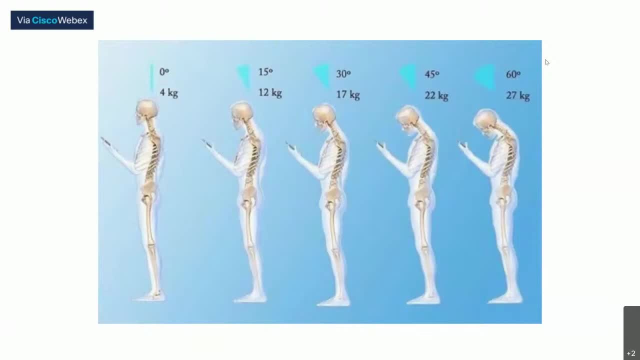 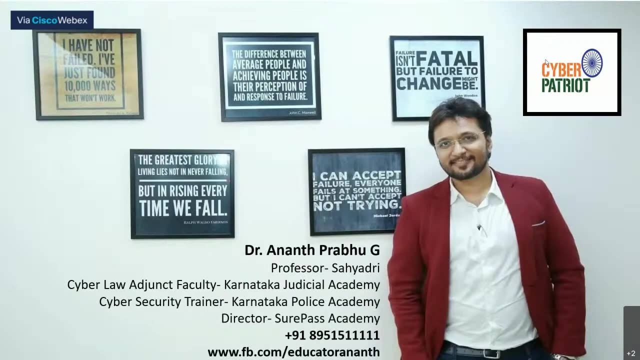 that is why many of you have got head pain, neck pain and all that. so please take care of your head. if you have any questions, most welcome to shoot. and this is me. this is my um mobile number. i'm not available over phone, only whatsapp telegram signal and uh, i hope you enjoyed the session. 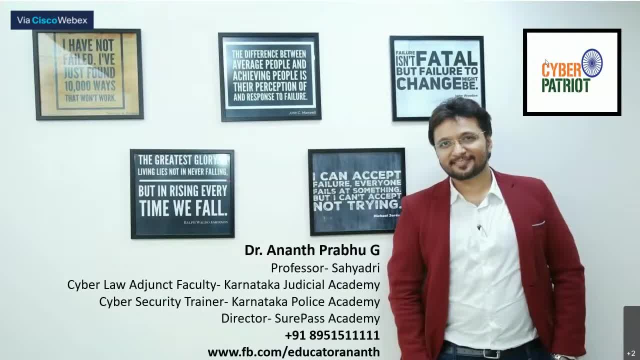 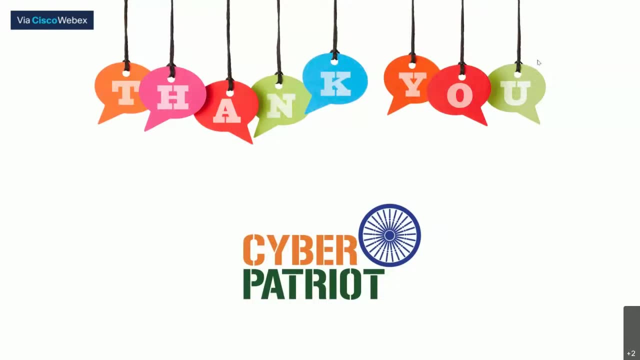 and uh, if there is any improvements that i need to do, please feel free to share the feedback. it was a 1 hour 15 minute session and, as promised, right on time, so thank you very much for the time. so the question is: why didn't we talk about kali? no, because today was only about tails, as you have. 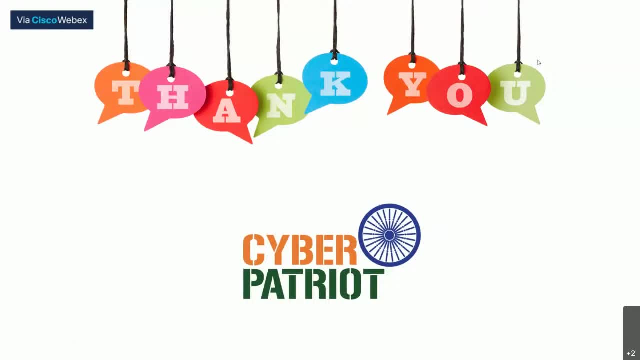 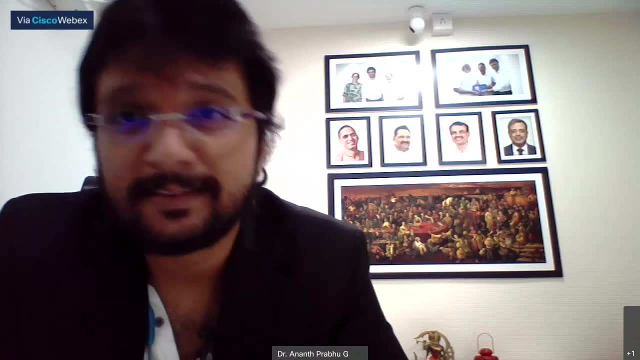 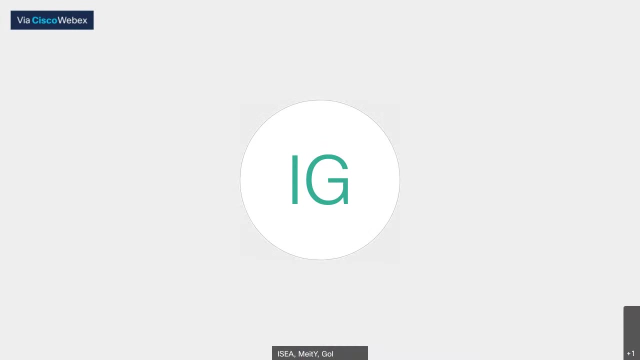 rightly said. probably we'll have one workshop after who nicks on kali linux, also when i'll be talking about some tools which can be used for ethical hacking. okay, 706 participants- super, very glad this went beyond 736. and youtube: more than 123 people are there. 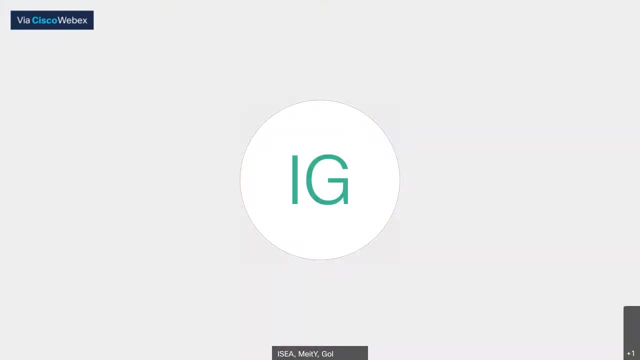 it is, overall, extremely, extremely super obsession, sir, And I think all the people have liked it. uh, you know, uh, the kind of feedback which is, which is that throwing here and there, and I think there are some few questions. Can we take this question, sir, Please, please, please. 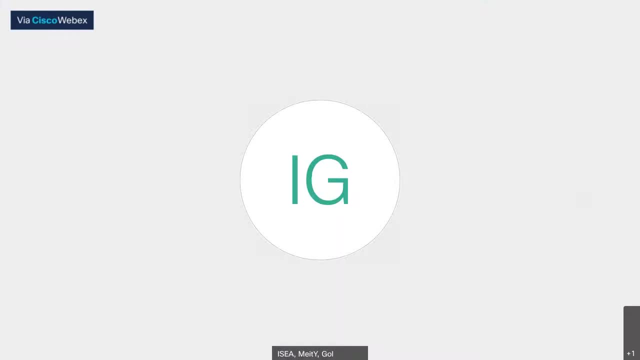 Okay, uh, these questions are collated from both uh as well as YouTube also. Uh, why spam messages came in mail? Okay, messages usually come because, uh, whenever you're using uh any email address, for that matter. 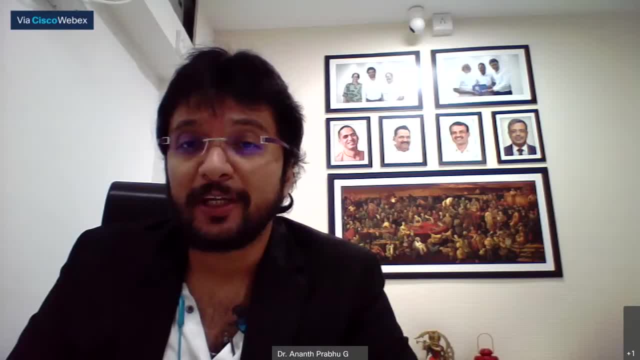 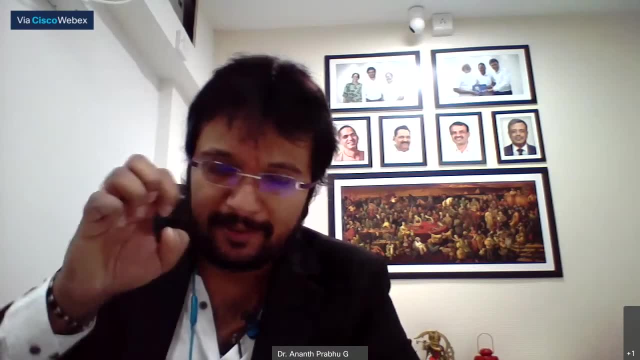 Sometimes, what your friends will do is, when they're sending an email, uh, instead of putting in, they put in CC, so they're they're going to uh. many of these people are going to collect these uh emails and there are many service providers who will be buying these emails from you. 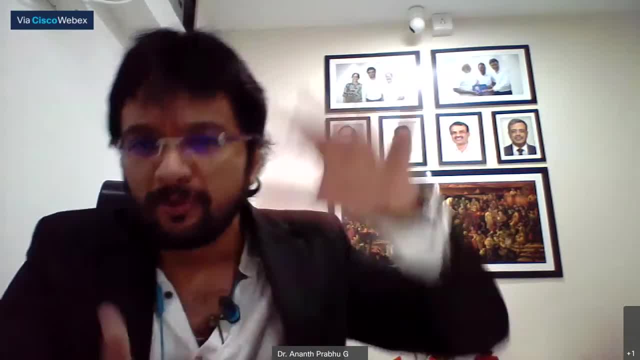 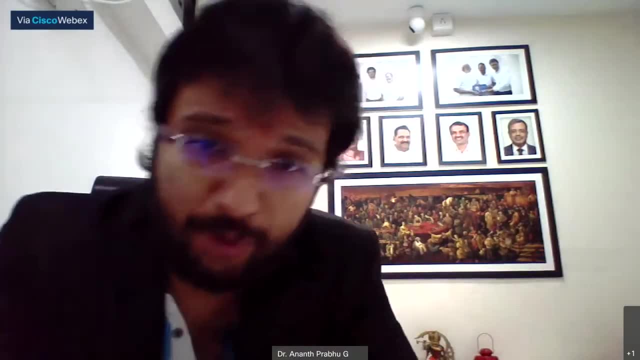 They're paying 1 rupee, 2 rupees per email. So you can give new emails which are valid, which are functional. If you give it to them, you can earn money. So people send the email addresses to others and these email people. what they do is they profile based on country, age, sex. 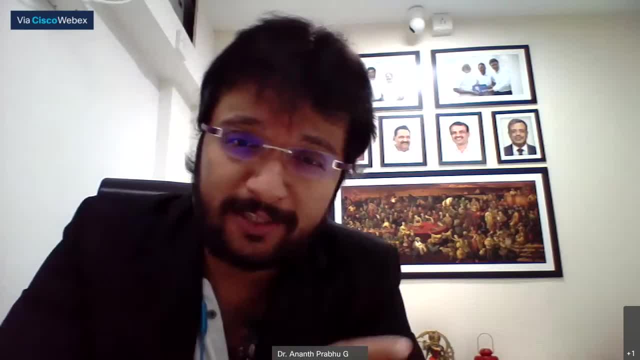 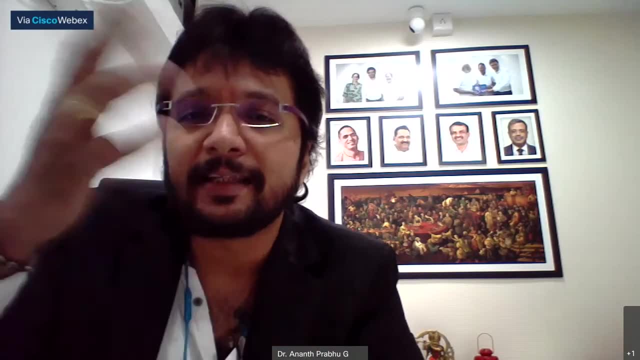 Uh network, whether you're a high network guy, low network, and they're going to sell the emails. and once the uh companies buy the emails then they'll be sending their uh advertisements and all that to to you. 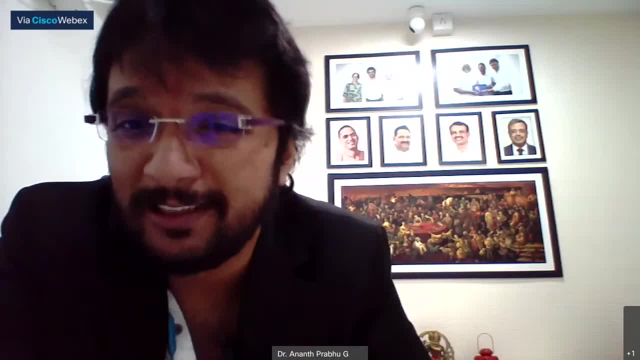 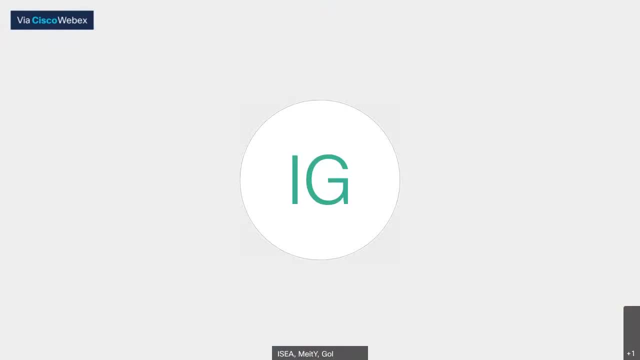 So this is how the spam is usually originated, because unsolicited mails keep coming without Do you actually subscribing to them. Okay, uh. so one question like: uh uh, track my phone, how to know that and how I know? uh, check, uh, uh, check or stop this problem. 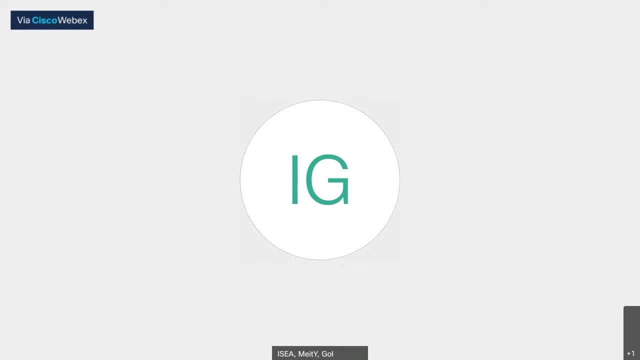 Like if someone is, uh, I think the question may be like: uh, uh, if, if he's, if he lost the phone, like, how do we track? Okay, so if you have lost your phone, if it is an iPhone, you can go to the cloud, and if it is the Android phone, 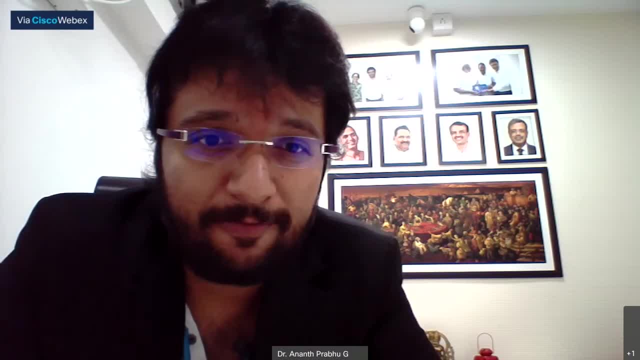 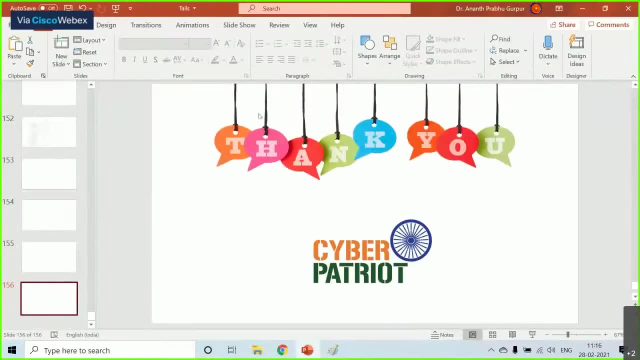 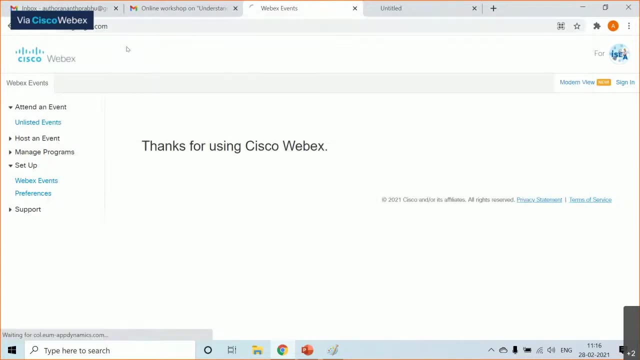 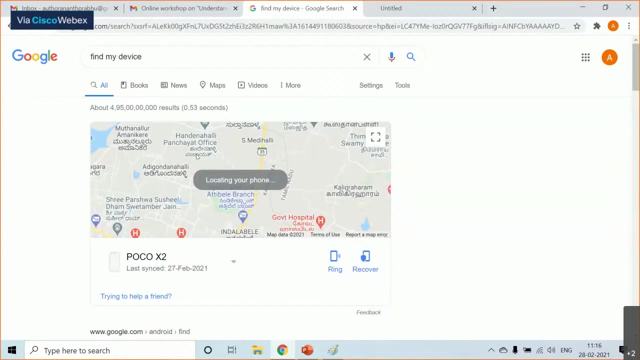 Uh, I'll, I'll just show, Show you a live demo. and find my phone. I'll show you a live demo. So my screen I'm going to share. Okay, so my screen, is my screen visible to all of you? Yeah, Yeah, So I I just go to, uh, Google, Google dot com, and I just type: find my device. Okay, So now look at this. So it's going to locate my device, So it tells where my devices. 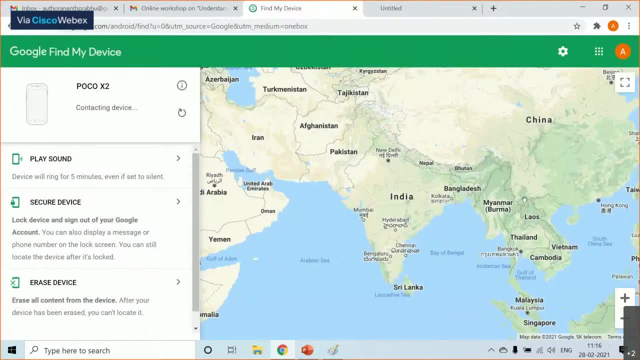 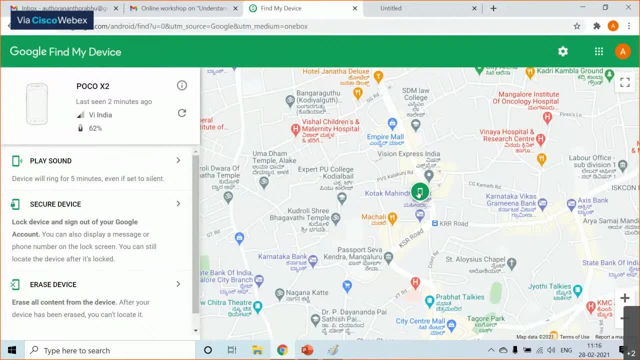 And I click on that. so right now my device is. It's contacting my device, Okay, Okay, Right now it is here, It's in case round or it is over here. Now I can do play a sound if I press on that. 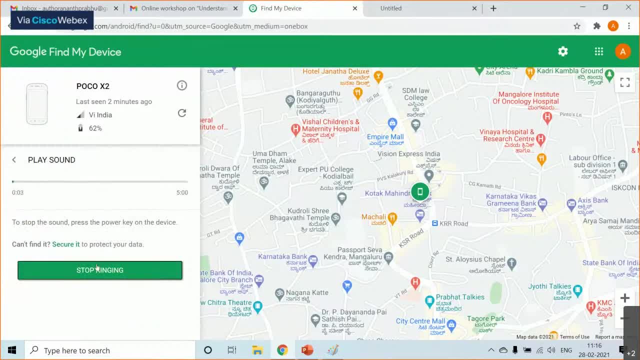 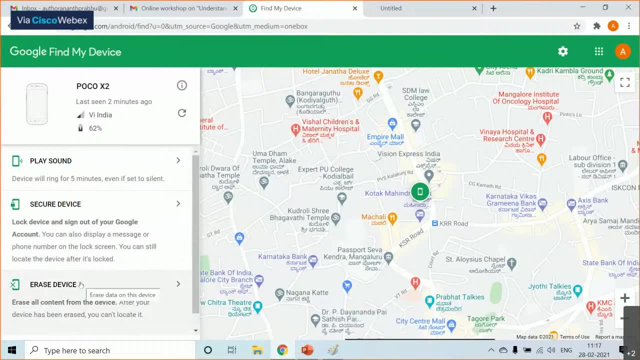 See my. my phone starts ringing. Okay, I can stop it. Uh, I can secure device because if I'm not law and I can erase device also. So if I feel that my device is gone, I don't want the guy to get my uh details- I can get his device. So this way, same you can do it to the cloud also. 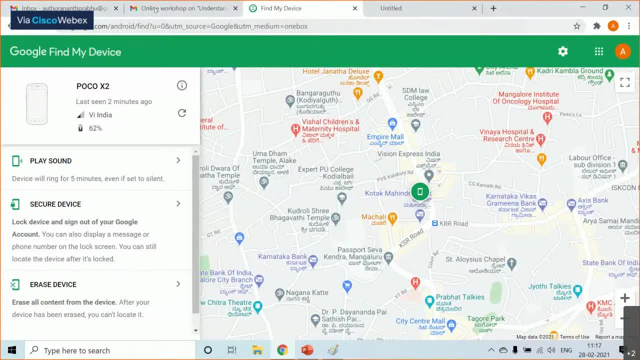 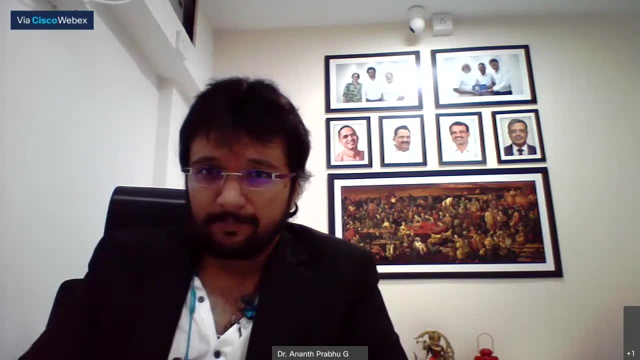 Uh and uh, yeah, um, you can also have some uh tracking software on your phone to Check if your phone is lost or not. All right, Okay, How can you trust one dot one, dot, one, dot one. 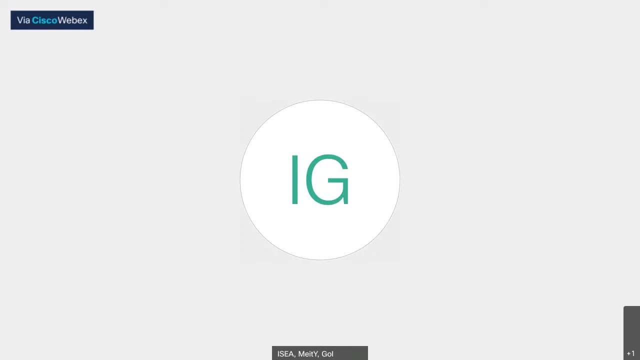 How can you trust on one dot one, one dot one. It's open source, so you can check the code, You can check, uh, how, how it works. It's uh transparent, Okay And uh, I think this question is from if someone is searching. 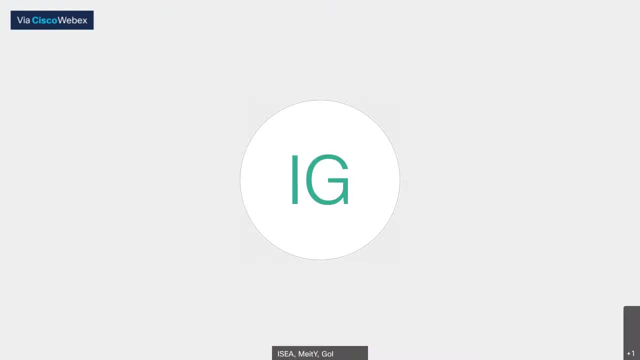 On a point of love. uh, other sites provide a lot of data on the same topic, Which immensely help the researcher on the topic, Is it not? it? I didn't get the question. sometimes open, such is beneficial, For example, if someone is searching on a point of law. 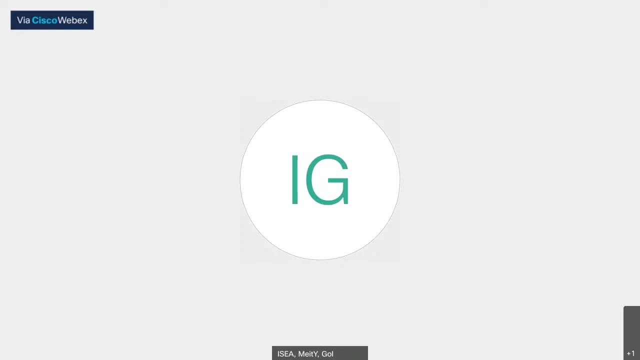 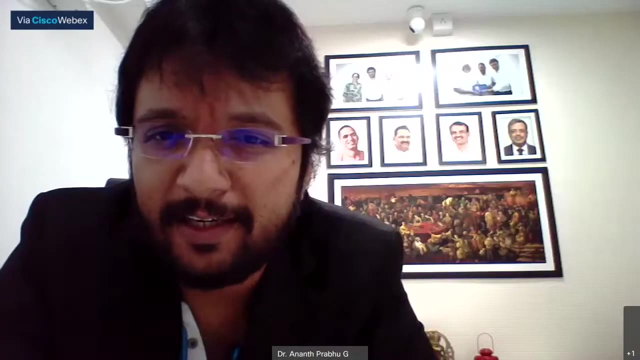 Other sites provide a lot of data on the same topic, which immensely help the research on the topic, Is it not? Yeah, it does help because last time, even through our, we had conducted a workshop on where intelligence, where we can gather a lot of information. 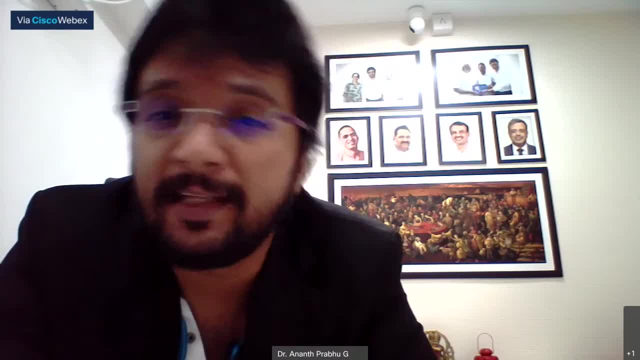 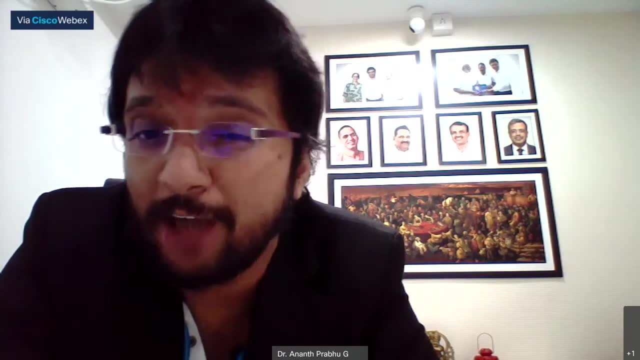 Now that information- if it is information with your consent that is available, that is no problem, Somebody will get it. But many times what happens is we undergo 1 concept which is called a dog scene. So basically is your private information getting public. 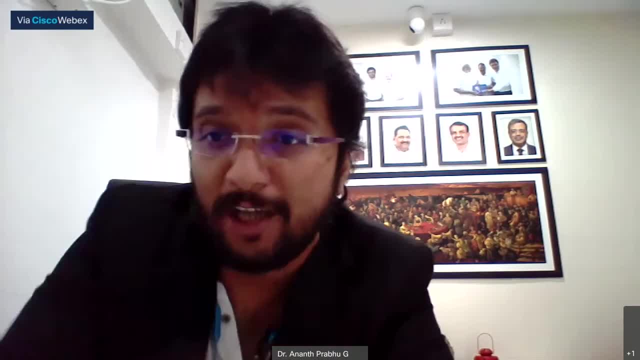 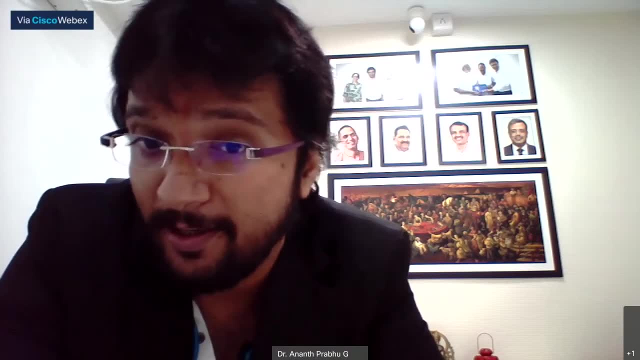 There's the problem comes. So in that case, you need to do a Google search about yourself, Because I always tell you search for so many things, but have you searched for yourself? search for yourself and then, if you find your information, private information there. please request the system admin. 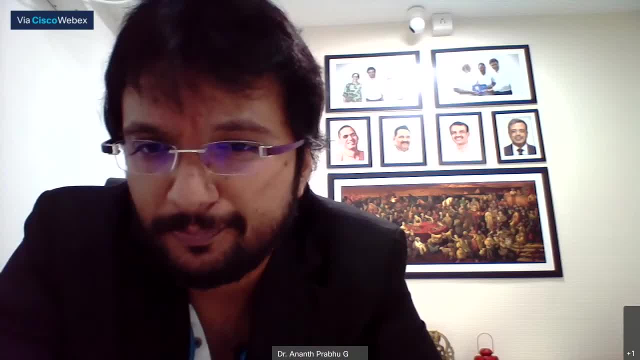 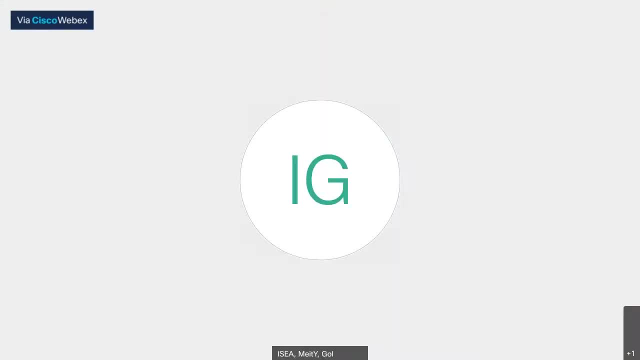 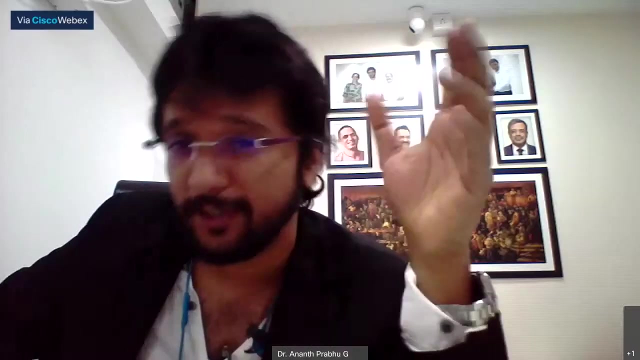 Of that particular website to take that information? Okay, so is what's up, say for telegrams, if It is using end to end encryption? Only safely can you save. Nothing is safe. Okay, last question: Are there any other questions? Anyways, the telegram group is there so we can ask him then. Yes, Yes, Yes, Yes, I think those are the questions. We can take it up in the telegram. 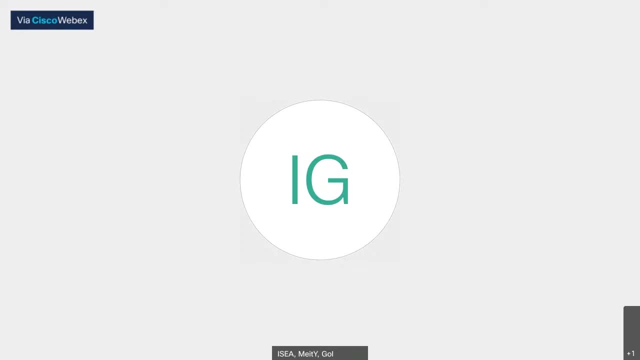 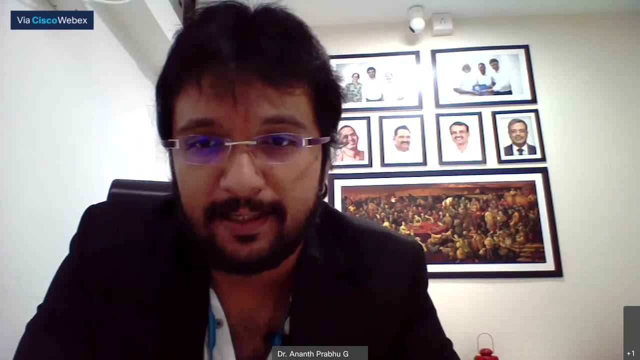 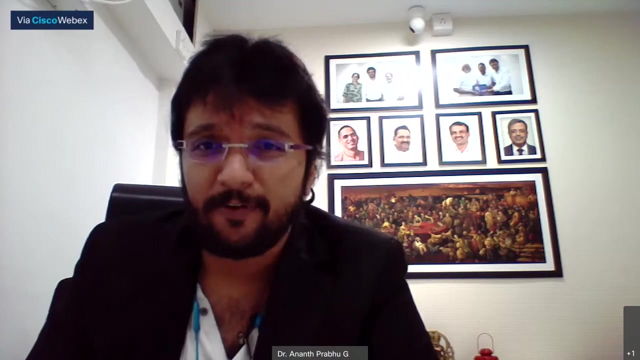 And we thank you for an excellent and wonderful session, and Thanks to all and I look forward to stay in touch with everybody, and my, my sincere request for all is: uh. this is my uh Facebook uh page, So I request you to please like my page so that you can stay in touch, and thanks to uh see me, madam Thanks. Thanks for making this. 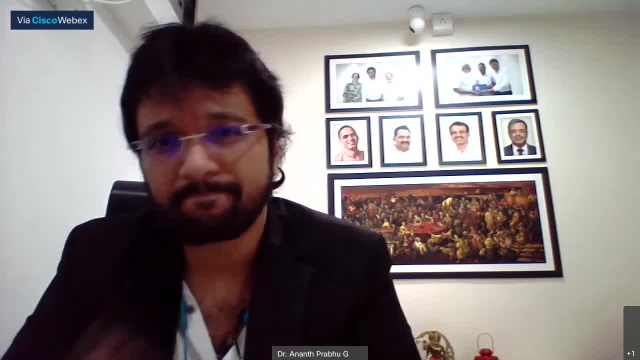 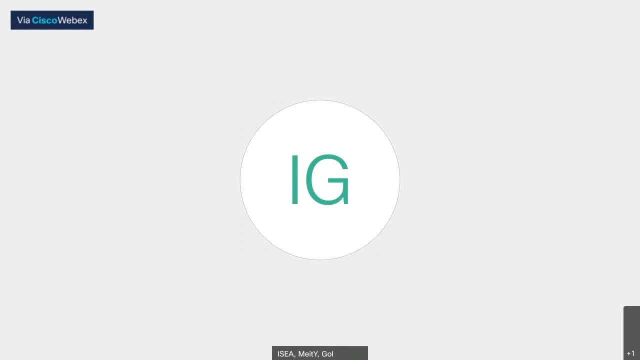 Seminar and it's a thank you. Thank you so much, sir, And we also thank all the participants uh joining and participating actively. That is more interesting. Oh yes, On a Sunday, on a Sunday, on a Sunday like uh, getting more than a 1000, uh near a 1000 people is not that easy. 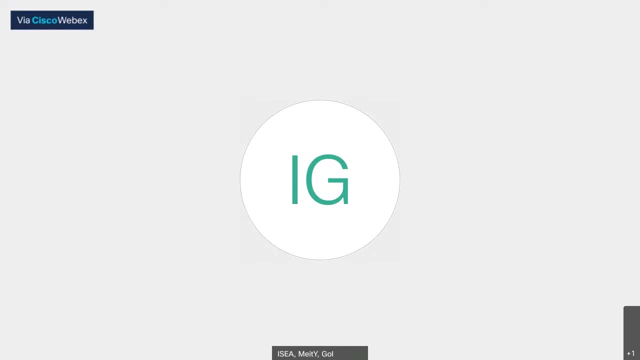 And we thank each 1 of you like uh joining the session from as well as YouTube, And I hope you all enjoyed this session. and many of them are asking, like how do we get this certificate? Yes, Like, we will be sending. uh, you know, we'll compile the data. uh, like who are? 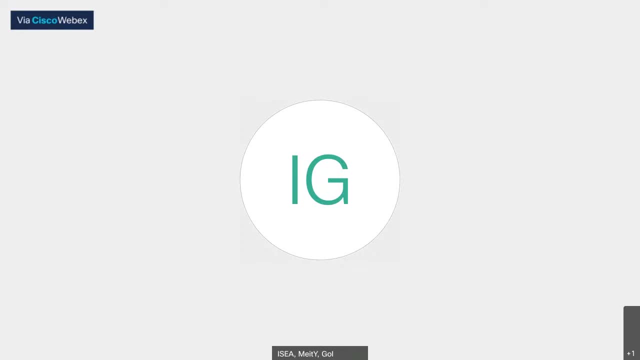 Join this session. like we will be sending the link- uh, you know, assessment link- to all the uh people via email. Yes, Via email will be sending and so that you can download your certificate by giving some kind of feedback as well as. 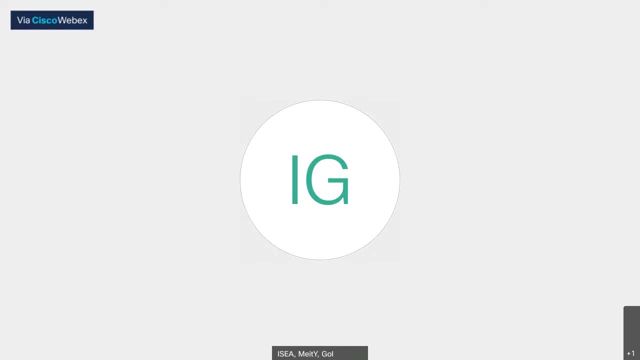 And what are the details you provided Like during the registration? like you might have been provided a email ID, mobile limbo, uh- the same thing. you have to use it while downloading the uh certificate. Otherwise, the if the if the data is not tallied, it won't allow you to download the certificate.